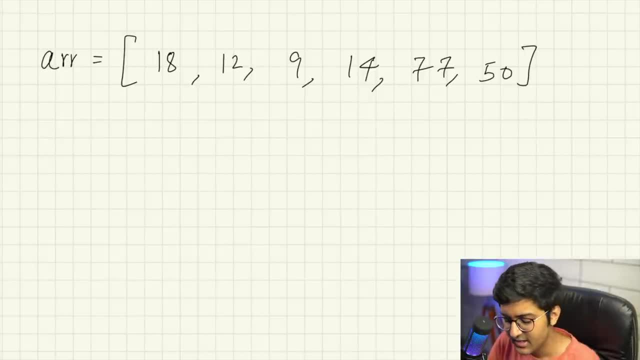 all these things. okay, it contains such numbers: linear search. so linear search is one of the techniques for searching some element in like a collection of data, like you can in this, because we have only studied about, like the string data type, the data structure, and we have also studied 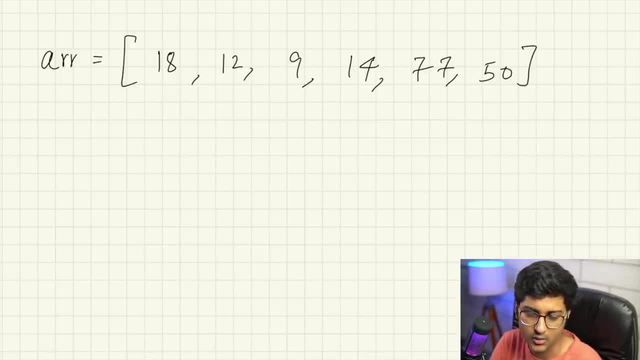 about arrays. so that is what we're going to be applying- searching towards- right now. but as we move forward, as we learn about more and more data structures, we'll see how we can search in those data structures as well. in this video, we will only talk about a few of those data structures. 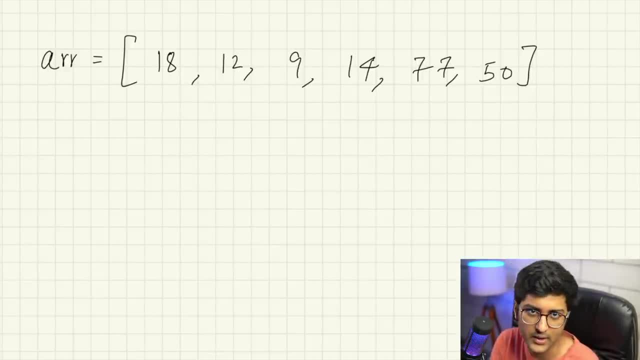 in this video we will only talk about some of the data structures that are available in the only be learning about linear search, and in the next video we will be learning about binary search, which is a very important topic. so this is a very basic searching algorithm- linear search, will you? 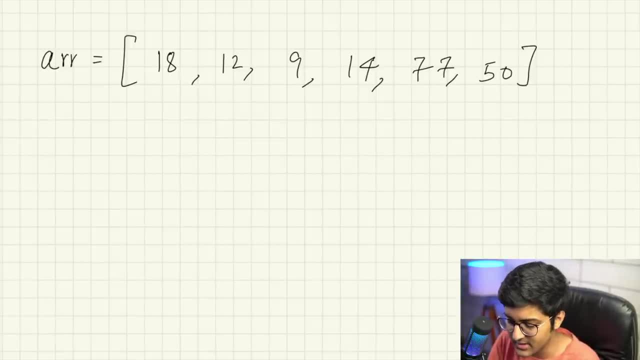 know, look into it how it goes, but let's say for now, our problem statement is that you are given an array of numbers, an array of integers like this, and the question is something like this. so question is: find whether 14 exists in the array or not. 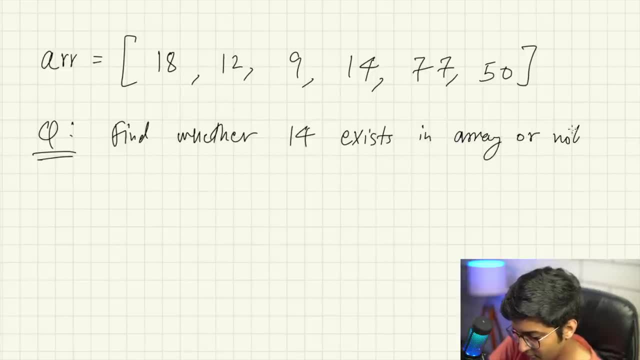 so there's a question: you have to find whether 14 exists, exists in the array or not. as you all know, we have already studied about it. you can access every index of the element, every element, every index of the array. you can access every element using what two things we already covered. 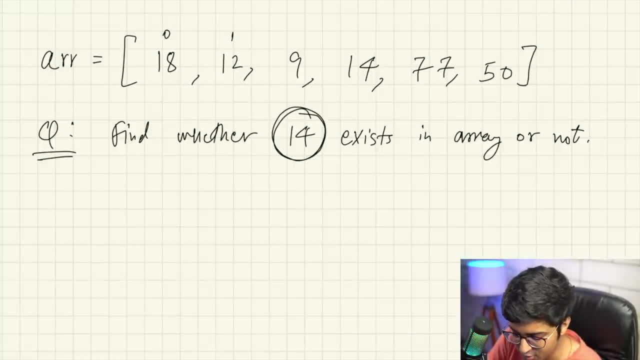 this in the array lecture. you can either access it via the index values. so if the size of the array is six, index is going to start from zero and five. so if i try to access arr of, one means the index at one, it's going to give me 12, for example, very basic stuff. other than that you can also use a. 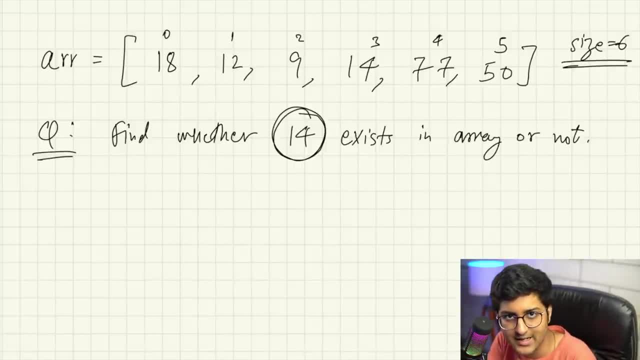 for each loop. okay, for each loop basically iterates over every element itself. we have also learned about that in the array section. links in the description. okay, so linear search is very simple. linear search says that start searching from the first element till you find the element that you're looking for. that is it. that's it, so it's. 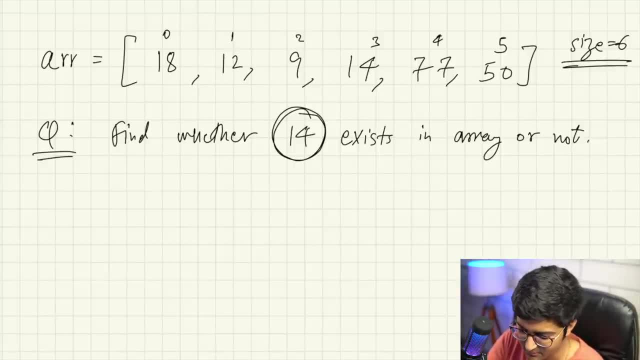 basically saying: start searching from here. so my pointer- let's say i pointer, let me change the color of this, let me change it to red, let's say so my i pointer is going to be here. it's going to say, hey, is 18 the one that you're looking for? it's going to be like: no, it's not okay. then it will move ahead. 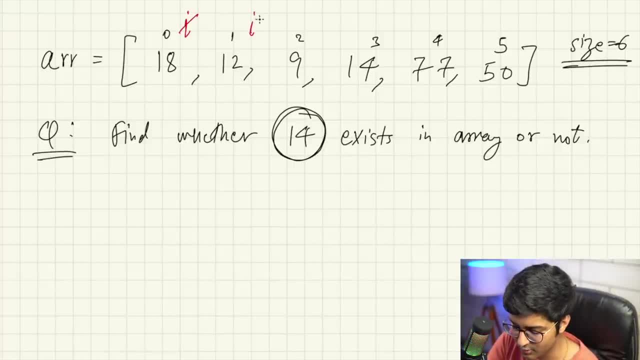 is 12 equal to 14, something that you're looking for. it's going to be like: no, it's not move ahead. is 9 equal to 14? no, it's not. is 14 equal to 14? yes, it is. it will then return the index value like 14 exists at the index number. 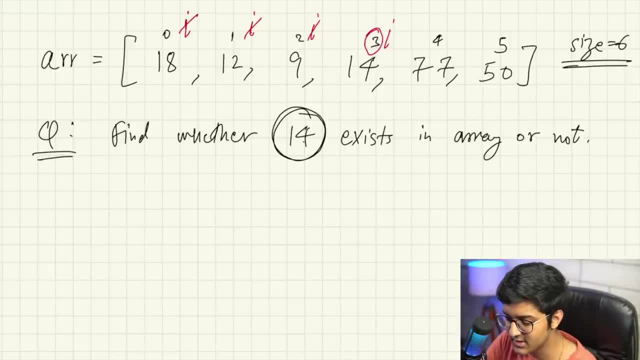 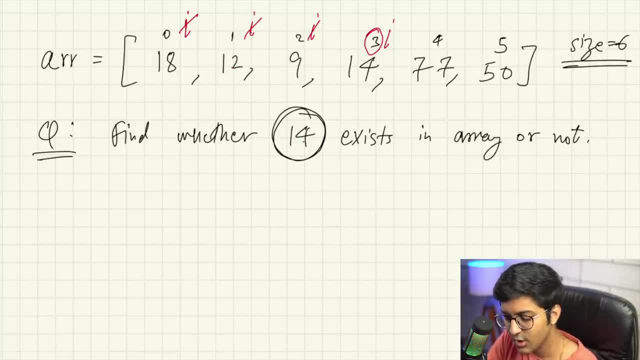 now you have reached the end of the index. so basically you're going to be like: no index is available that contains 88. in that case, like if no value found, return minus one, for example, because minus one index does not exist. so when you return minus one, it means that the value is not found, value does not exist. it's very simple as it is okay. 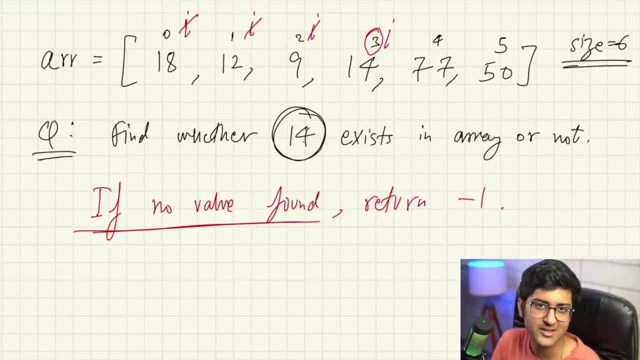 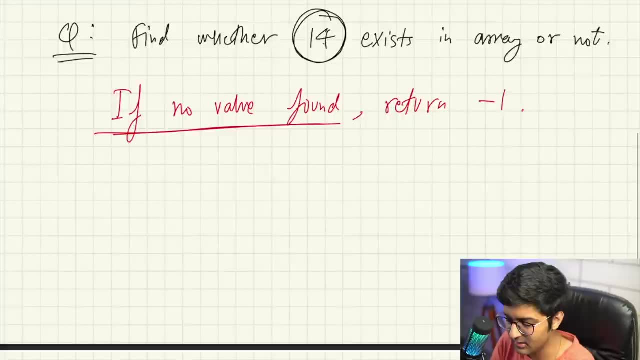 that is it, and we all know we are going to be using a for loop in this. so we just want to iterate upon everything and we are just going to check whether this is it or not. one thing for many people, those who are now- this is another important point, if you are already aware. 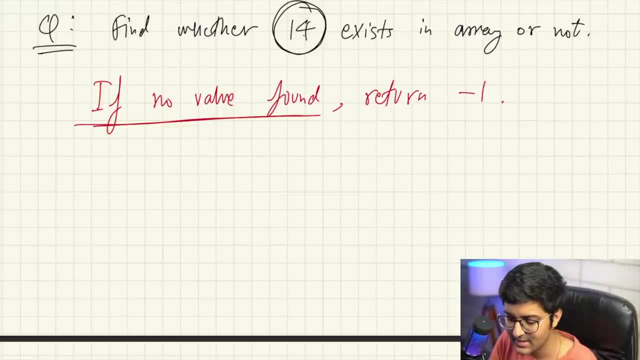 of what space complexity is, what time complexity is, then this will be helpful to you. so, basically, the time complexity. i'll explain it to people who are not aware of this thing as well, so don't worry, we have a separate section on time complexity that will be coming soon, in which we will be discussing 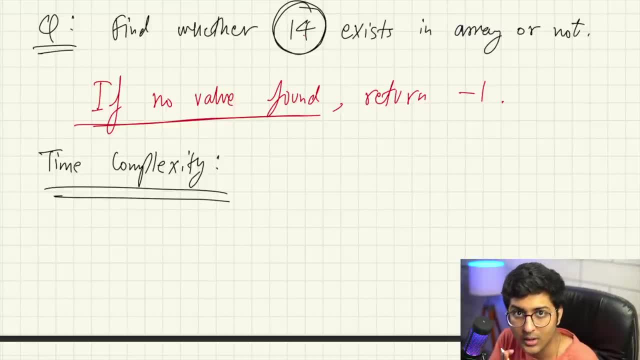 what is big O notation, how that is written in mathematics, what is the significant or significant of it. you know what is the intuition behind it in words. we will be writing everything in formulas and everything we will be covering, but for now in simple language for those of you who know. 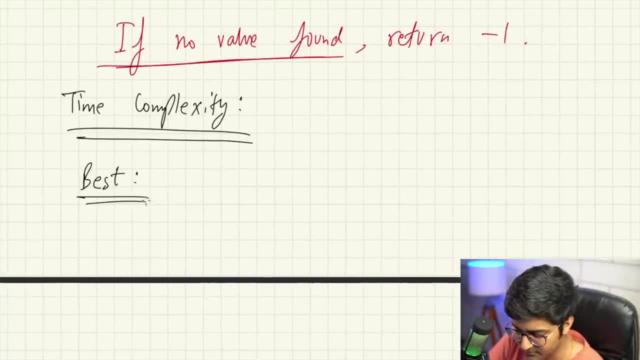 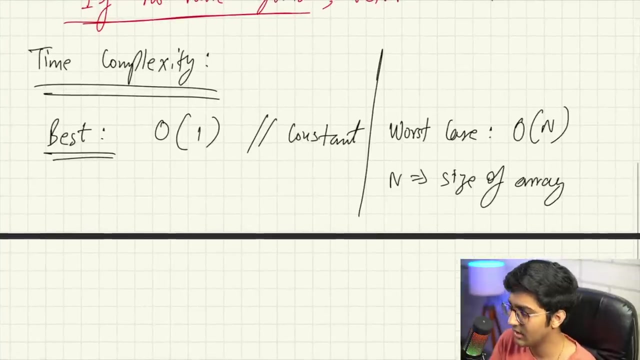 best case, complexity of linear search, is what big O of 1 means constant, and worst case is big O of n, where n is the size of the array. for those people who don't know what big O is, what is time complexity? don't worry, we will cover it in the later sections. for now, don't worry about. 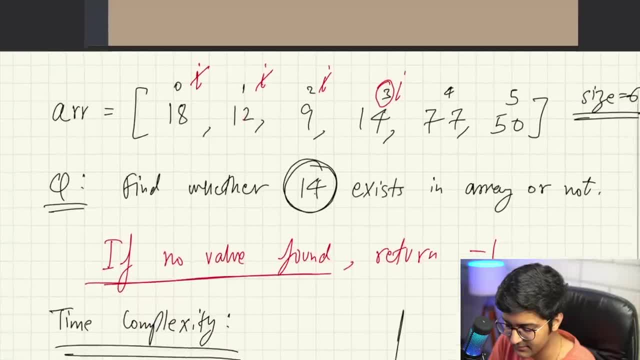 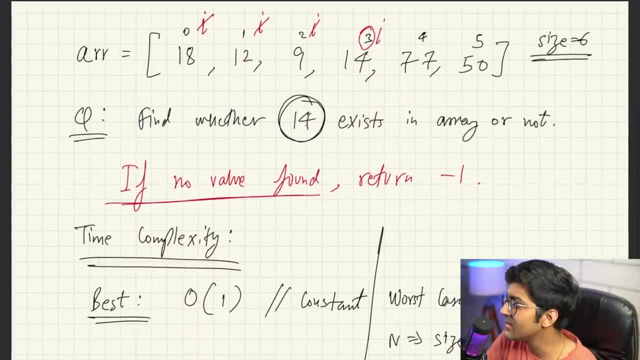 what is this big O notation? constant basically means that if you're trying to, let's say, this is for people who are, like, not aware of what is time complexity. so time complexity basically means the amount of you know, basically not the amount of time, but how your time is going to grow as the 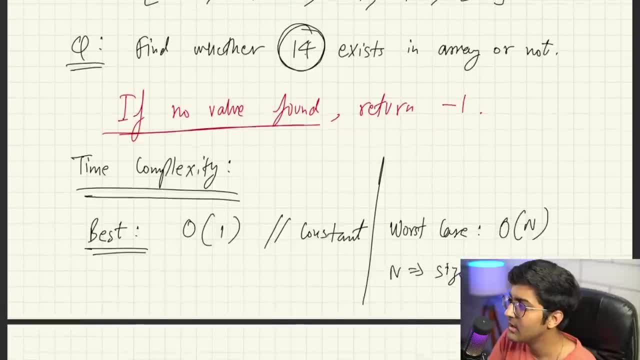 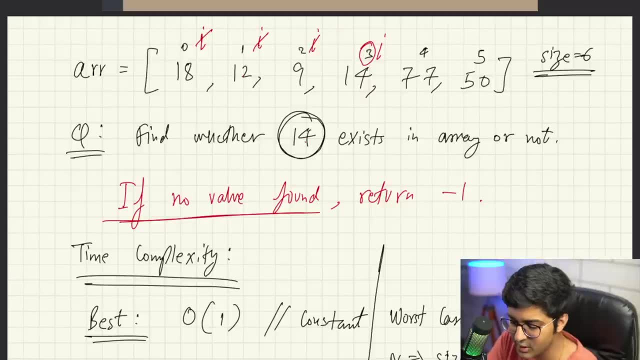 input will grow, don't worry about it. we will cover it in detail, but the idea over here is that let's say, in the best case, forget about time complexity. okay, what is the best case going to be when you're searching for an element? that is the question. 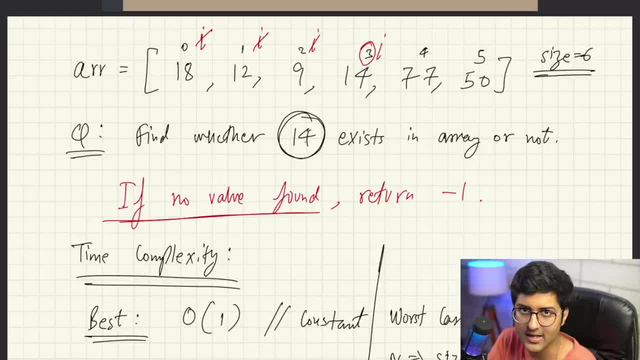 what is the best case going to be? you are searching for an element in an array. this is: it's an unsorted array. array is not sorted, it's unsorted. okay, what is the best case going to be? best case: your best life will be if the element that you're searching for is at the first index. 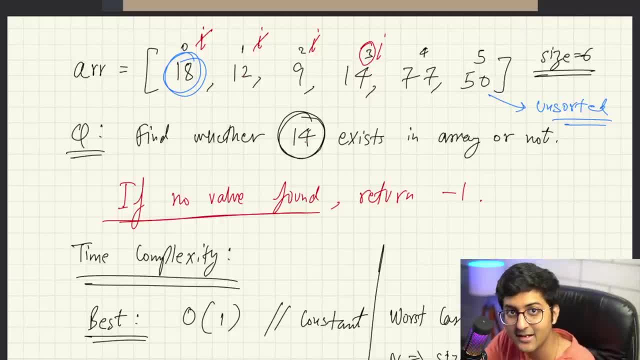 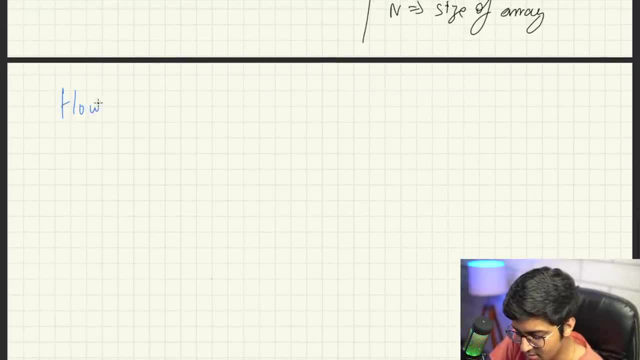 you have no need to search for the rest. that is like the ideal best case, right? in that case, how many comparables are there in the first index? how many comparisons will it make in best case? how many checks will the loop make in best case? that is element found at the very first index. 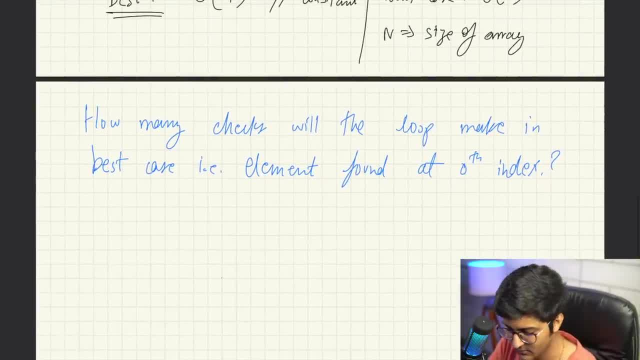 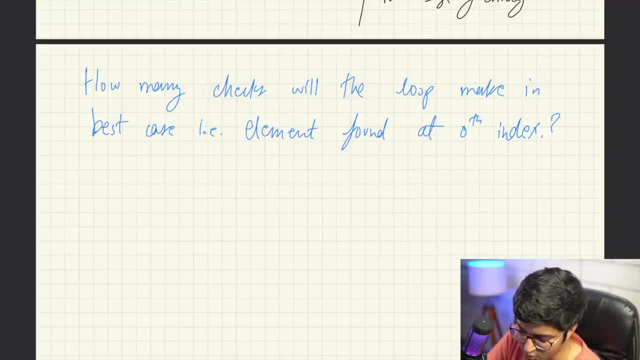 how many? let's say the size of the array is 200. okay, let's say the size of the array is, and you are searching for something like this. let's say: let's say the size of the array is 200. let's say the array is something like this: 8, 9, 12, 18, 200 elements. 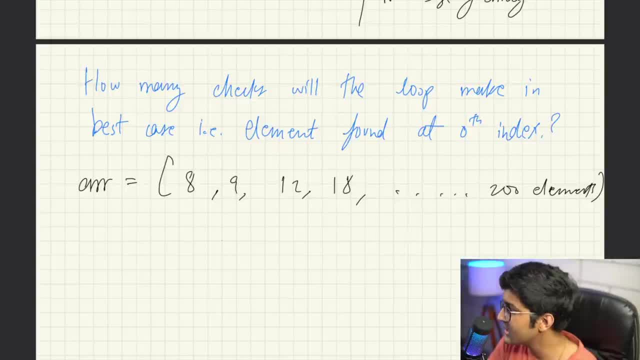 okay, let's say the array is something like this: and let's say: you want to search. my target you want to search is 8. so it's going to start from here. it's going to be like index number 0. it's going to say: is this equal to 8? yes, it is. it's just going to return 0. 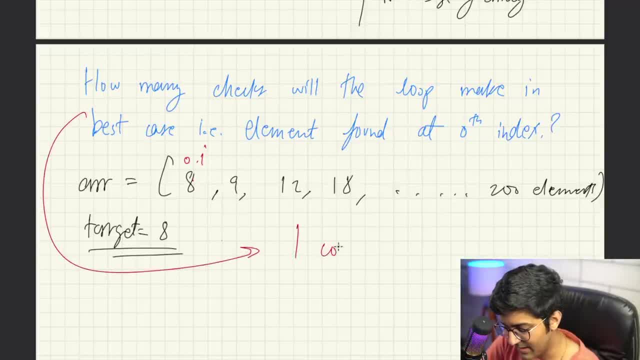 how many comparisons did it make? one comparison only in the best case. let's say this was, let's say, another example maybe the array of size. let's say the array is now of size 1 lakh. let's say the size of array is now 1 lakh. and let's say the item. 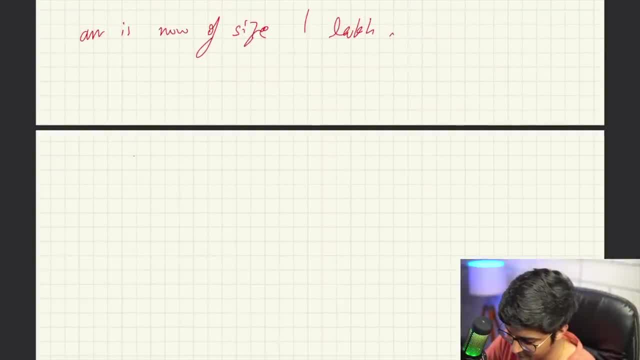 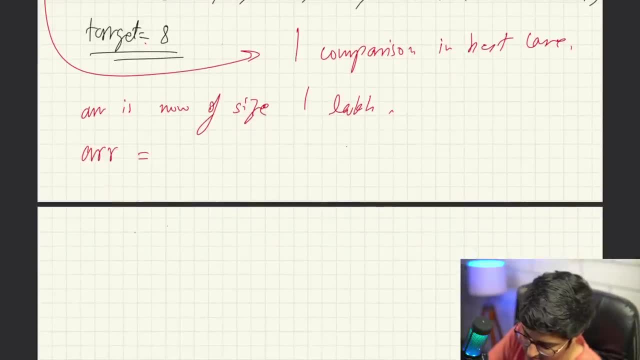 that you are searching. let's say it's something like this. let's say array is equal to something like this: 18, 12, 9, 7, 1 lakh items in the array. let's say you want to search for 18. where is 18 going to lie? it's going to check. is 0th index equal to 18? 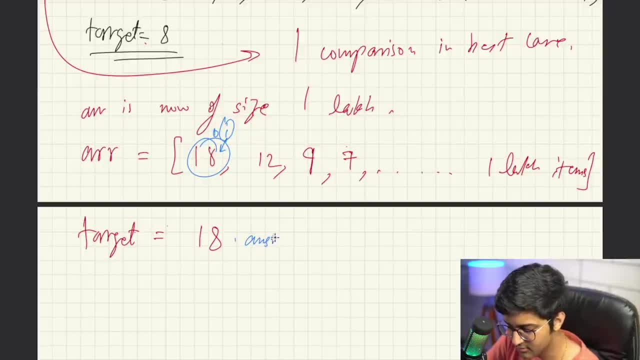 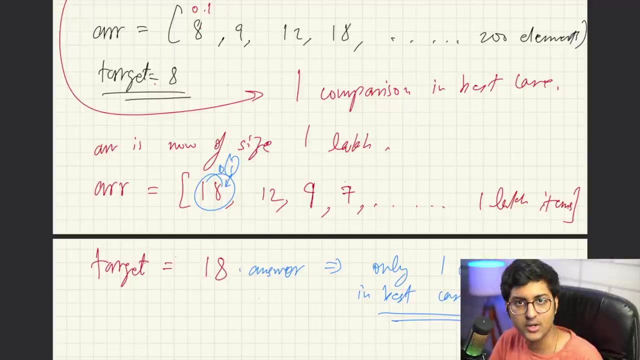 i is pointing to his yes answer- only again, one comparison made. only one comparison was made, right in best case. in best case, only one comparison made. this is for people who don't know what space time complexity is. okay, so time complexity basically over here, as you can see the number of comparisons. 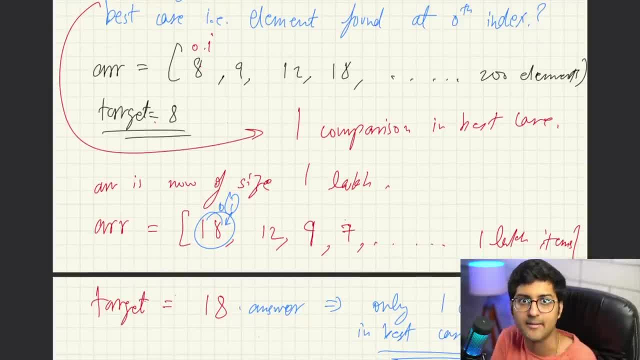 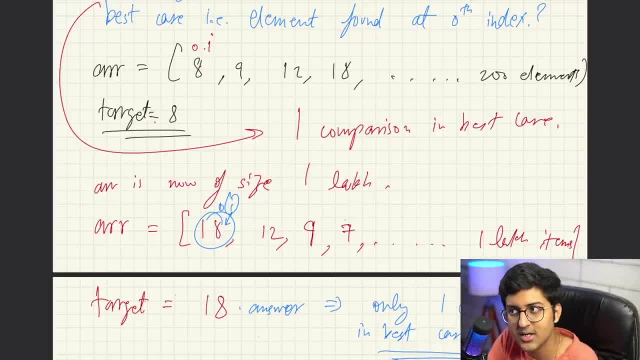 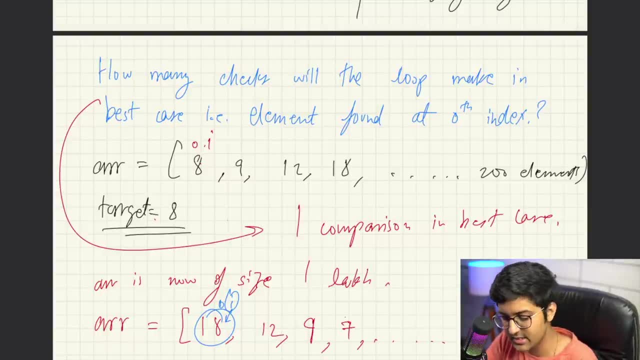 this is my ideal happy world. like okay, not much, i had to do, only just one one check in the for loop. like hey, is the 0th index l equal to the item it's going to be? like yes, it is, it's just going to return the 0th index here. it does not matter how many elements are there. in the best case, in the 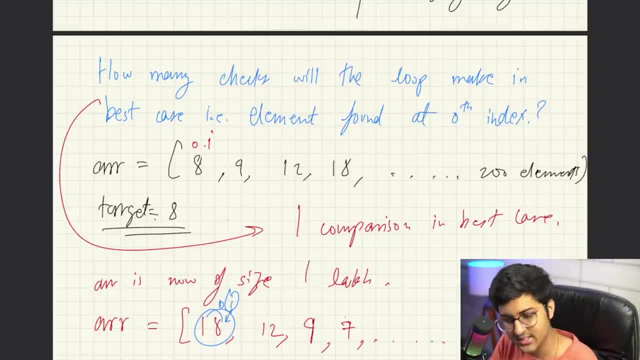 best possible scenario, if the item is lying in the very first index, at max, it's only going to make one comparison: is this item equal to the target element? if it is- in the best case it would be- it will just return that. so here you can see, in the best case the size is not mattering, the size of the array does. 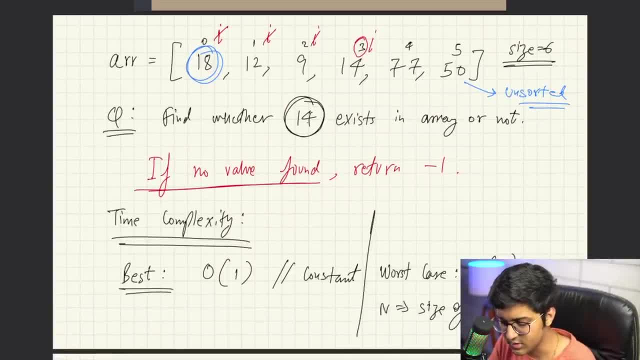 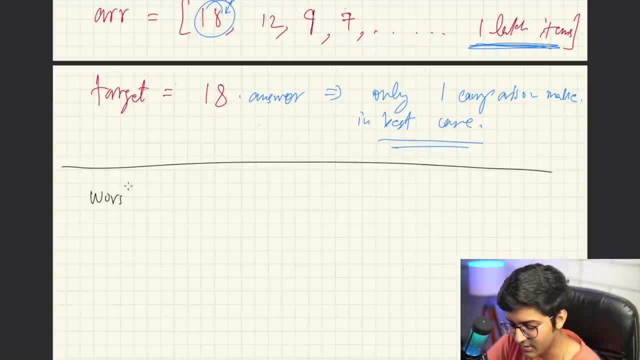 not matter. that is why time complexity is constant here. let's say, if we talk about the worst case, what is the worst case going to be? you tell me. i mean, how can you tell me? you are watching the recording, but you all know what is the worst case. pause this video. 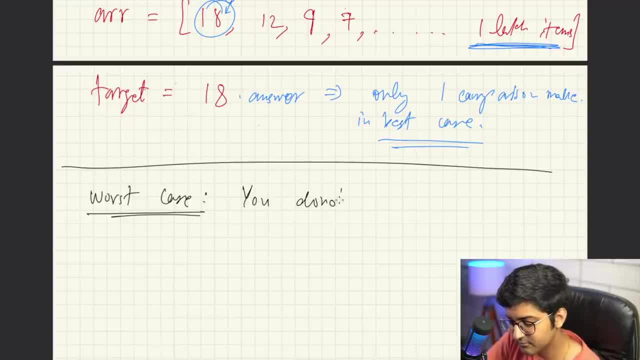 worst case is you do not find the item. that is the worst case. you will iterate through the entire array. you will check every element one by one in the for loop and in the end you will say: we have not found the item. okay, iterate or go through every item. 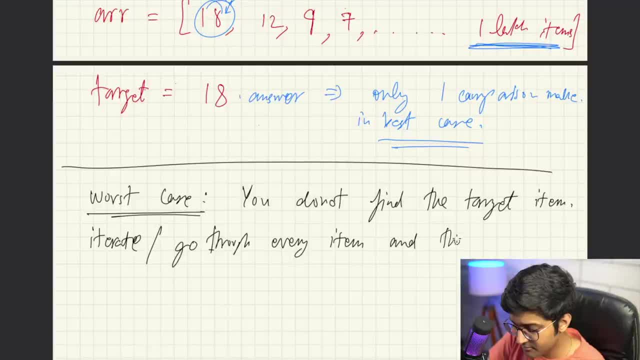 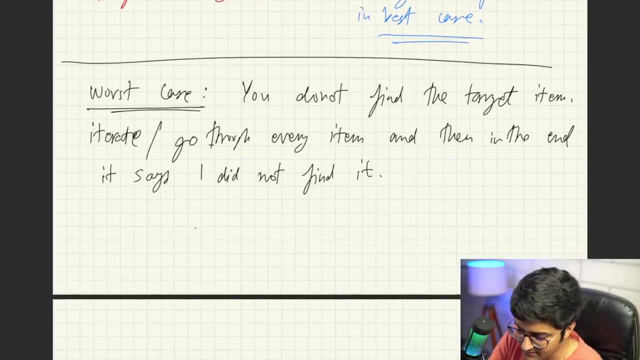 and then in the end it says: i did not find it so. another important point over here: if the size of the array, if the size of array is equal to 100, then it will make 100 comparisons. you know, loop will run 100 times and after running 100 times, after iterating through every item, in the worst case, when the item 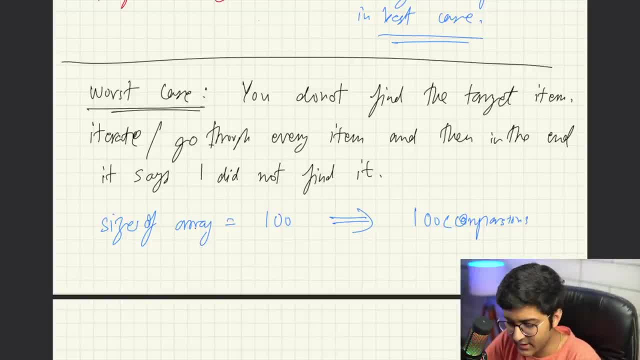 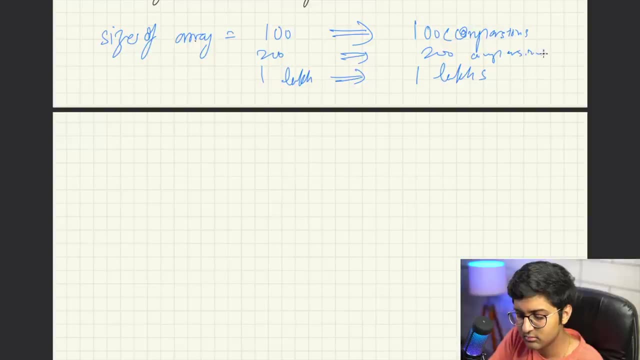 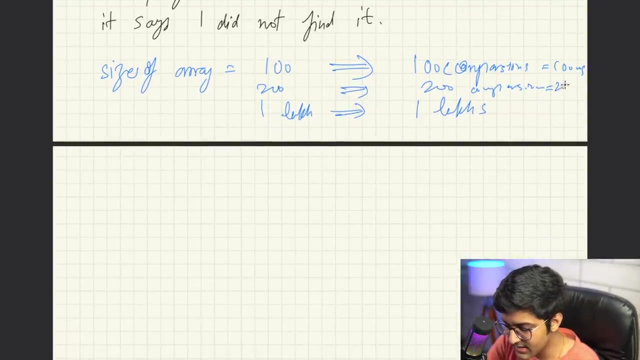 is not present in the array, it will say, hey, item does not exist. if the size of array is one lakh, it will make 1 lakh comparisons. okay, if the size of the array is 200, it will make 200 comparisons. okay. imagine this takes 100 millisecond. imagine this takes. 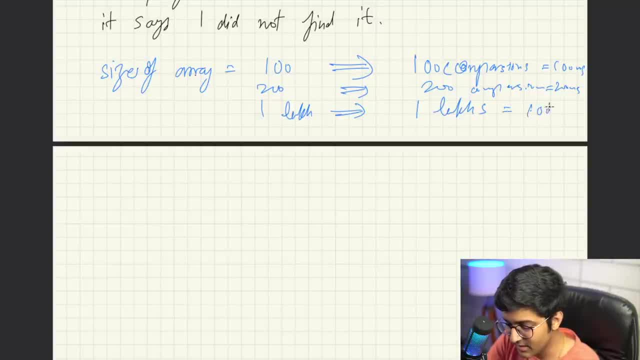 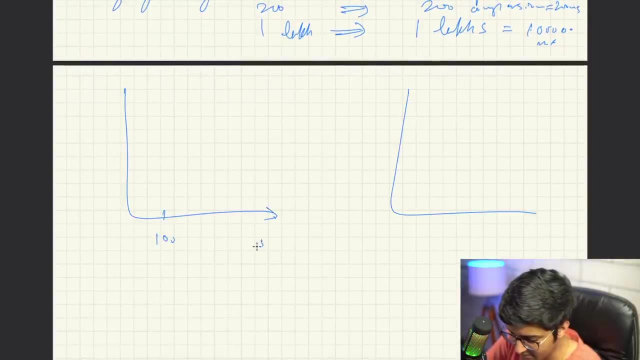 200 millisecond. imagine this takes 1 lakh milliseconds. what is 1 lakh milliseconds? 1 lakh milliseconds? let's draw a graph of this here. it's saying, for 100, size of the array. in the worst case, this is, let's say, the time taken in milliseconds for 100. 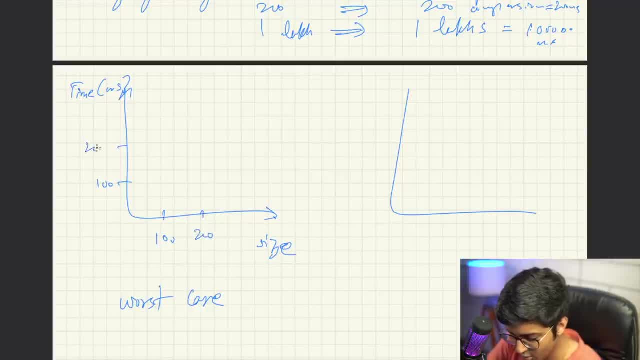 size, it's taking 100 millisecond. for 200, it's taking, let's say, 200 milliseconds. for 400, let's say it's taking 400 millisecond or something. if i draw this on a graph and you see that this is forming a linear graph, a single line. if i want to say for 500 items, 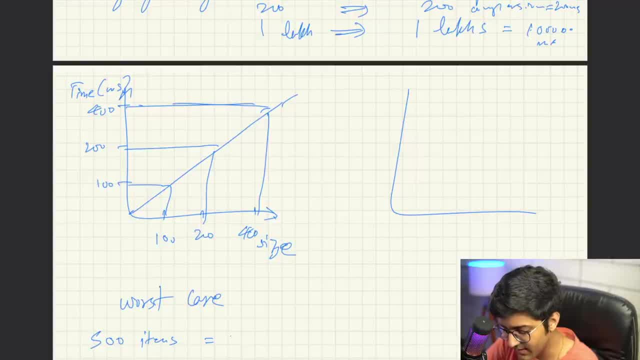 guess how much size would it be taking? so around around 500 milliseconds. can we say this looking at this graph? this is known as linear time complexity. this is what time complexity means, as the size of the input is growing, how my time is growing. that is called time complexity. 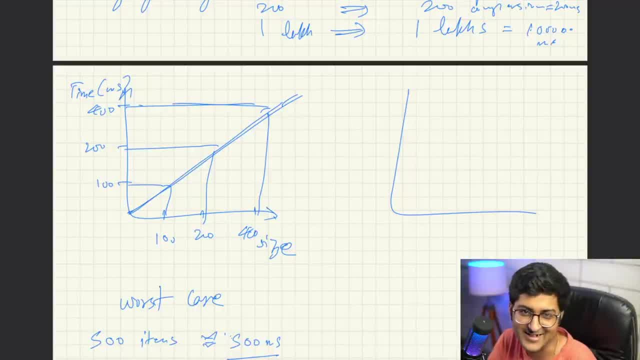 even though this lecture is of linear search. now you learned about time complexity as well. okay, let's talk about constant in the best case. in the best case, let's say the size and let's say the comparisons or the time taken. so let's say, in the best case, you know that it will only lie, it will only make one check. 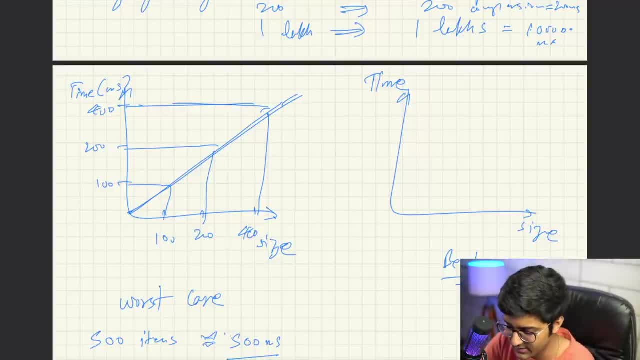 because in the best case, item will be at the very first index, at the zeroth index. the size of the array is 100. it will take, let's say, some one millisecond. size of the array is 200: it will only take one millisecond for that also. size of the array is 100, it will take, let's say, some one. 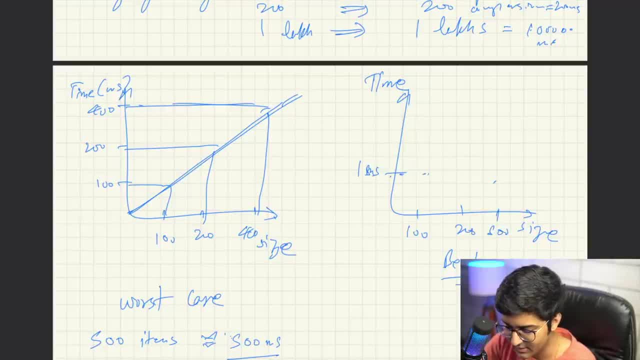 so size of the array is 500, it will take one millisecond for that only. size of the array is 1 lakh, it will take one millisecond. it does not matter what the size is, it is taking constant amount of time. this is constant time. complexity- okay, constant is like we will discuss more about. 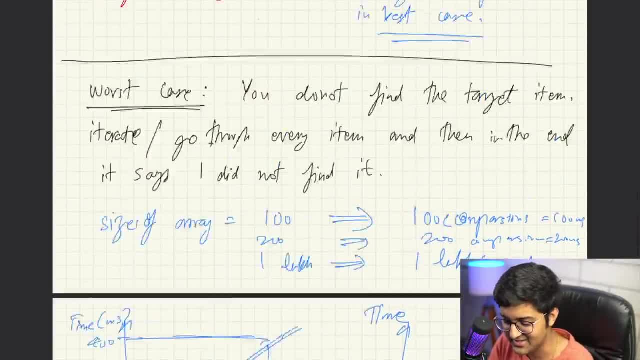 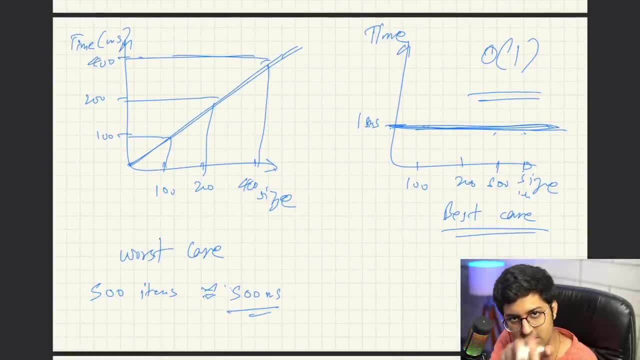 this later. i'm going to stop now because i don't want this to turn into a time complexity lecture. but as you know now that, uh, the worst case time complexity of linear search is big o of n, don't worry about what is big o notation, we will. 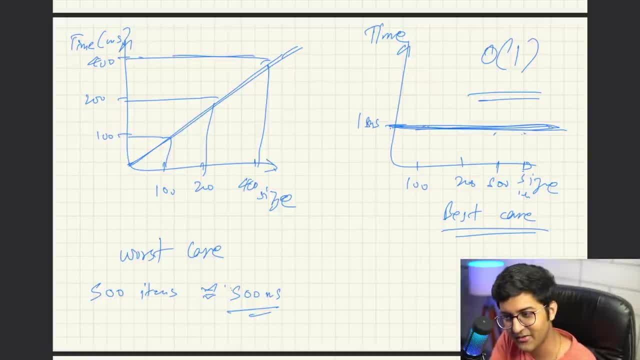 cover big o notation. in the end, if you want to get a little bit of hint, it gives you like the upper bound of the complexity. so basically it's never going to go worse than big o of n, worse than linear. basically big o of n means it will never go worse than linear. it can go better than. 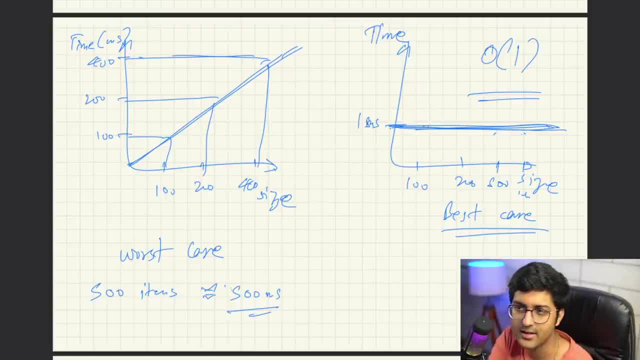 linear, like big o of 1, big o of log n, but never works than that. forget about it. if you're new to it, never mind forget, i will cover it in detail. it's going to be a really long, like one hour, two hour long lecture. it will be like a literally a two hour long. nice, everything you need to know. 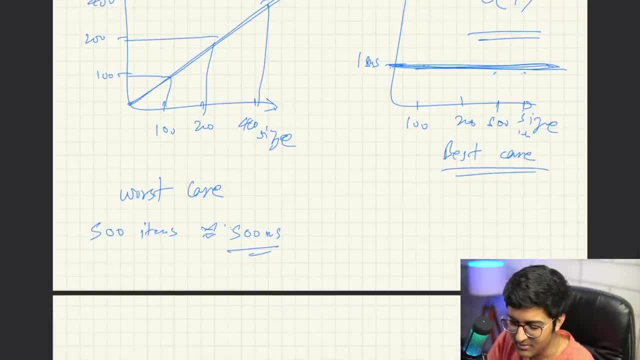 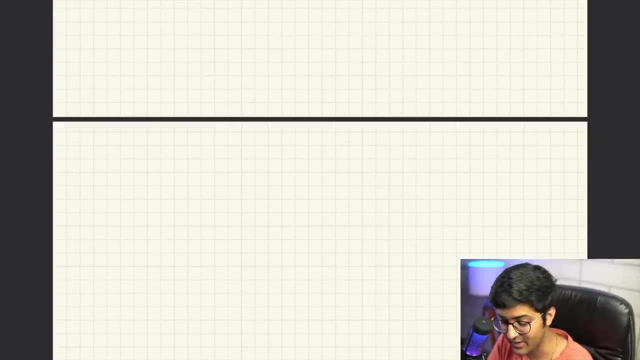 about space and time complexity lecture. we will do it in a very amazing way, but this is just a basic understanding it. time complexity is amount of time taken. uh, you know, it's not not the amount of time taken. time complexity is how the time grows, as your input grows. that is the for linear. 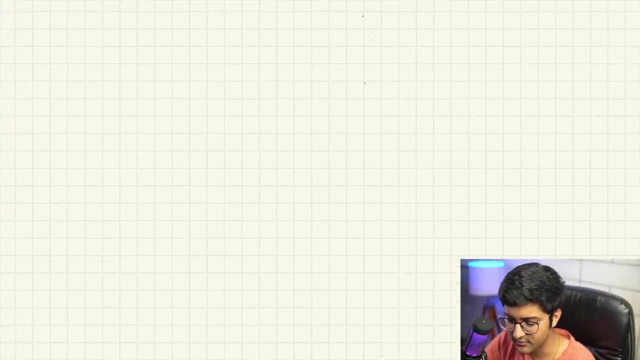 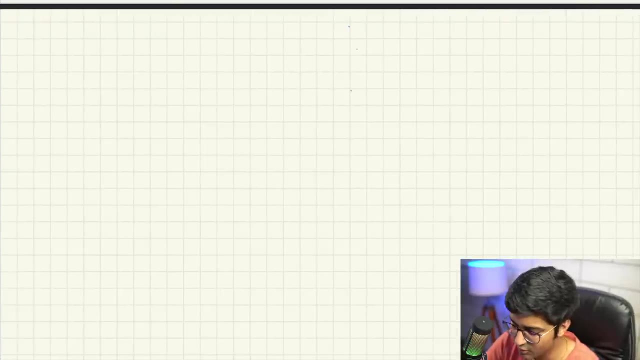 search. its best case is: o of 1 means constant. we already discussed that. worst case is um big. o of n means linear. time will grow linearly as the input grows. we also saw that space complexity is also constant. space complexity basically means: are you taking any extra space? okay, if you want to search through. 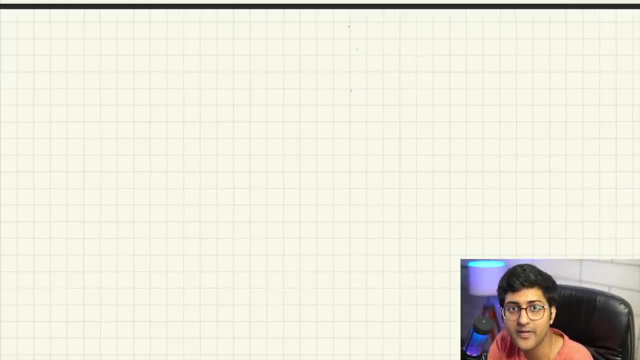 the array. are you making any another array? are you making a copy of that array? no, i'm just taking a few variables, that's it. if the size of the array is 10 lakh, i'm only taking one variable, which is the for loop of i, the, i index, checking everything, and maybe we'll take one- yeah, one- target element. 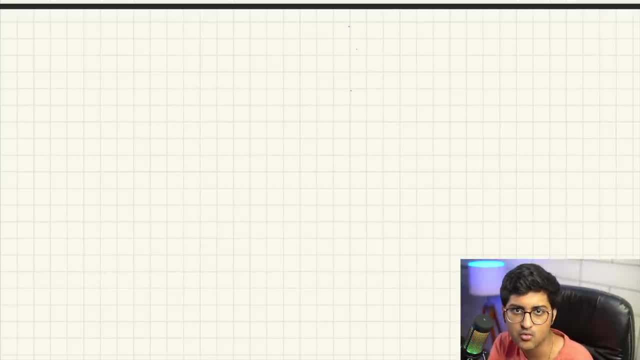 two reference variables only. if the array of size is 200, we are only taking two reference variables. so space complexity also we will discuss in detail. this is known as auxiliary space, means extra space taken. no extra space is being taken over here. we will discuss that later on. for now let us now look into. let me see if i missed something. so we talked. 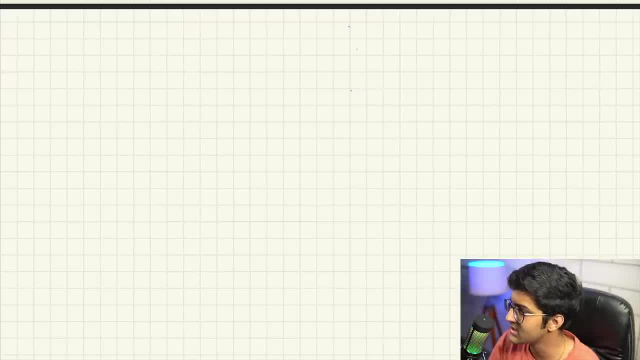 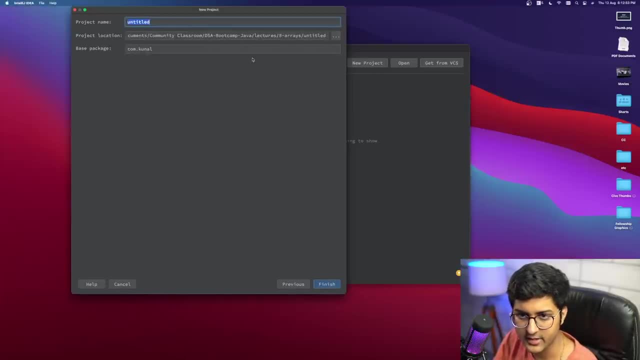 about introduction. we talked about best case scenario. we talked about worst case scenario. now let's look into the code base. so i'm just going to create a new project here. we have already covered intellij, idea and everything. if you new to java, check out the link in the description. there's an entire playlist available over there. 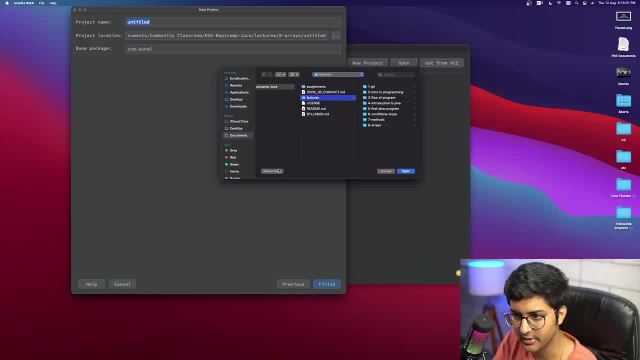 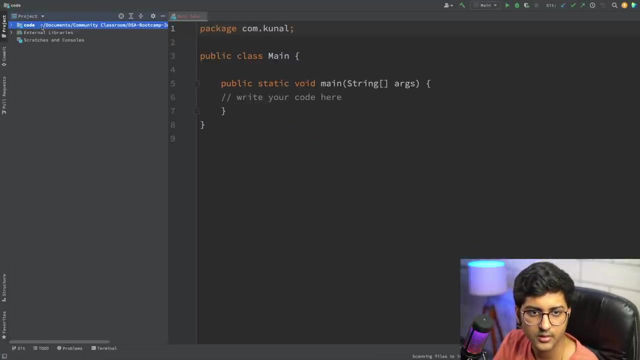 i'm going to create another lecture. i'm going to say lecture number nine, linear search, cool, and we'll create a folder over here called code open. finish, gonna gonna do the linear search code over here: don't show tips, close, very nice. okay, let's create separate function for it. let's say, for linear search i can say static. 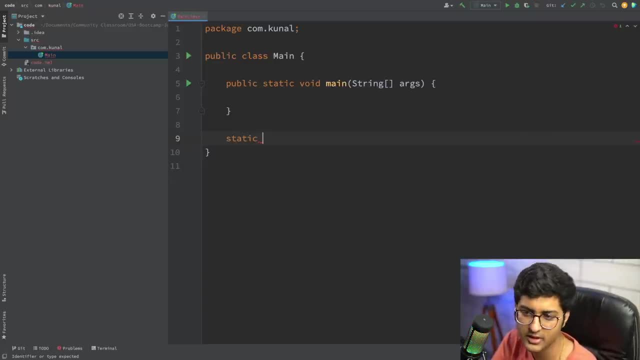 we all know that we are not worried about why we are starting static over here. i already covered it in functions and we'll go dive deep into it, like in the, you know in the um tutorial, like of object into programming. but let's say first we try to, you know, sort the array in place, like sort the array. 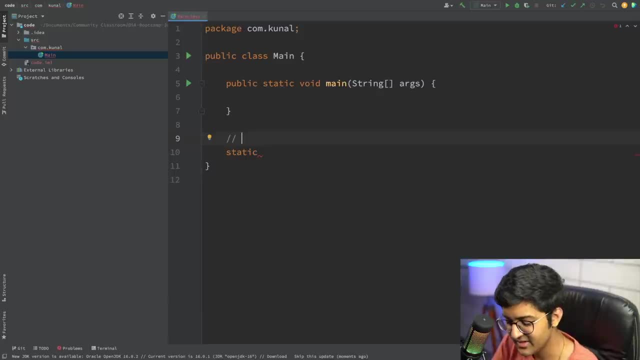 sorry, why am i writing sort? ah, really need some sleep. search in the array. so here we are, searching in the array. so we are basically going to return the index if item pound. otherwise, if item not found, return minus one. okay, so i'm going to return an integer static. i'm going 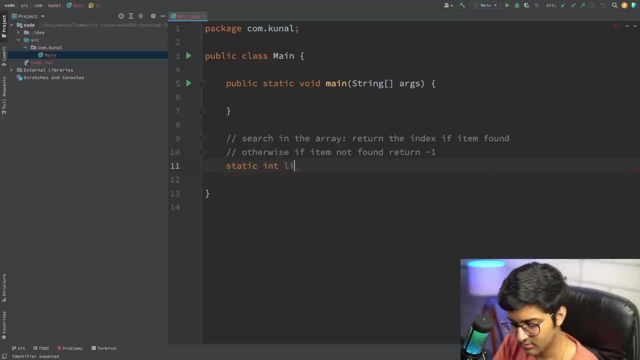 to say: int, um, linear search is my function name, any name i can give. it's taking an array. okay, now i'm just going to say some basic checks. i can say: if arraylength is equal to, equal to 0, then i'm just going to say one more thing i missed out. what do i want to search? 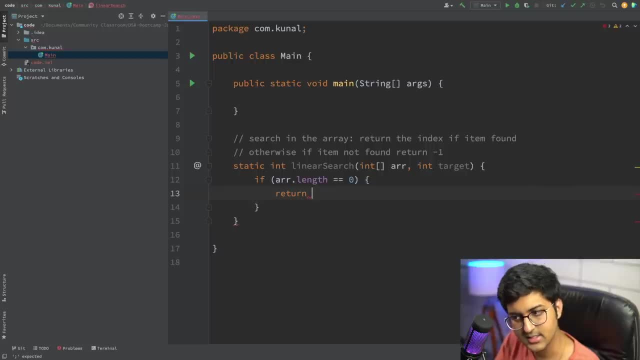 my target element i want to search. so if array length is 0 i can just say does not exist. otherwise i'm just going to run an integral setting of. again, it's the nochmal function. everyone knows it gives a little surplus time to re stupidly give a. 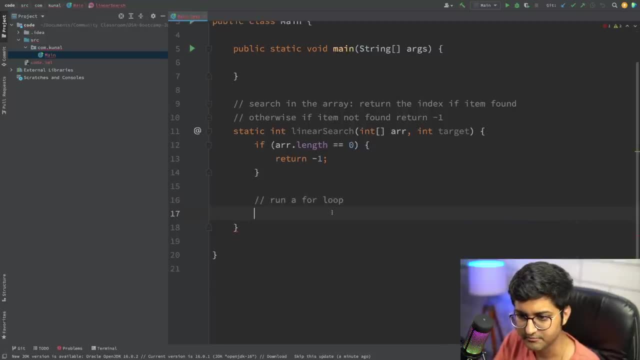 run a for loop. i'm going to say for i zero, i is less than um. you know that is length, i plus plus. basically it's just going to go till the index of the. a like the. you know if it's like, if the length of the array is six, so it's just going to i is just going to go less than six, basically. 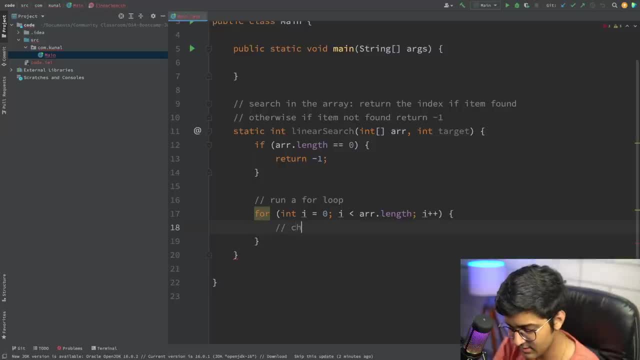 till five only then. so for every index, check, check for element at every index if it is equal to a target that we want to search. basically, i'm going to say my element is going to be arr of i if the element is equal to, equal to the target that i'm going to search. 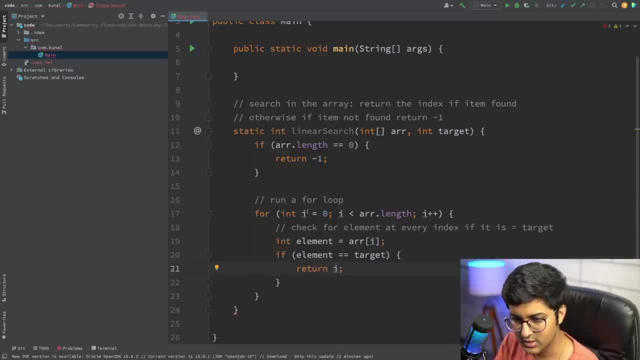 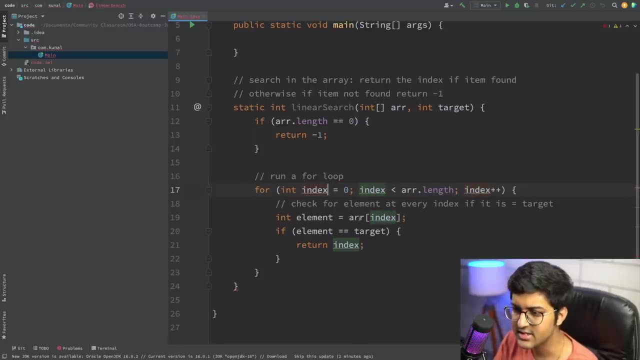 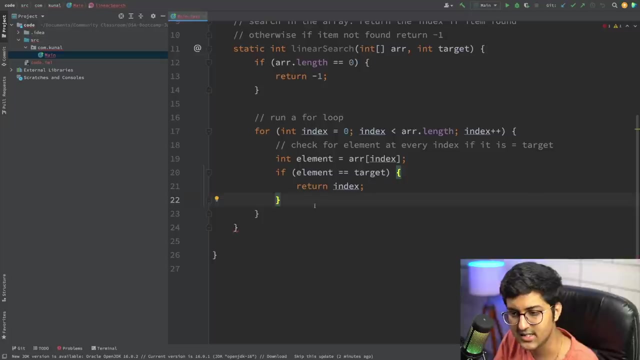 i'm just going to return the index i i can actually change this to. i can rename it to index. so you are able to understand. i just did a refractor. refractor basically means you can change the name without doing it like individually. it basically changes the name of all the occurrences, basically just right click refactor. 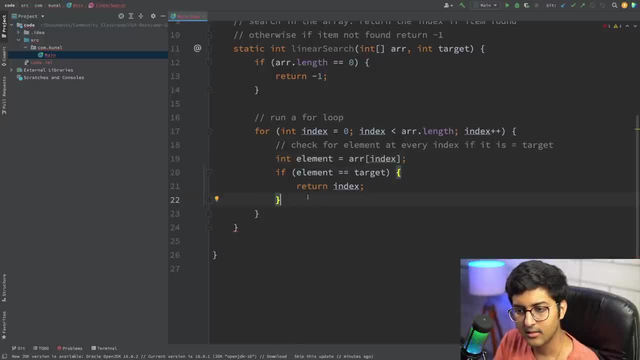 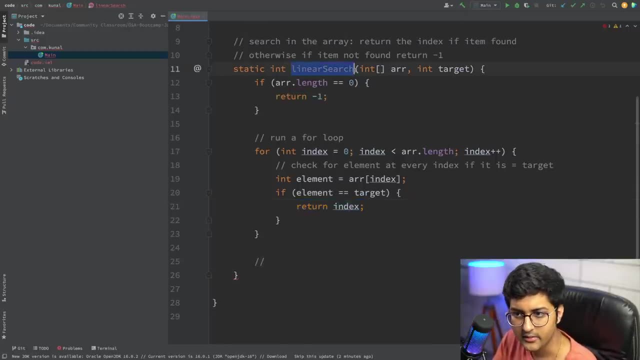 rename. that's it. okay, uh, that is it. and we all know in functions we learnt: whenever the return statement is hit, it means that it will return like: uh, it will come out of this function. it will like: end the function and you'll come out of the function and it will come back and it'll work. 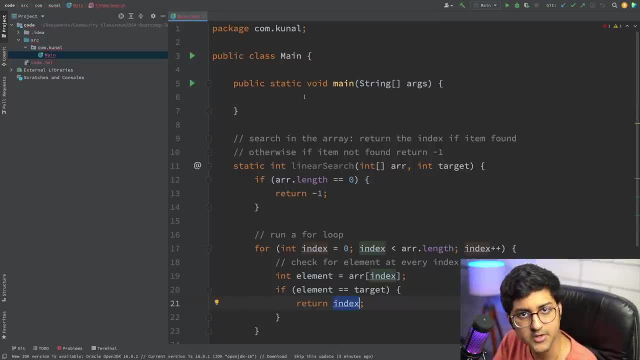 and after few six days, meeting r is or return end, then it will like pop up, but not for the will return the value wherever this function is called. so if you want to learn more about how functions are working. so basically, if i have an array like this over here- integer array- 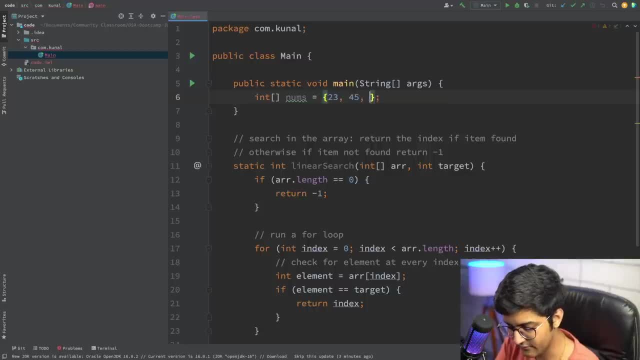 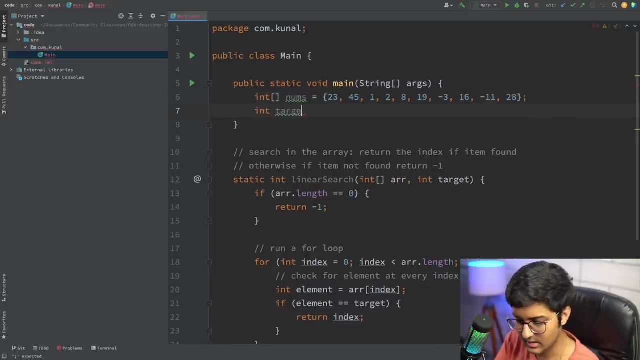 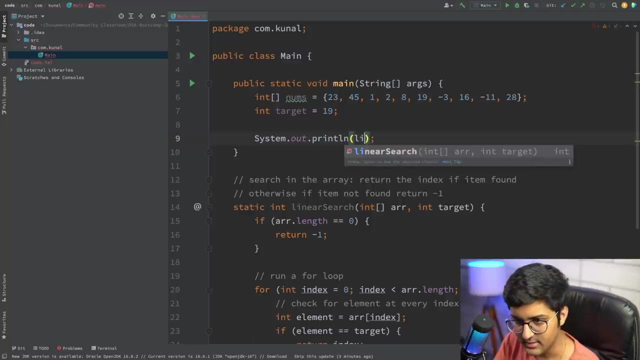 nums is equal to something like this: 23, 45, 1, 2, 8, 19 minus 3, 16 minus 11, 28 or whatever. let's say my target is equal to. let's say you want to search for 19. you can just print out my linear search or i can just say my. 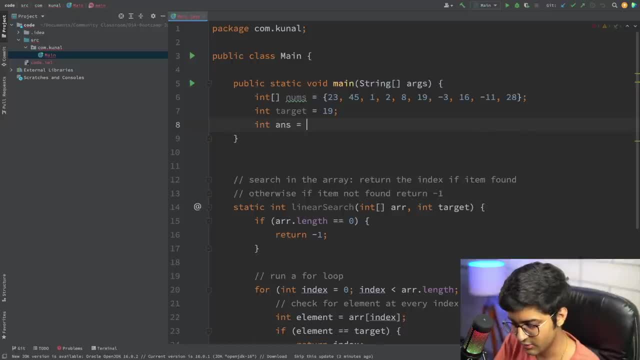 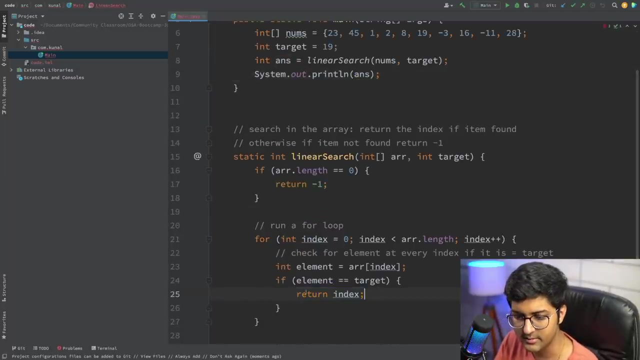 answer is going to be: i'm going to call linear search, i'm going to pass an array to it, so nums, and the second thing i'm passing is target, basically my target, okay, and i'm just going to print the answer. so return. as we all already know, return basically means this function will end and it will return. 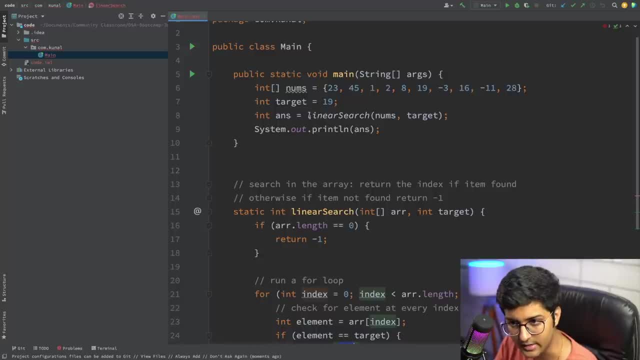 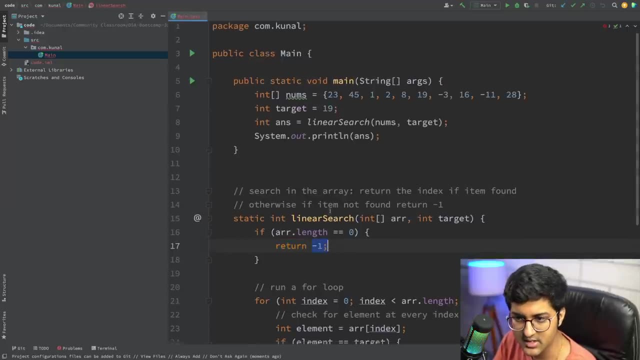 this value. this value will be returned to the function call here. this entire values, this entire function calls value will be whatever is returned over here or here, whatever if minus 1 is returned, this value will be minus 1 and it will be stored in answer. so answers value will be minus 1 and. 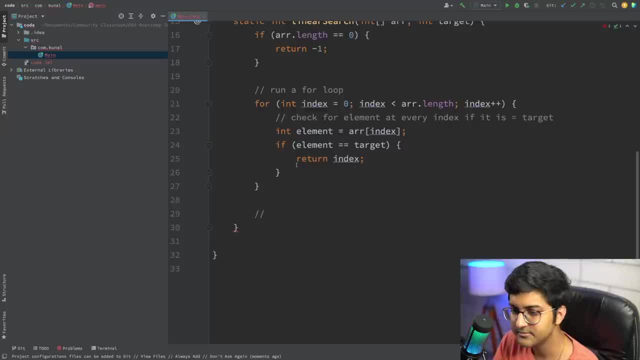 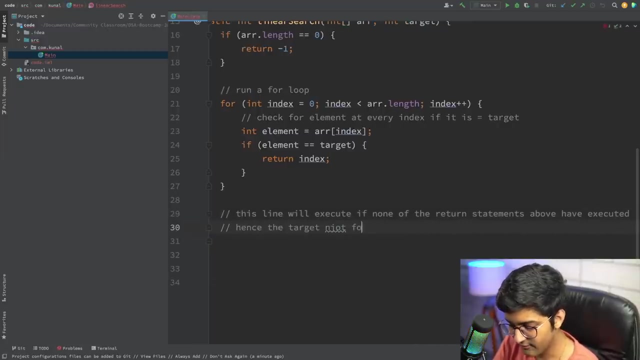 it will print minus 1. we have covered this in detail in functions, don't worry, check out the links in the description otherwise. so, basically, we know this line will execute, obviously if none of the return statements above have executed, hence the target not found. okay, so if no return statement is hit, it means that you know no target has been found. 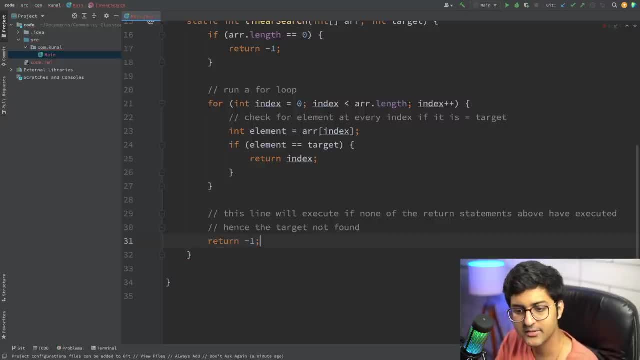 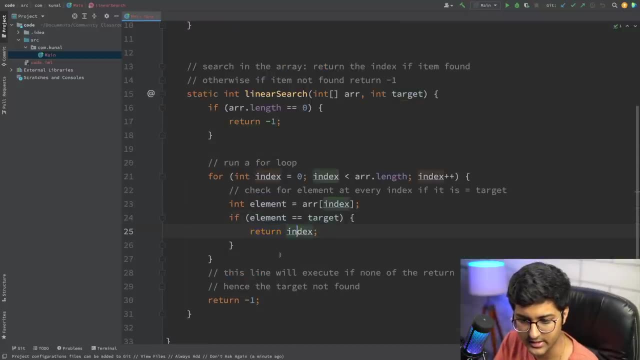 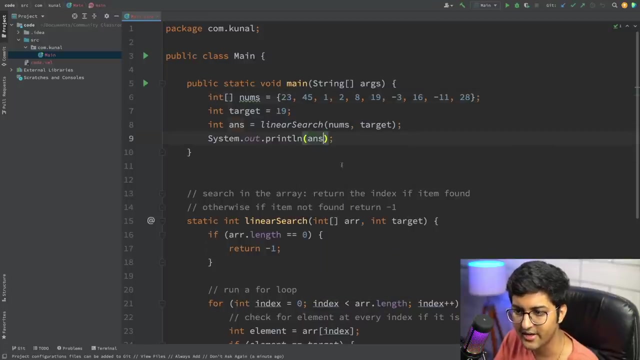 means the element does not exist in the array, just return minus 1. that's it searching for every element. if element equal to target, return the index, otherwise return minus 1. let's try to print this. it should print 0, 1, 2, 3, 4, 5. index number 5: 19 is at index number 5. it should: 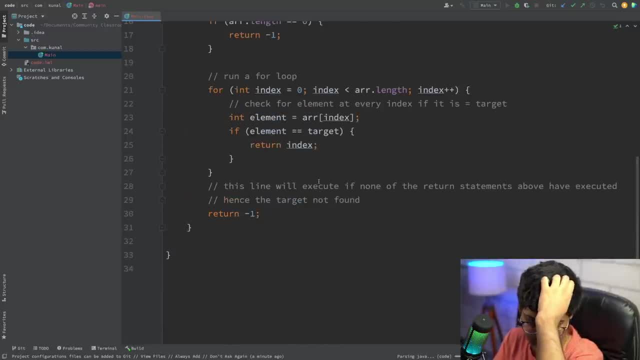 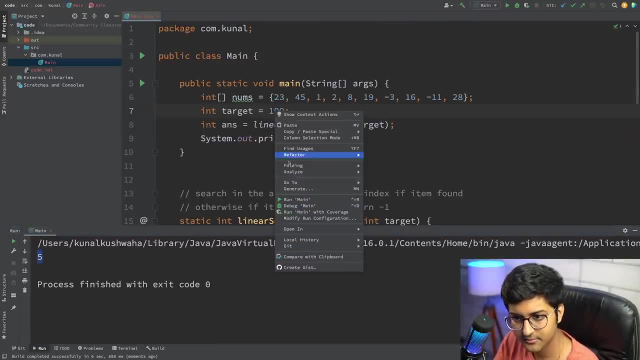 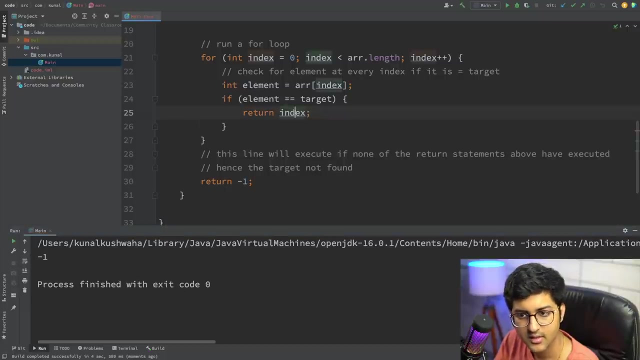 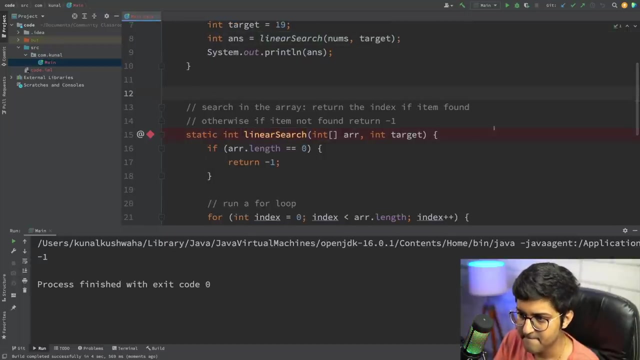 print 5, 5. let's try to search for something that does not exist. it will give me minus 1, minus 1. let's try to see how this is working internally by using a debug pointer. debug this now. you can see line by line how this thing is working. 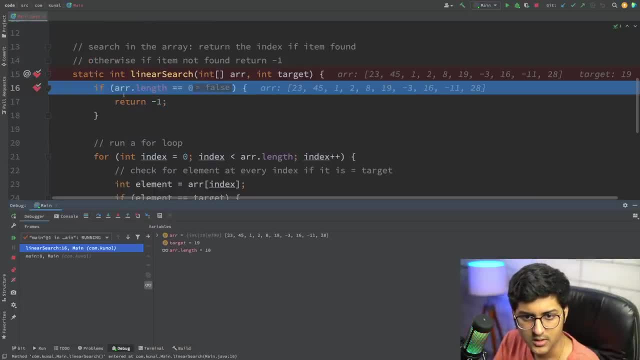 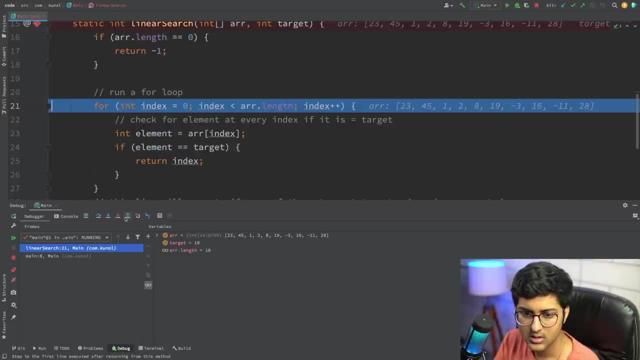 okay, so here it's going to check: is the length equal to 0? no, it's not, so it will be skipping this condition and directly going to the next one for loop. currently it's saying index is equal to 0 and the element at the 0th index is equal to 23, so it's going to check: is the length equal to 0? 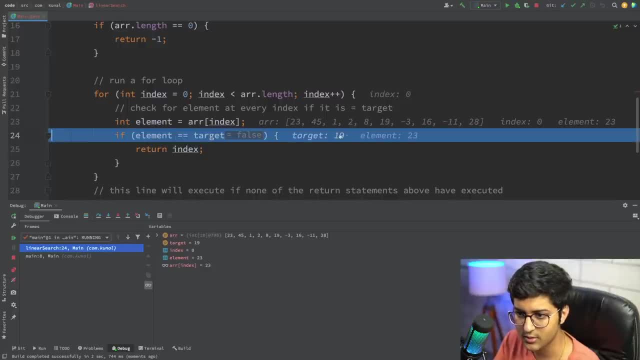 it says over here, then is going to say: is 23 equal to equal to 19? it's going to say, no, this is false, hence it will not return anything. it will move ahead in the for loop. so now index is equal to 1. as you can see, index is equal. 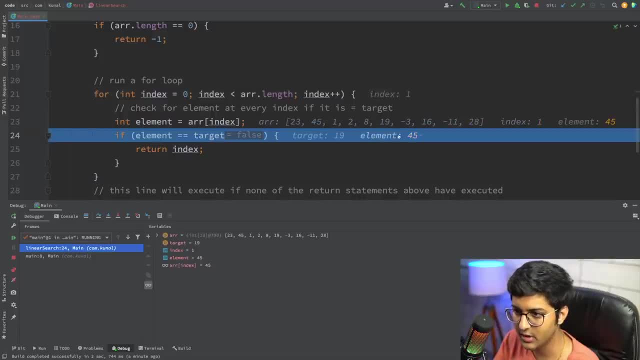 to 1 and my element is equal to at index number 145. element is 45: 45 equal to 19? no, it's not. move ahead. similarly, is 1 equal to 19? no, it's not. is a element 2 equal to 19? also is not. is 8 equal to 19. 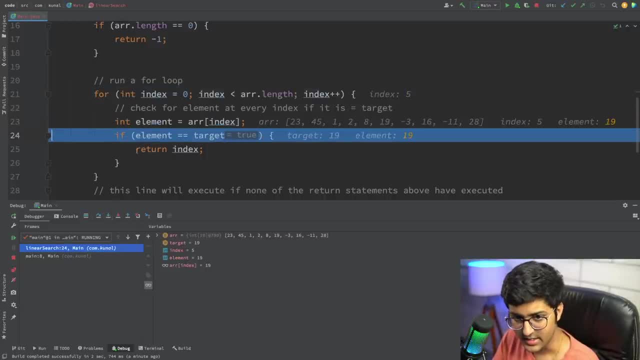 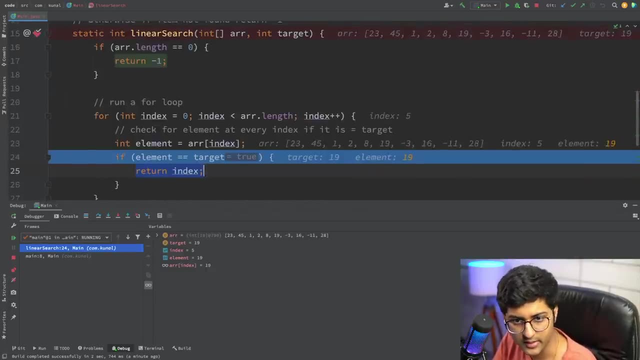 to 19? no, it's not. is 19 equal to 19? yes, it is. it will now notice return the index and it will come out over here. that is what i told you. when you return some value in the function, function gets over, so you can see it will return the value. now in the next line it will come out of the function. 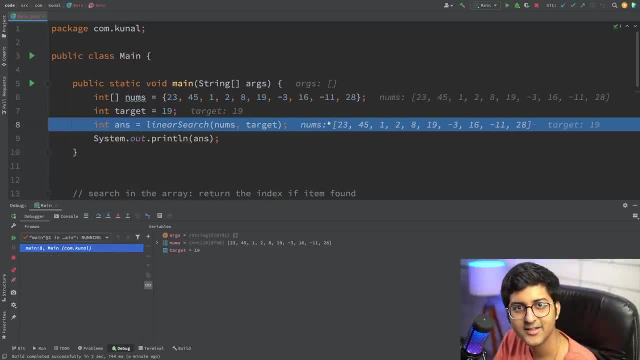 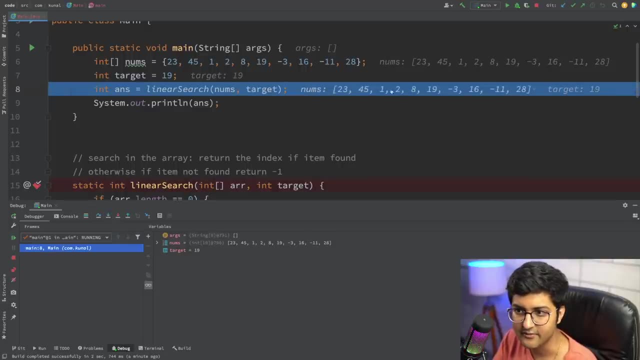 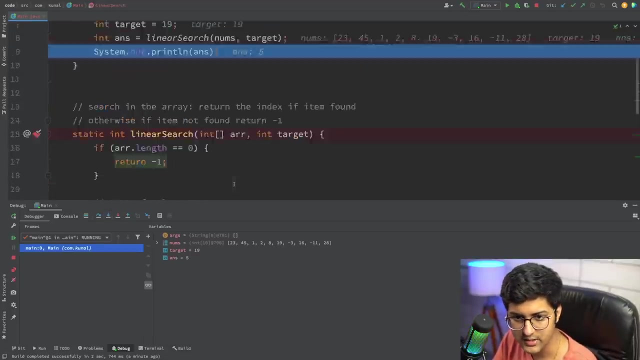 over here. now it's over here. function over. it's over here and the value is equal to 19. so answer will be sorry. 5, which is the index value that it returned. so answer is equal to 5. this value was returned. 5 over here here. 5 was returned, so this value is 5. it will print 5 and function program. 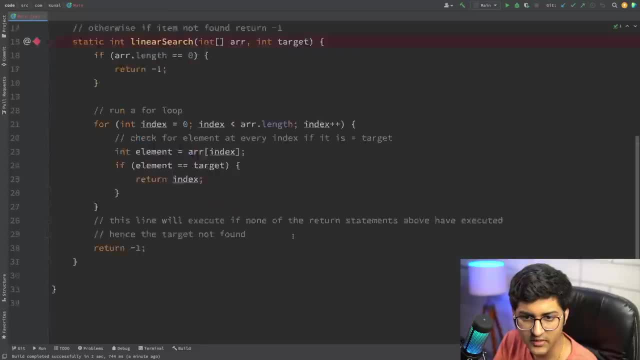 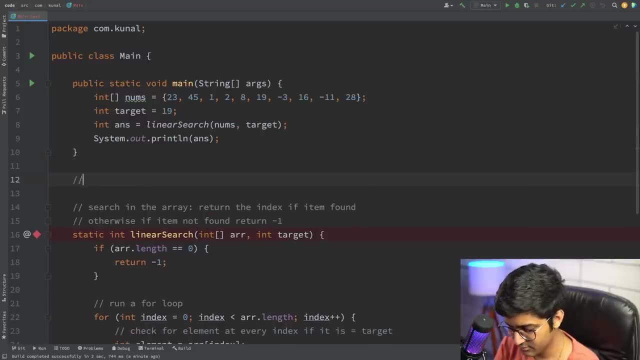 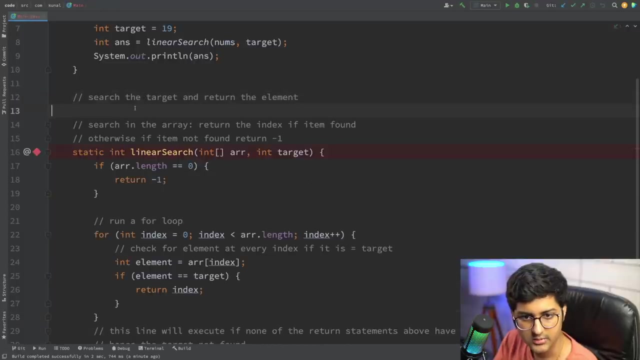 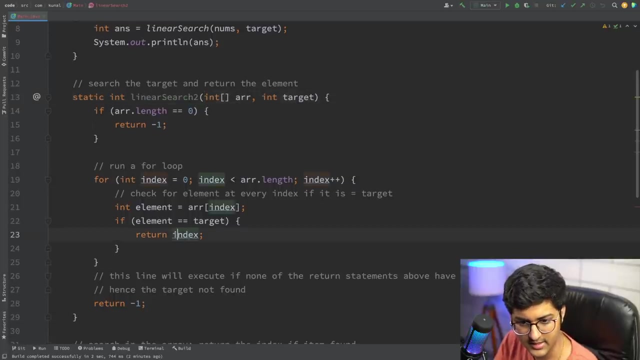 over. okay, we can do it in many other way. let's say you want to do something like you know: search the target and return the element itself. so let's say you don't want to return the index, you want to return the element. i'm just going to copy paste this linear search 2 and here, instead of returning the index, i can. 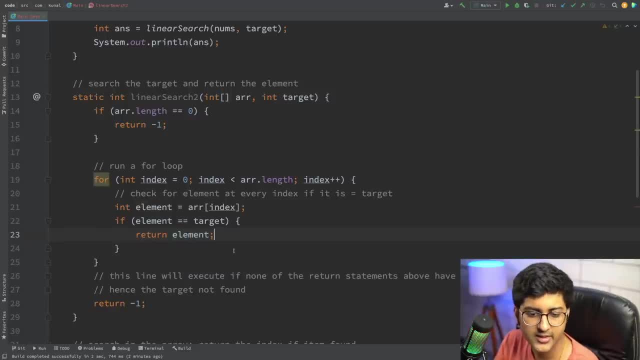 just say return the element. that's it. but since now i'm not making any use of the index stuff, i can replace this in a enhanced for loop for every element in the array. if i'm not making any use of the index stuff, i can replace this in a enhanced for loop. 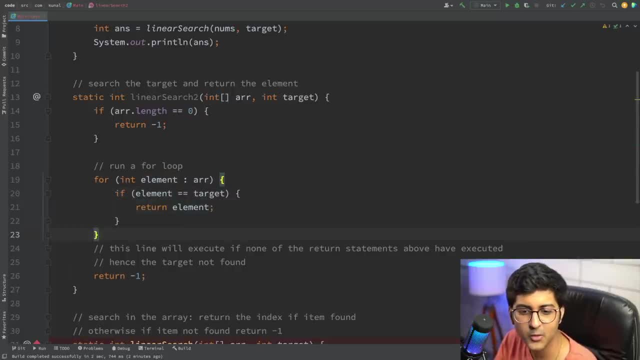 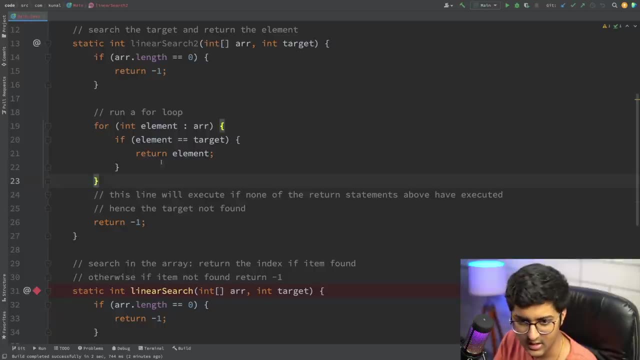 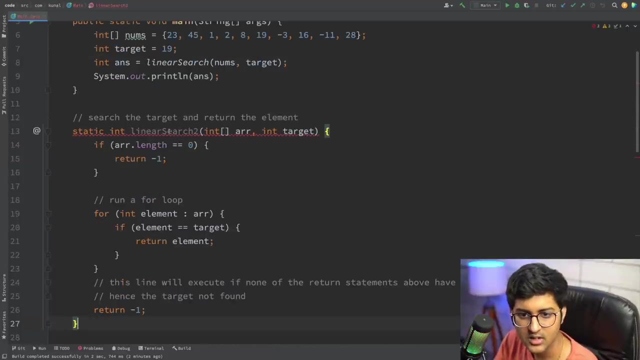 the element is equal to target. return the element for loop, enhanced for loop. we have already studied this in the previous like iterables, like on the all the like loop section. okay, let's say you just want to return true or false. that is also something you can do in your search 3. so search the target. 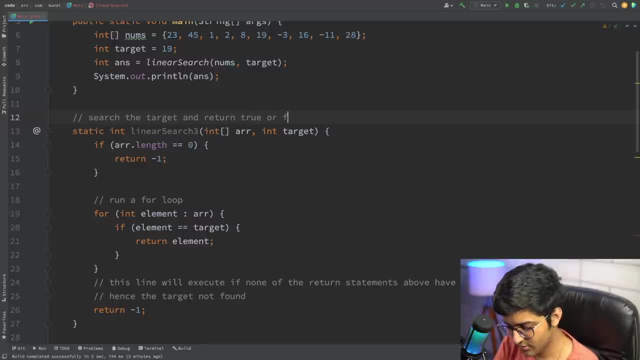 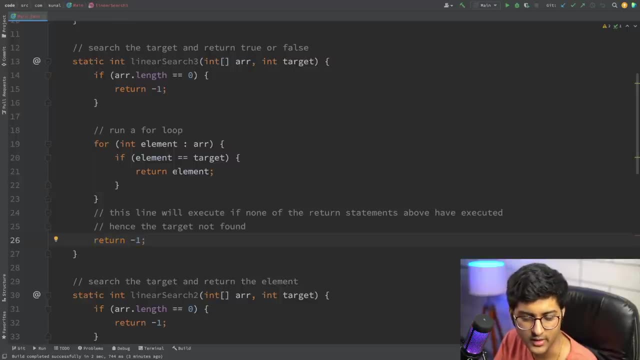 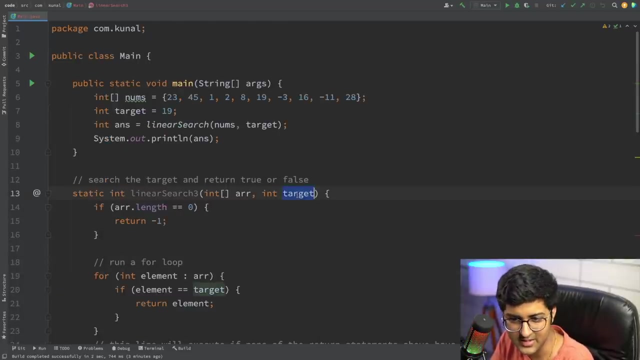 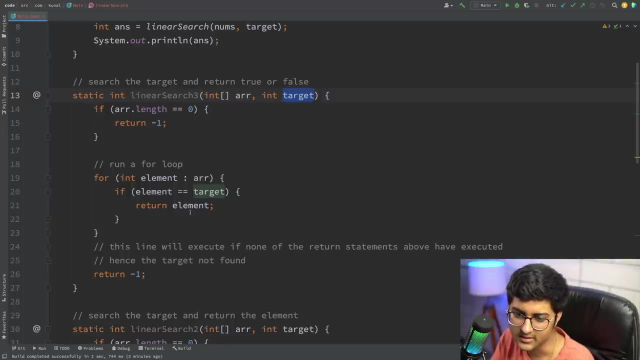 and return: uh, true or false. okay, in this case you have to uh worry about, like, okay, if element is equal to a, because in there might be a case that minus one by might be equal to the target. okay, so, in this case, uh, you know, um, yeah, it might say that, uh, if 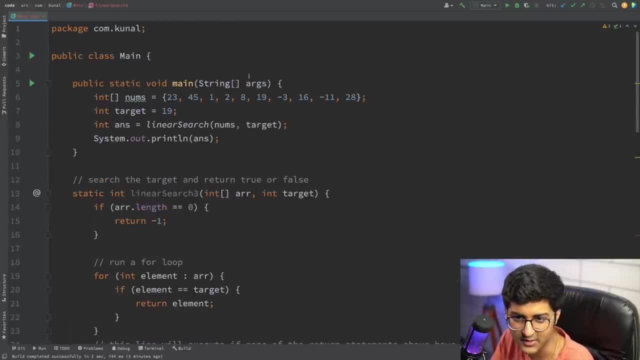 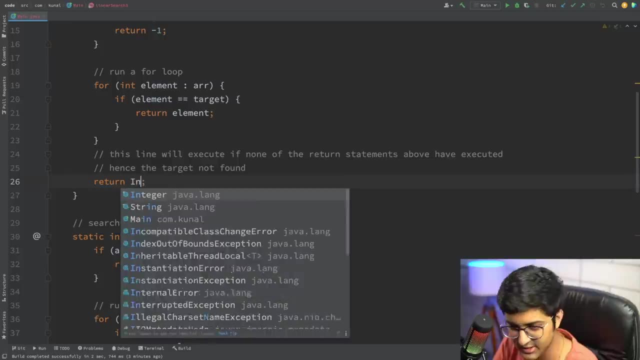 if a number does not exist and it might return minus one. so it might be possible that you know how do i know that minus one exists in this, or is it like the minus one that it does not exist? so here you can return something like integer dot uh. 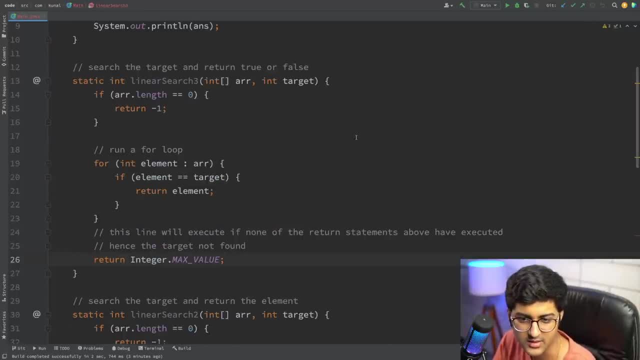 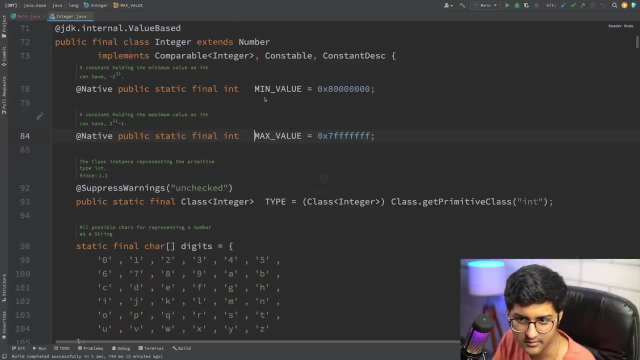 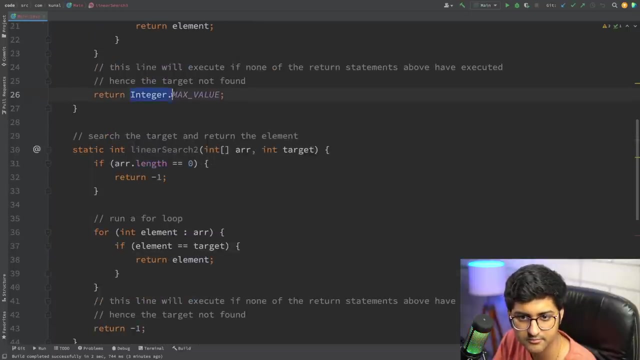 so it's just like a constant. by the way, this is another convention. constants are written in capitals. okay, other than that, we can do return the sorry. this should go over here. basically, i'm just saying return this if the item is not found, because minus one might be one of the. 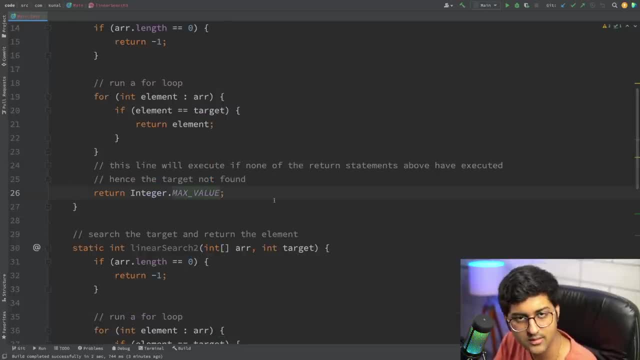 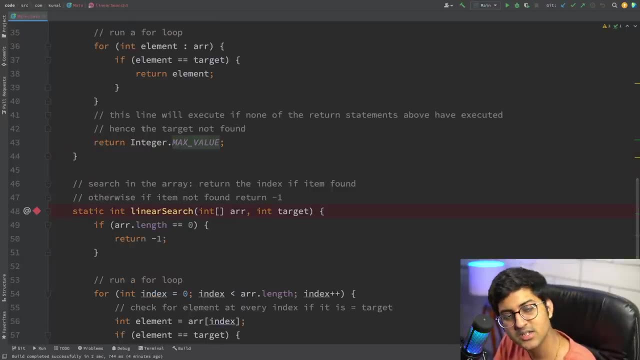 elements. okay, so here, because in where am i? why am i returning minus one over here? because i know minus 1 will never be an index. but here there is a problem: minus 1 may be the item in the array. that's why I'm returning index value like this over here, like the. 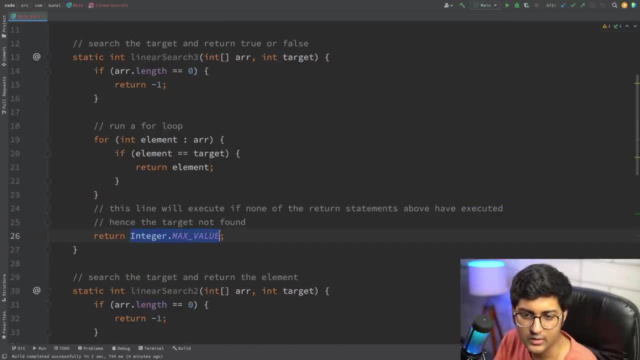 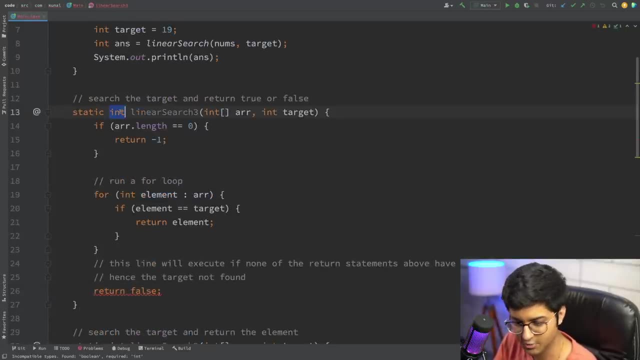 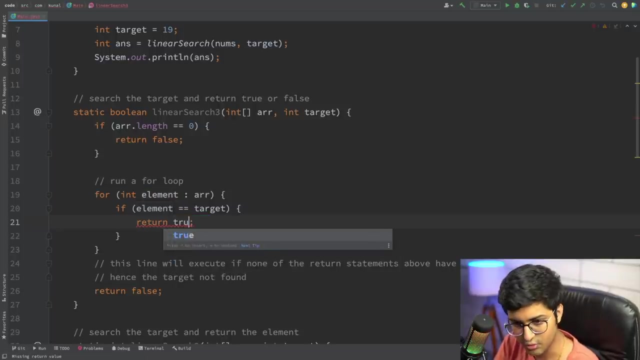 integer: the max value of the integer. here I can do something like return true or false. basically, if does not exist, return false, this will now be changed to boolean. this will be changing to return false. this will be also true. very simple stuff, okay. so we did like linear search today and now we can do. 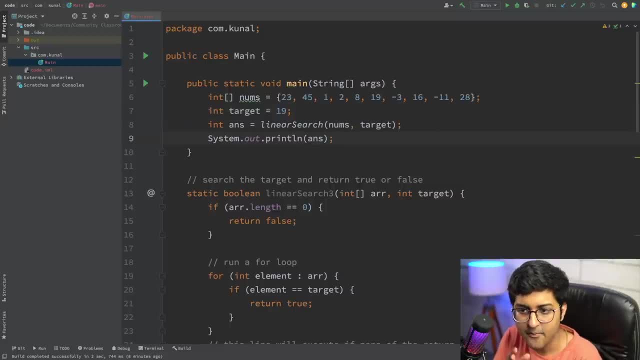 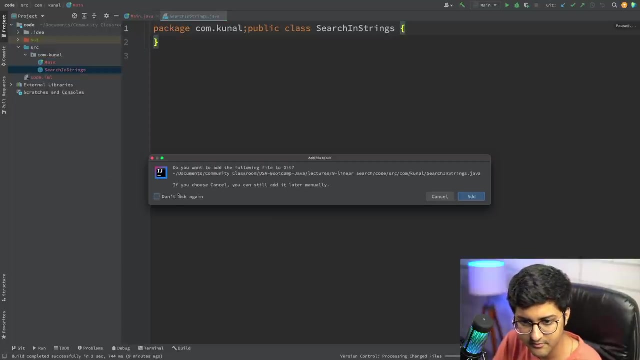 some questions. okay, so I also mentioned like the string is also like a collection, like an array, you can imagine it as like an array of characters. I can also, you know, work with strings so I can say: search in strings. okay, you, I'm not going to create a function, I'm just going to write it over here, but I 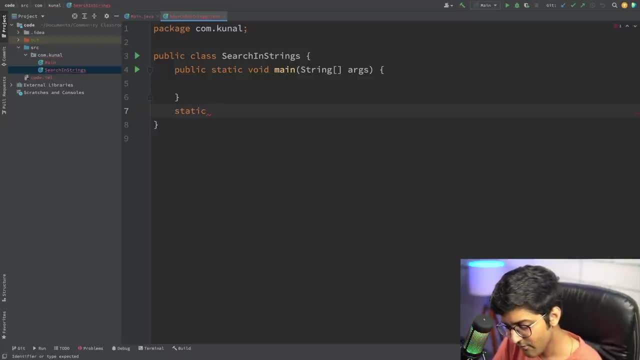 can make a function, no worries, static. I can say boolean search. pass a string over here and I need to search for, let's say, a character in a string. okay, let's say: string name is equal to Kunal character to search is equal to, let's say: 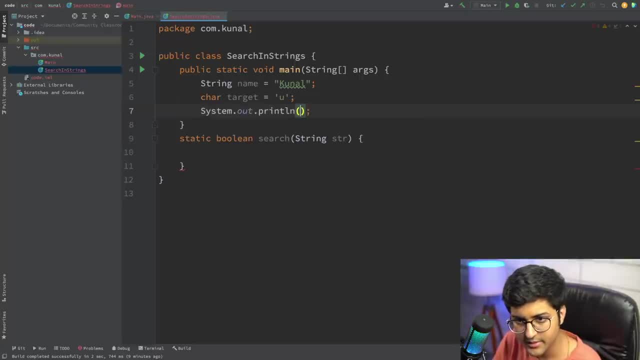 you does you exist in this string print search of search target. so I need to put a target over here as well: car target. so basically I'm just going to say if string dot length is equal to equal to 0, then I can just say return false you. 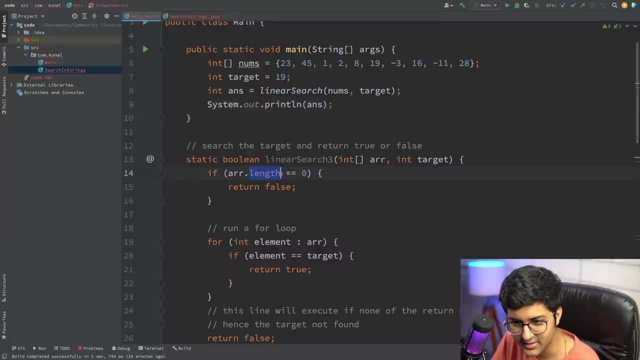 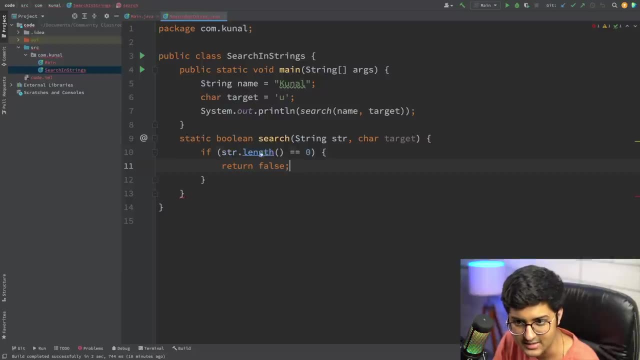 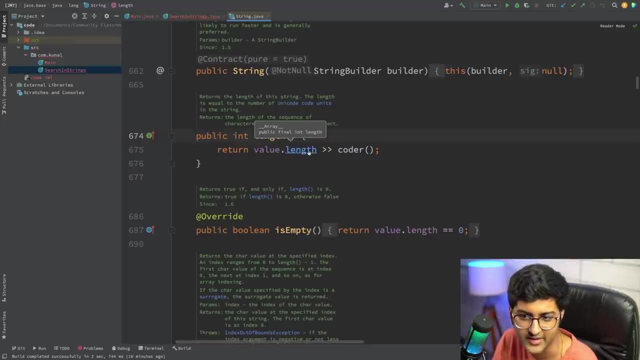 might be on asking like: hey, why is a radar dot length not having the brackets? because this is a variable, okay, and this is a function in string class function and internally it also has the value dot variable, like the value dot length, only the variable public final length, length of the type. 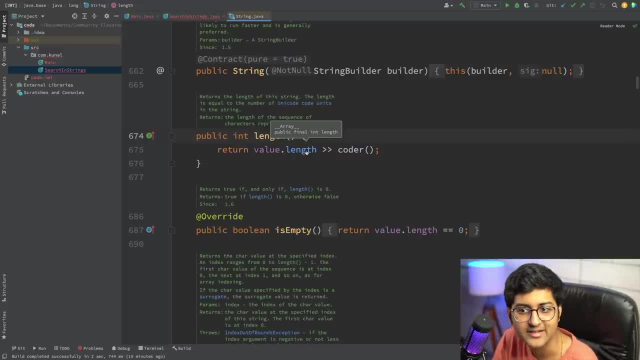 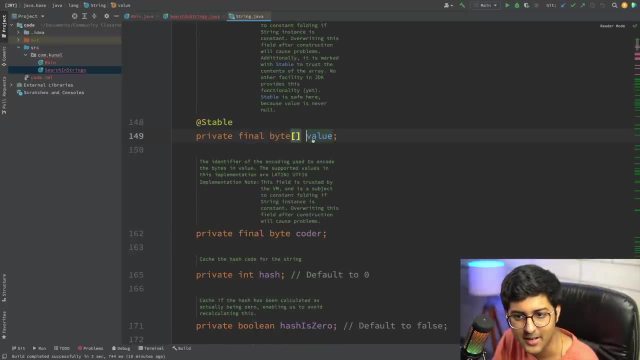 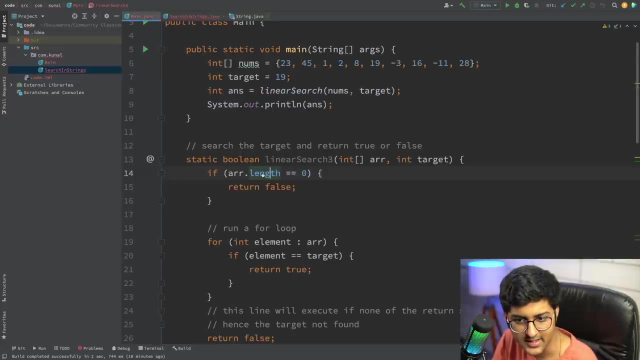 array, as you can see. so internally it's array only. internal representation is array only. okay, it's like a byte array, I believe. here and here it says that the persons and same, here it's any get all. so I'm calling a function of 0 or I'm 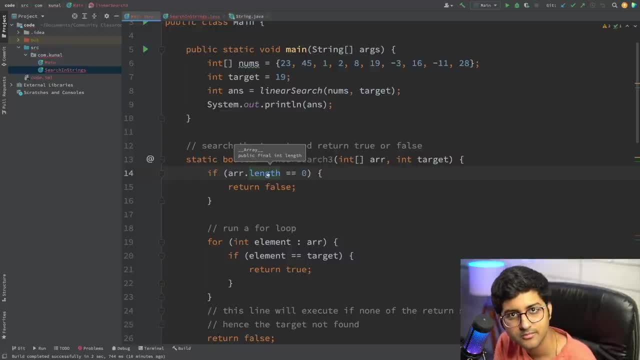 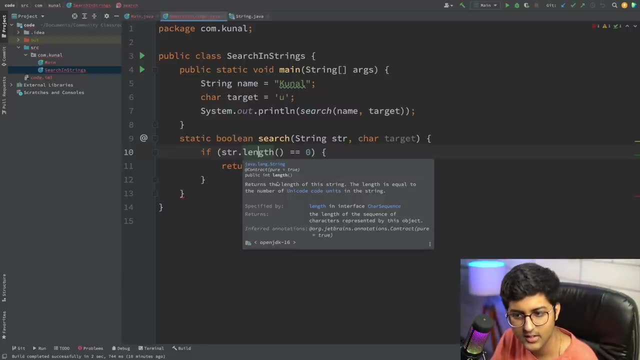 taking a, and since the porte is a variable, i'm putting 0 and this one is the instance, so that's why I'm using that from here. then I'll use electrical Pacific anyway, okay here, since it's an array. so it's definitely I seeking okay. 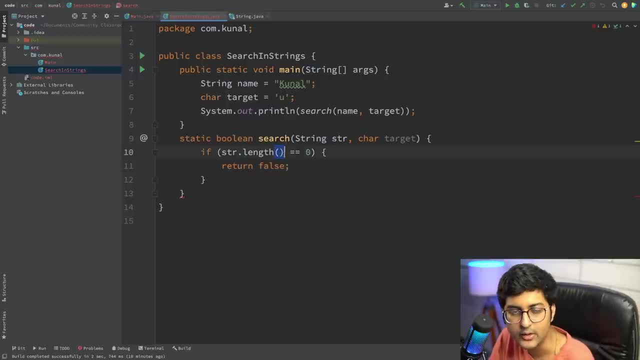 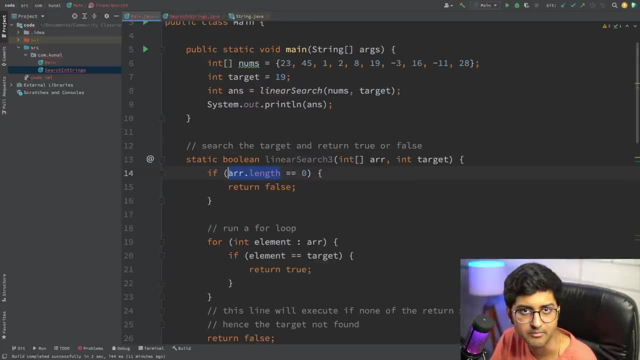 same thing: public-final int length. so, okay, this is a variable, this is a function part, a method. okay, Letry turns the length of the stream, so that's why it has calling over here. so I'm calling a function internally also, it has this same, so this: 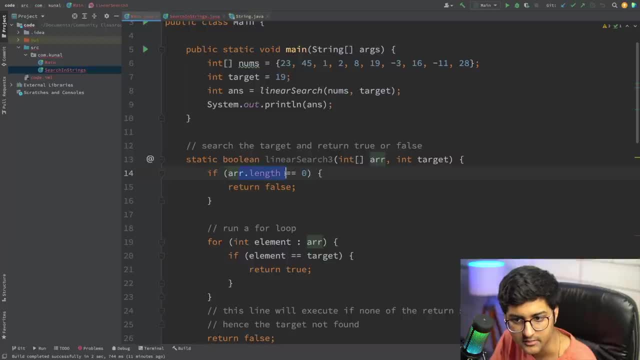 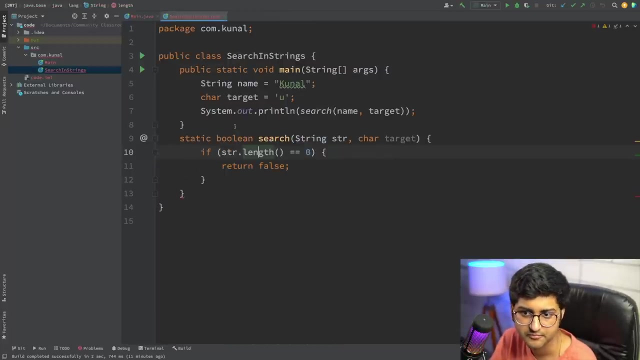 so internally also, it's calling this only this thing for its length. so it's saying the value, which is the, you know, array dot length. that is why array dot length for array data type dot length. so just a simple function, all right, so i'm just going to say for every character: 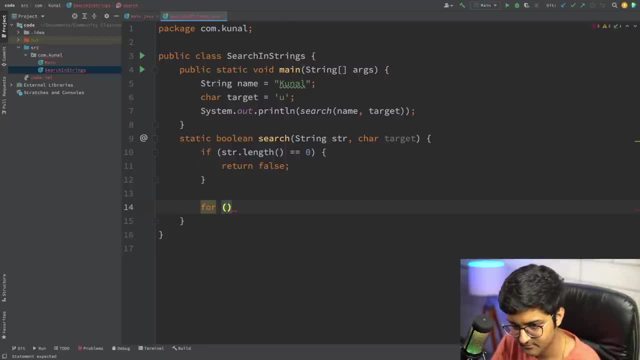 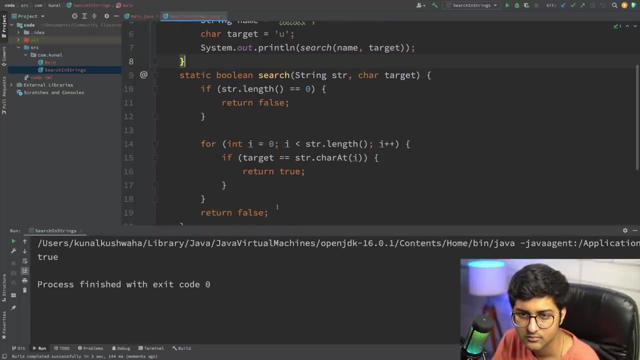 i can say for um, for i is equal to zero, i is less than string dot length, i plus plus. if target is equal to equal to string dot character at i, i'm just going to say return true, otherwise return false. give it will give me true, true. so you want to get a character at a particular index of any string? you can use the carat. 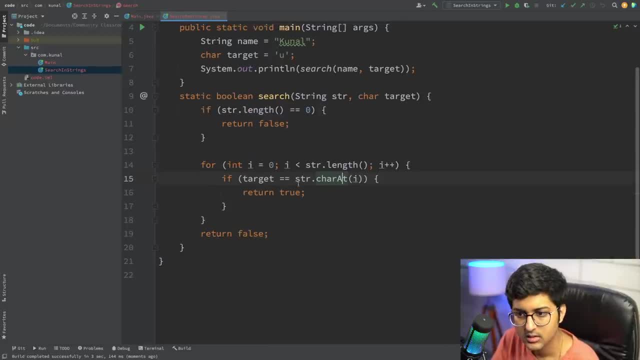 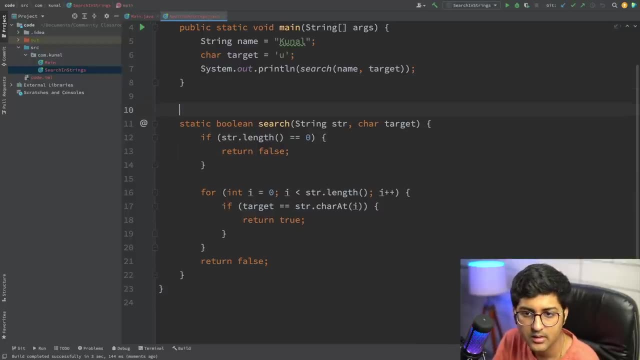 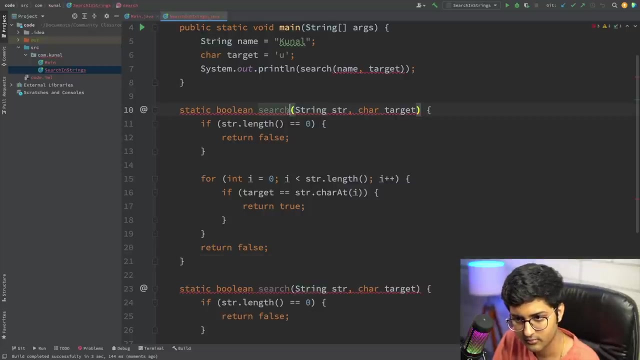 method. okay, so after this i can also do for each over here. for each basically runs on an iteration. so basically i can can say for. so i'm going to say for every character in my string: dot to carat: if ch is equal to equal to target. 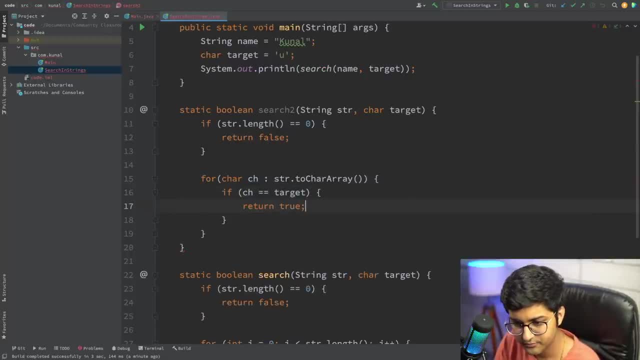 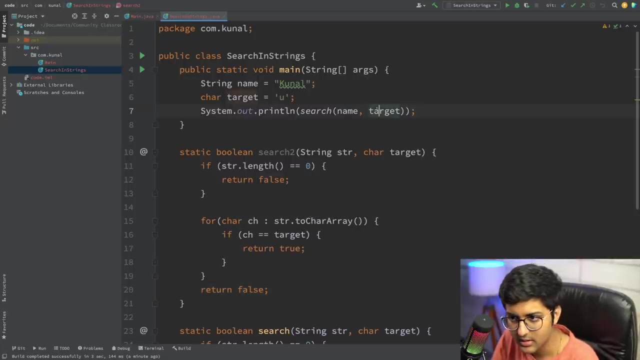 return true, return false. basically for every. for each like to use the for each loop. you need like some array or collection or something. that is why i had to just convert a string into a character at a. it's very simple. basically, this is what i did for my create new. 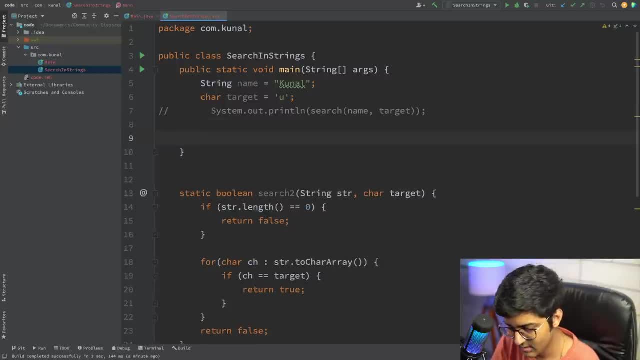 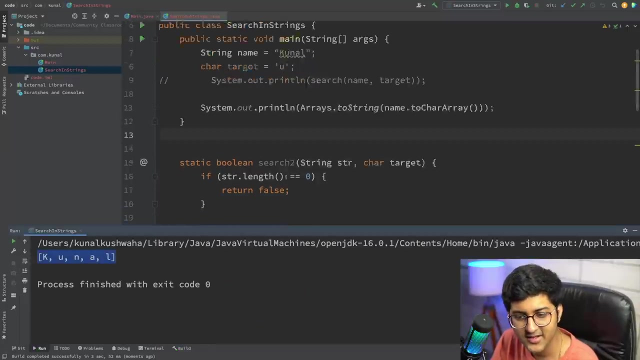 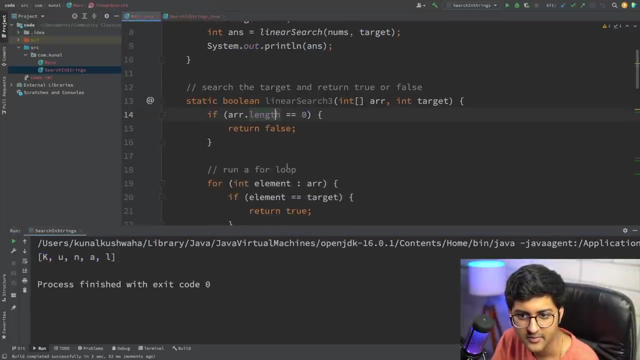 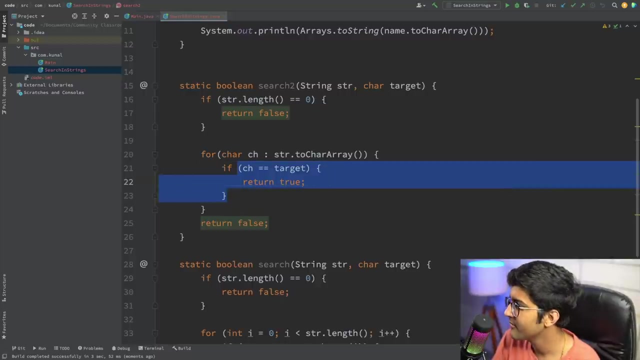 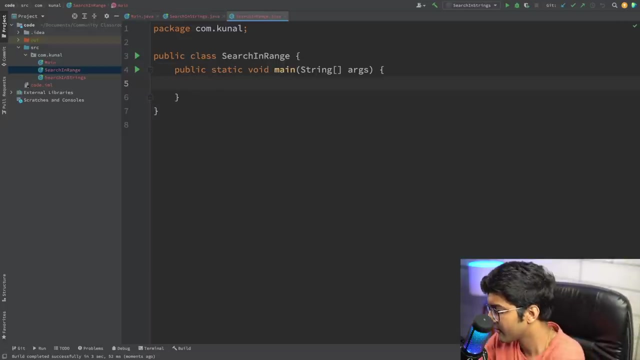 order. that's it. okay, that's it. similarly, as we were doing with this thing: for every element in the array check. for every element in the array check. all right, cool. next thing we can do is search in range. so, for example, how do we search in a particular range? for example, if you're given an array? 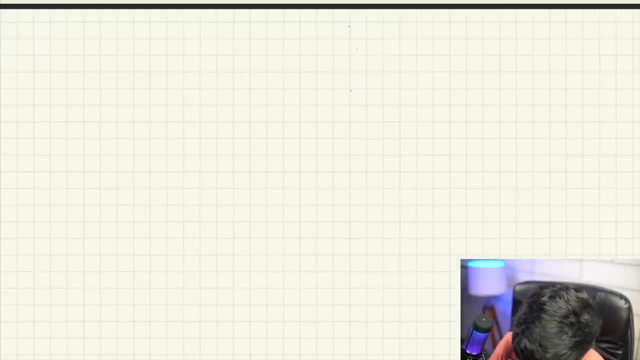 like this. you can say: like my array is equal to um. 18, 12 minus 7, 3, 14, 28, whatever. these are the index values: 0, 1, 2, 3, 4, 5. and if you are given an array like this, you can say: 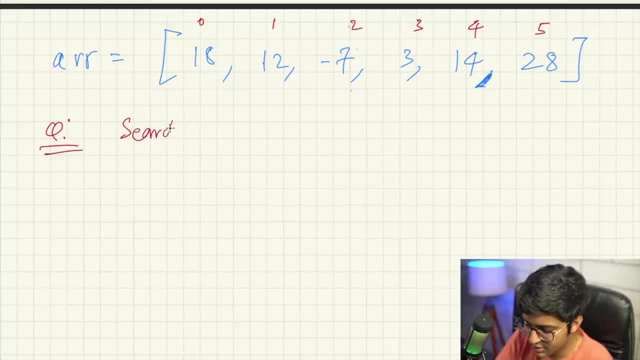 and the question is that search for 3 in the range of index um, let's say 1 till 4.. so in this only range you need to check. we are just going to do the same thing, but instead of running from 0 till the. 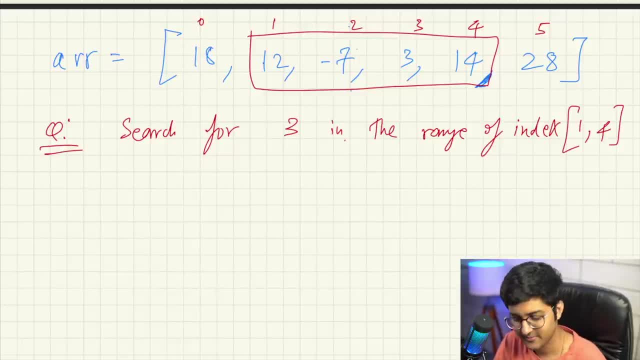 end. we are going to run from 1 till sorry, 1 till 4. yeah, start and end. that's it we are. we are doing the same thing. nothing, nothing new over here. okay, just the range is changing and in order to show you why there is, 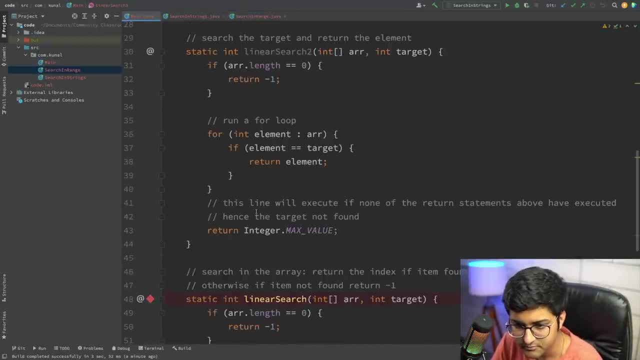 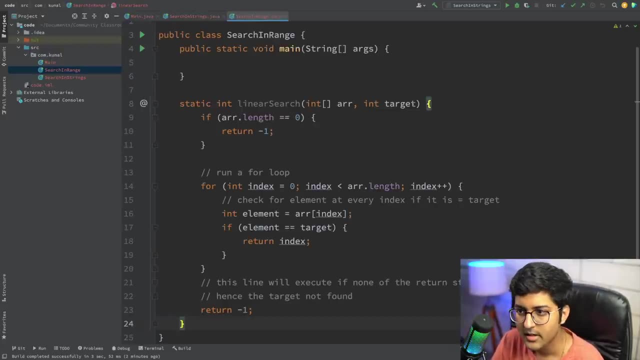 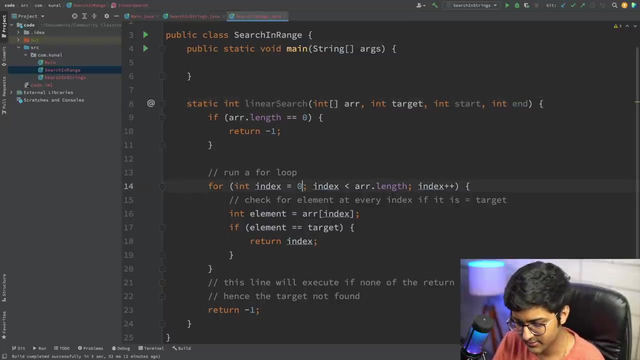 nothing new. i'm just going to copy paste the previous example. let's copy paste this here. i'm just going to take start and end, okay, and this i'm just going to replace with start, and here i'm going to say less than equal to, because i actually want to. 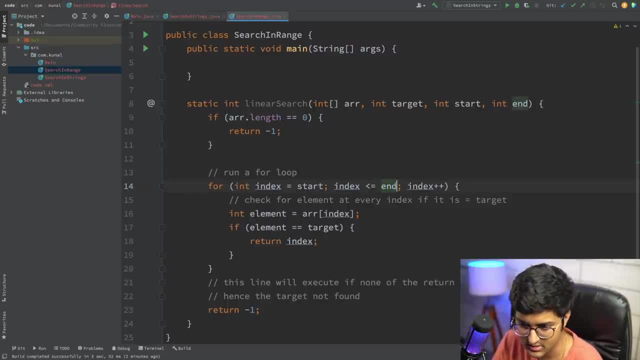 include this. i'm not taking length, i'm actually taking the index only. so this is the index, that's it. that is it, nothing new? instead of running from 0 till end, i'm just now running from start till end, like zero, to the end of the array. now. 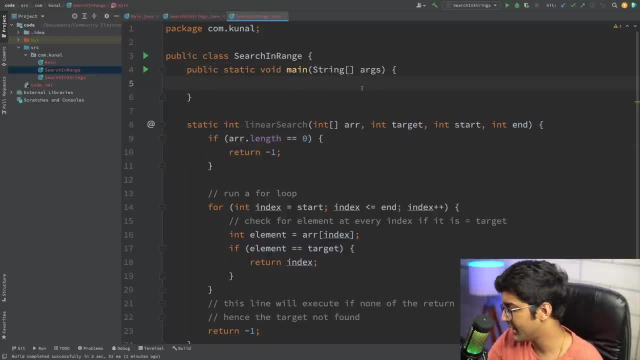 start till the end of the array. so here, basically, we had int array. in the previous example we had uh, what did we have? 18, 12. i'm looking at my ipad, the drawing minus 7, 3, 14 and 28 and i'm going to say my target is equal. 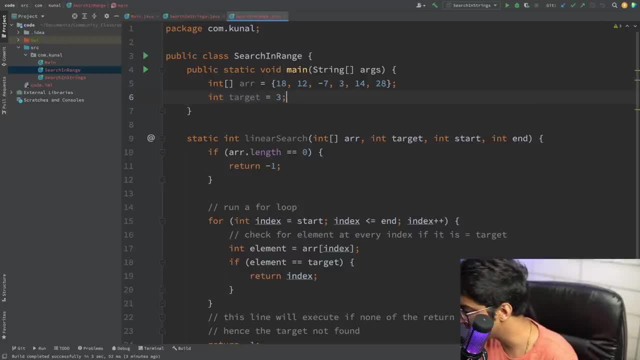 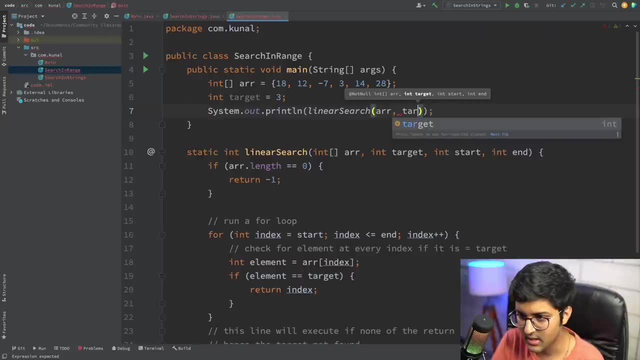 to what i was searching for: 3, and i was searching in the range of 1 till 4.. print my linear search, my array, my target, searching from 1 till 4. so this should give me i'm searching for what three, so three is at the third index, because zero, one, two, three, so it should give me three. 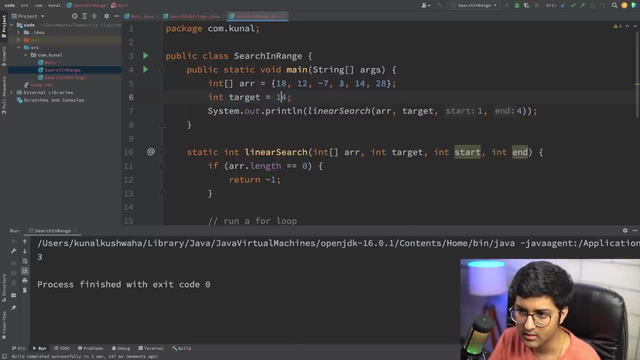 right. if i search for 14, it will give me index number four. zero one, two, three, four. yeah. if i search for something outside this range, like 18- 18 is outside the range- it will give me minus one, minus one. okay. if i search for something that does not exist, it will give me minus one, which is: 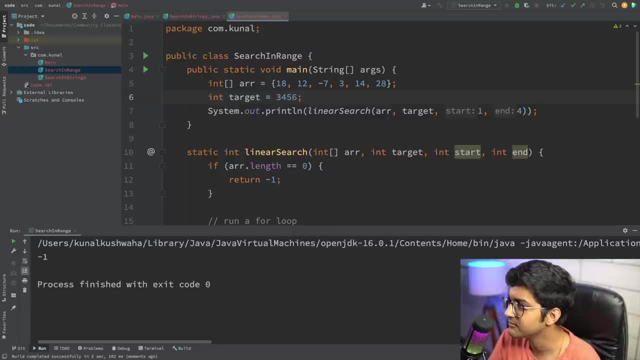 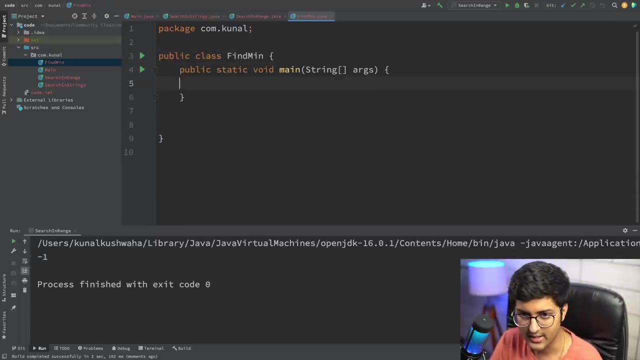 very obvious. all righty, very cool stuff. another simple example, you know another can be: find a maximum number or minimum number, so find minimum number, public static void main. so i have an array. something like this array is equal to. i'm just going to copy, copy this one. 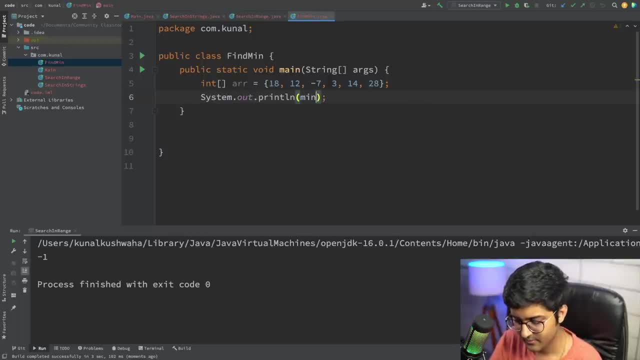 okay, and i'm just going to say print minimum of this static. i'm finding the minimum number, so i'm going to return an integer minimum number here. i just have an array. let's see how this is going to work. basically, we just want to find the minimum number in the area. so, in order to find the minimum number, how are we? 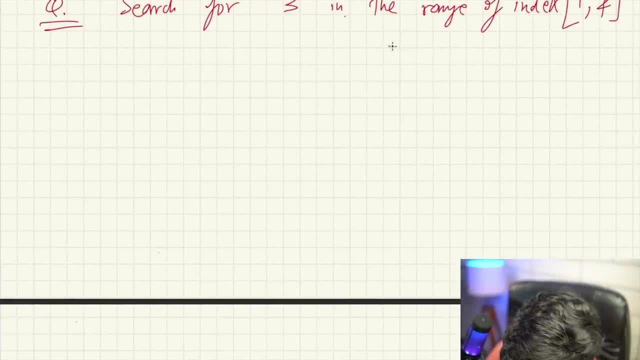 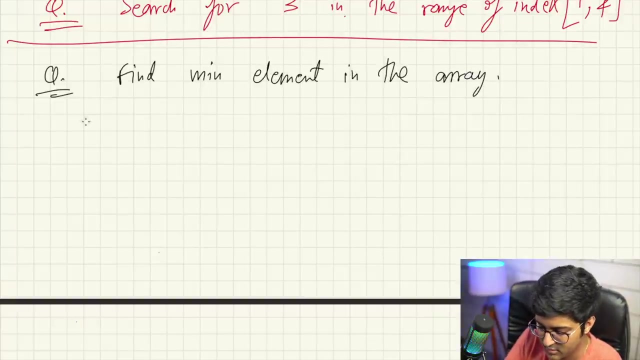 going to do this question: find minimum element in the array. so let's say arr is equal to the same, which is 18, 12. let's say minus 7, 3, 14, 28 minus 7 is the minimum one. so we are going to start the linear search. so i'm going to 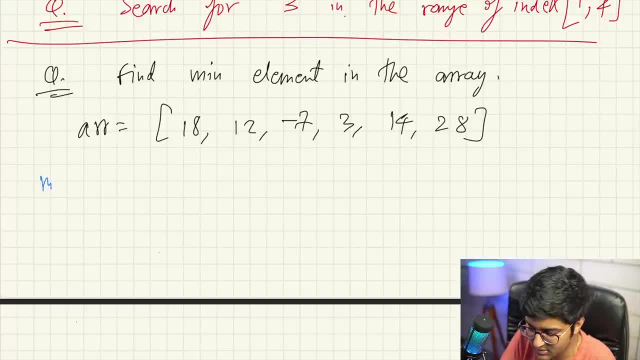 say, let's say i assume that this is minimum, the first one. so i'm going to say, let's say minimum is 15. then we start searching from here. is 12 less than 18? yes, it is update. it is minus 7 less than 12. yes, it is new. minimum is minus 7. is 3 less than minus 7? no, it's not. is 14 less than. 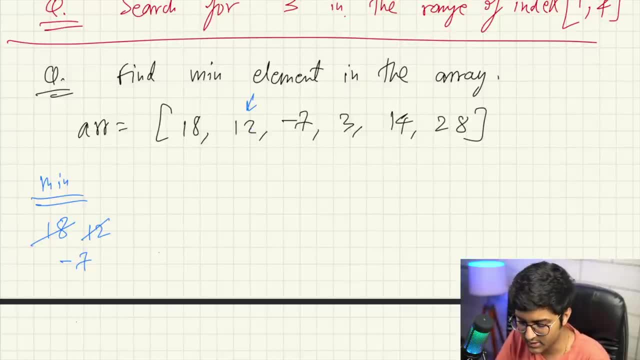 minus 7? no, it's not. is 28 less than minus 7? no, it's not. answer: is minus 7 in the end? very simple, nothing. nothing is going on over here. similarly you can do maximum. similarly you can do minimum and maximum in between the ranges. 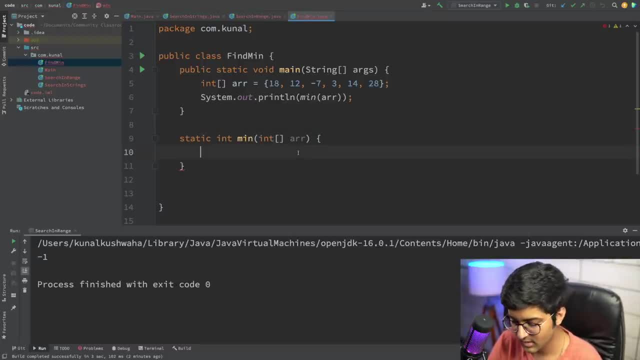 okay, i'm just going to show you the very simple one. so i can say: you know, um, if i can say, assume arr dot length is not equal to zero, so assume this is not an empty array, so i can say my answer is equal to the zeroth index. and then i'm going to say, starting from, 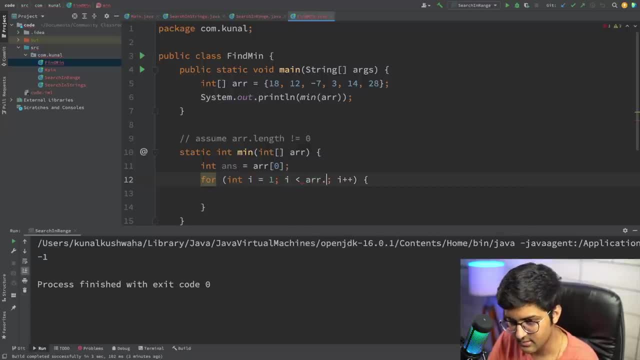 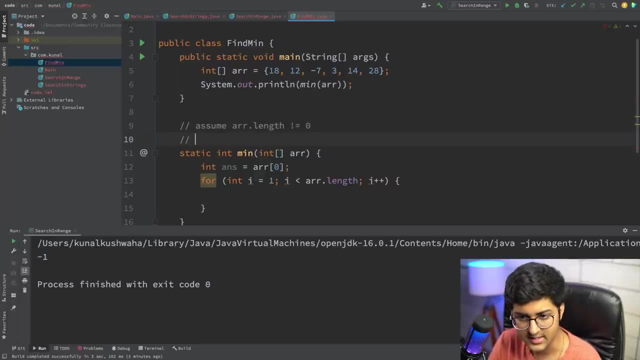 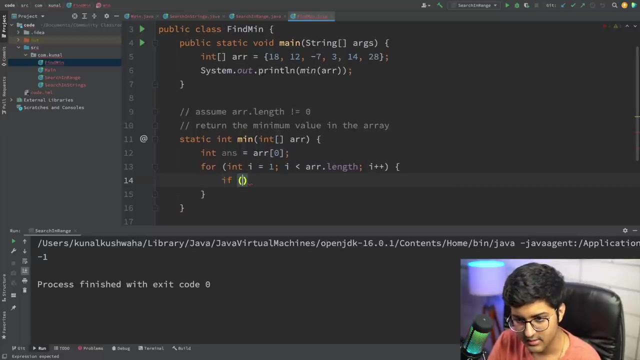 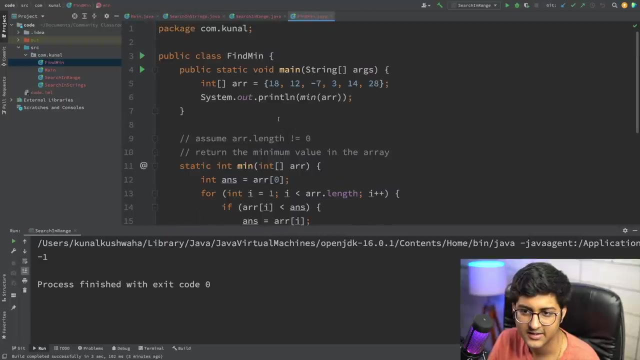 the index number one less than the array dot length. i'm going to say here basically, let's say, return the mini minimum value in the array. so i'm just going to say if the current value is actually less than my overall answer, then update the answer in the end. just return the answer. that is it. this is going to print minus 7. 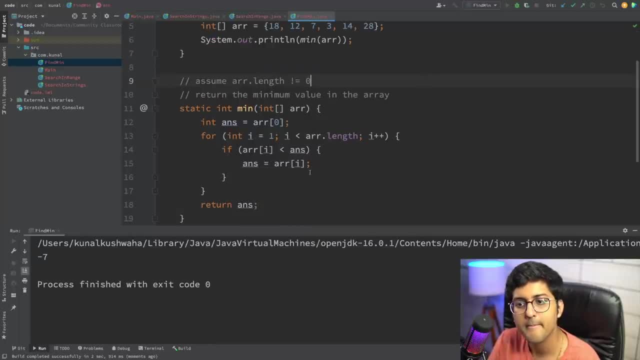 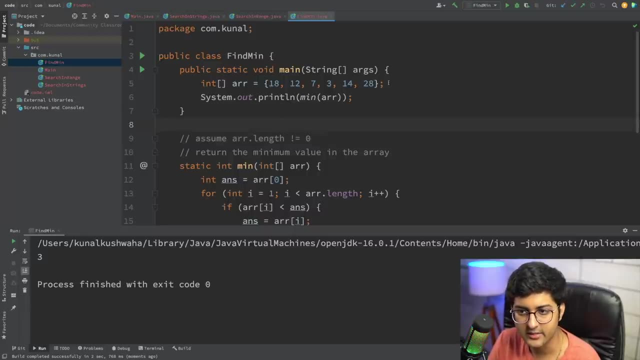 if i convert this to 7- now the minimum value is 3- it will print 3. now let me update the answer. something very simple stuff: just checking each and every element and taking one answer as, like the, my main answer. i will keep updating that answer whenever i find. 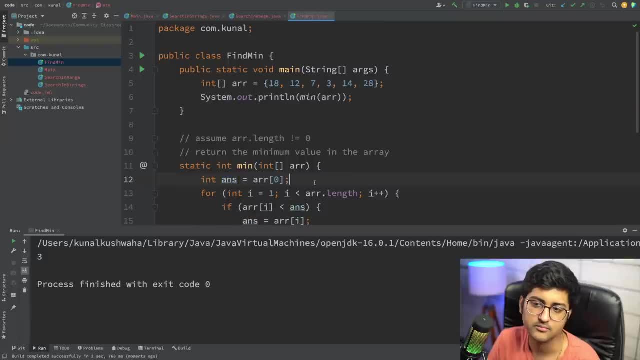 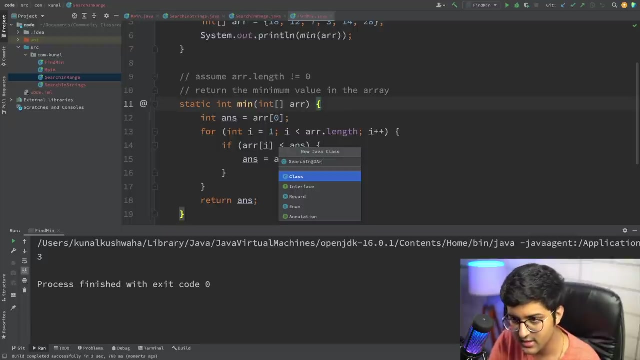 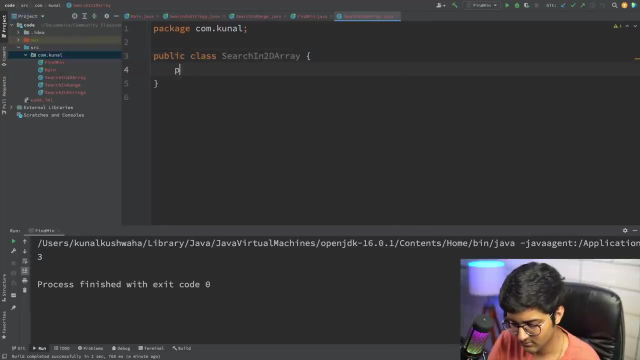 a new answer that is smaller than the previous answer. at the end i will have the minimum answer, okay, so that is pretty much about it. let's say we can also search in a 2d array array. okay, let's say, I create a 2d array like this. I create something like we. 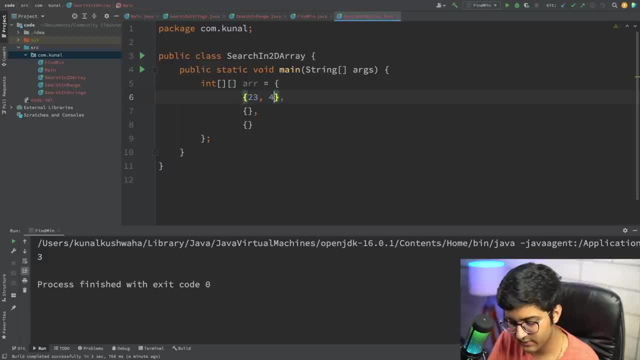 already covered 2d arrays in the previous lectures: 23, 4, 1, 18, 12, 3. 9 then is 78, 99, 34, 36 or whatever take. let's see one more: 18, 12, 18 is 2 times no. 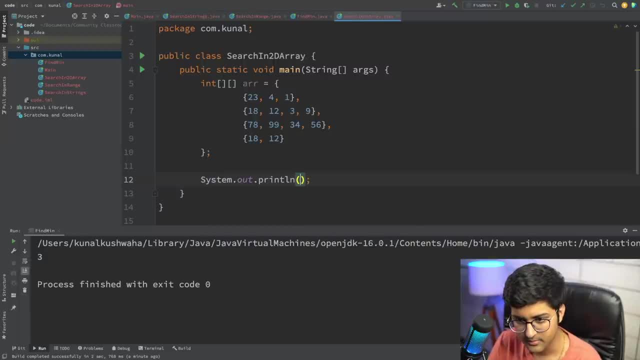 worries, does not matter. I'm going to say print answer, not answer. I can say search in the array for my target element. let's say I want to search for what do I want to search for? 34, I can search for 34. I'm just going to create search over here. static return. 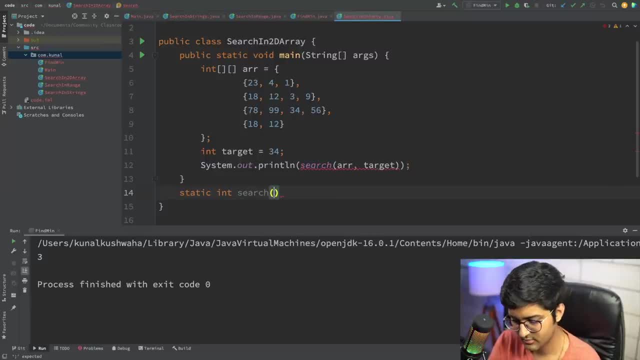 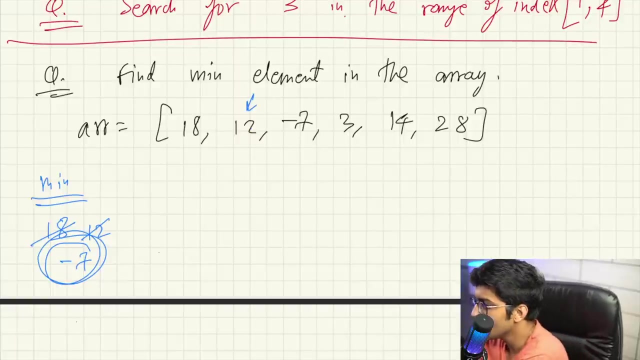 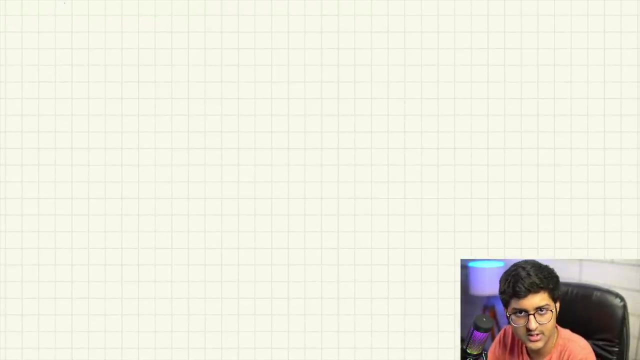 the integer search, 2d array and target. so how do we search for in a 2d array? let's look into that as well. this is very, very simple. we have already learned how to iterate over the 2d arrays in the previous lectures, so we already learned that- how to like iterate over. 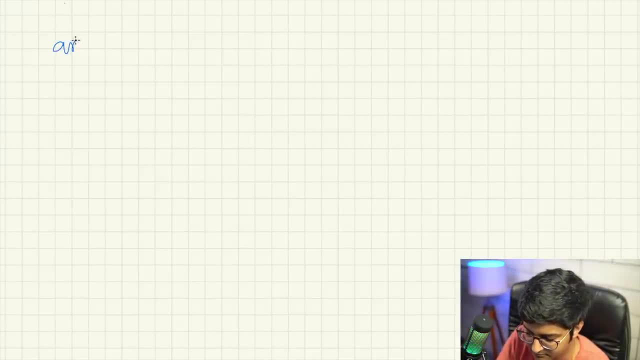 the arrays. so let's say, your array is something like: so your array is something like this: let's say it's one, two, three, nine, eighteen, five and six, seven, fourteen. let's say it's something like this: so basically, you're just going to start, for row is equal to zero, row is: 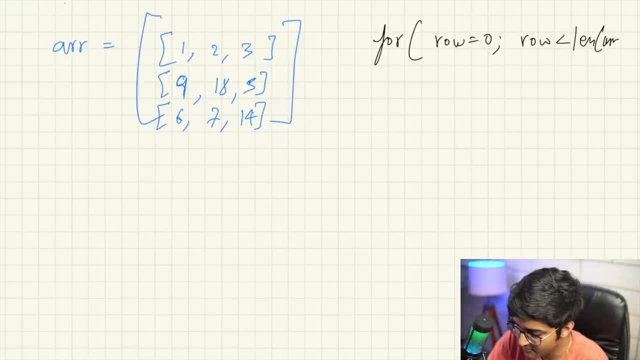 less than length of the array and row plus plus. we have already done this in detail. now, for every, column is equal to zero and column is less than the length of that row and column plus plus. if the array of row and column is equal to my target, I have found the answer. that is it very. 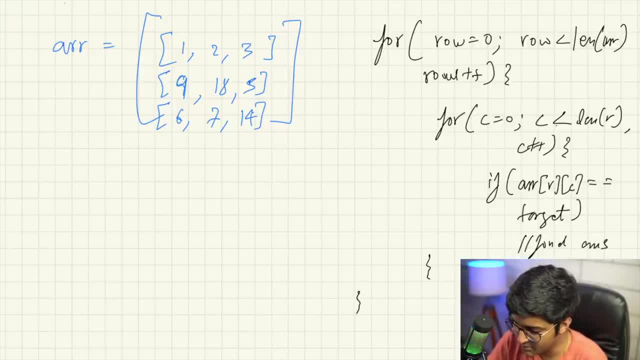 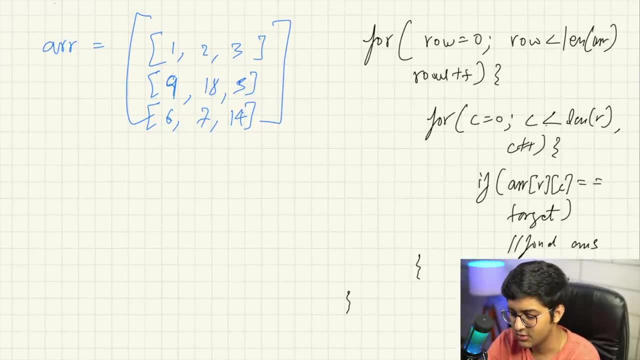 simple stuff, and if, after running this for loop, you have not found your answer, it means that you can just then return. you know, minus one or whatever. so if you want to learn more about how this thing is working internally, so for this, the outside loop is for the row, inside is for the column. I'm not skipping anything. 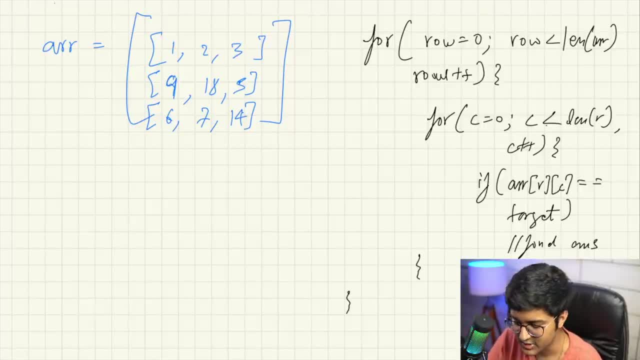 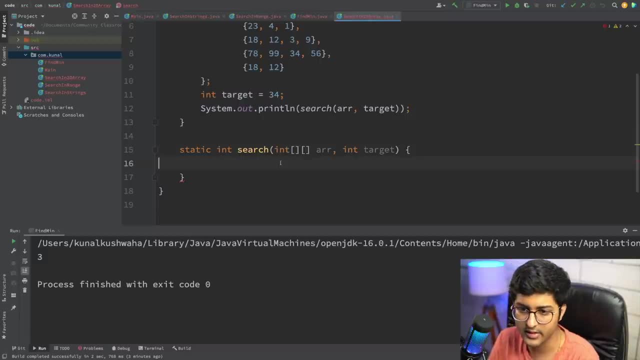 we have already covered this in detail in the arrays lecture, so check out the arrays lecture. the link is in the description. everything we have covered, like the entire iteration part, and everything we have covered in detail. so I'm just going to say, for every row, zero array dot length. for every column, zero till a. 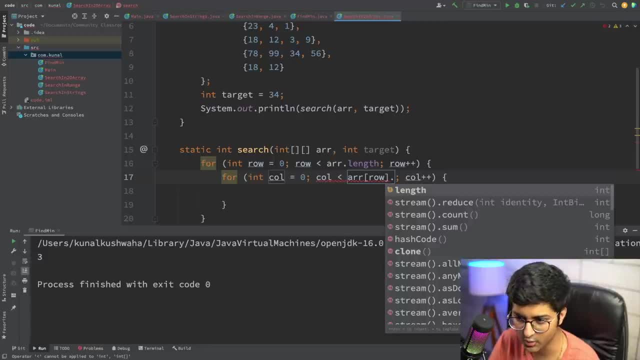 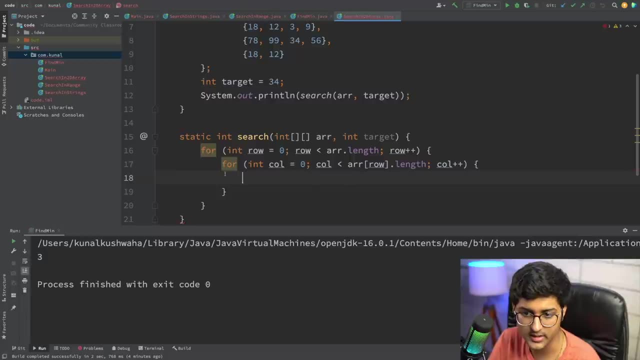 array of row. so this itself is going to be a row. uh, this itself is going to be an array. we have also seen in the lectures, in the description below, how these 2d arrays work internally and why internally, and why this is entirely a new array and you know another, simple, like it's an array. 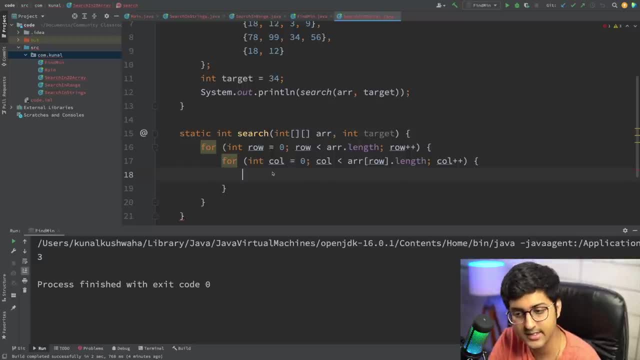 of arrays. basically, you can say: a 2d array is an array of array. we have covered this in detail. so i can say: if the row, so this basically itself, will give me a single array which is like the individual array at every row, since this is an array, i can take every column by column, column. 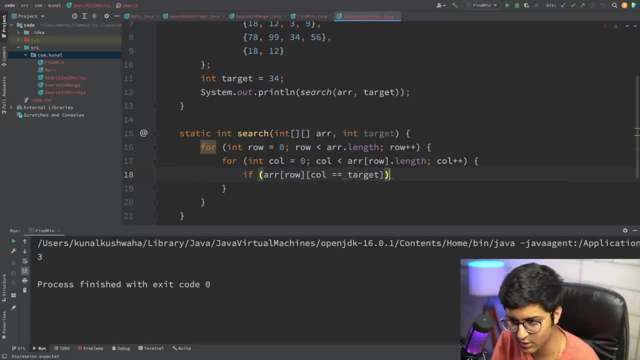 by column of this. so nothing new. we have covered this traversal already. so here i just can say: return my. now here the thing is, what am i going to return? i'm going to return the uh. i can return another array which contains row, comma, uh, column. okay, that is what i can do. 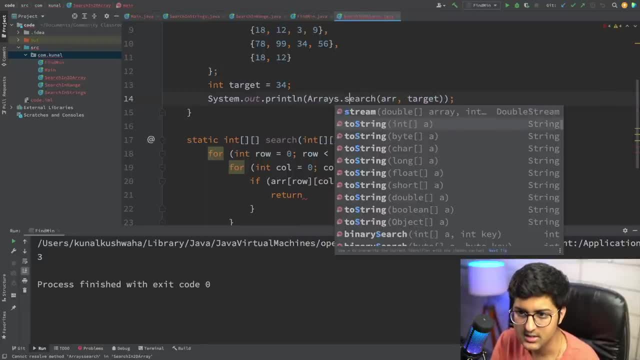 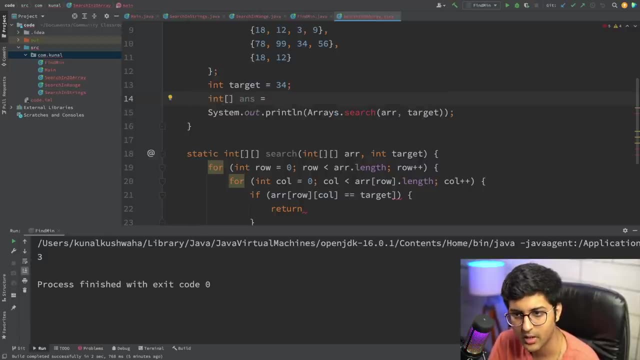 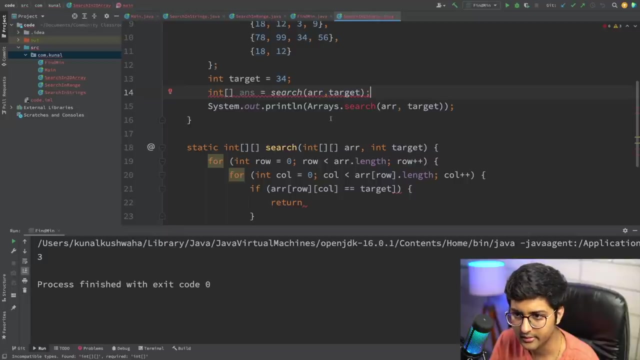 so here i can say arrays, my answer. i can just say over here my answer is going to be equal to um, what search for array n target? that is going to be my answer. and uh, here as here i'm just going to say that, uh, it's actually going to return just one array. so basically the format is going to be: 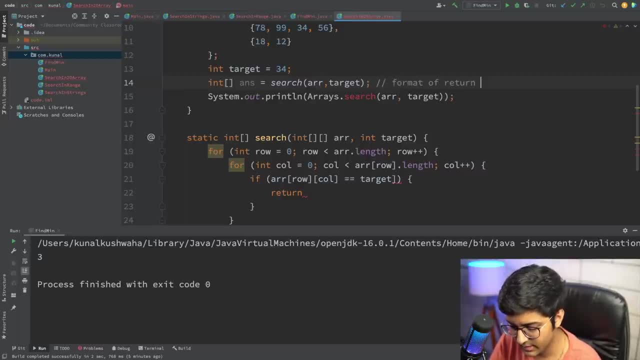 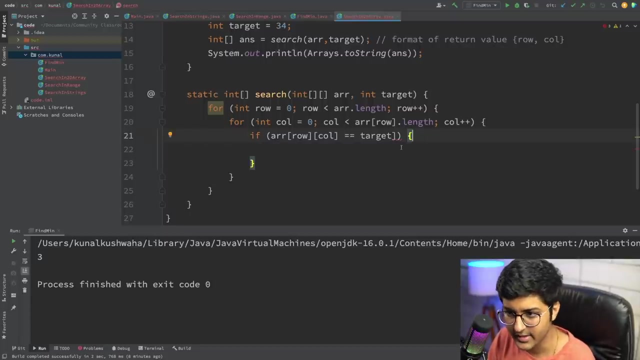 something like this format of return value, assimilating to my somewhat long name, i'm just going to say the end of an row, komen colon, inside an array which contains the start index and the end. Sorry not to start the row and column. okay, this is the thing here. i'm just going to say arrays dot. two-string answer. that is something einzel погнаćй fill colon. 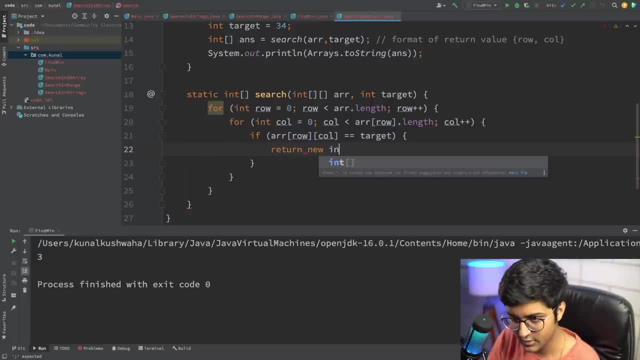 okay. so i'm just going to return an array or from a column. so i'm just going to say rIT on a new integer array and i can just at the value for growke my column. so i'm just going to say return a new integer array and i can just add the value for growke my column and i can just add this remarks here, and then i'm just going to say color DNS, oh vous. 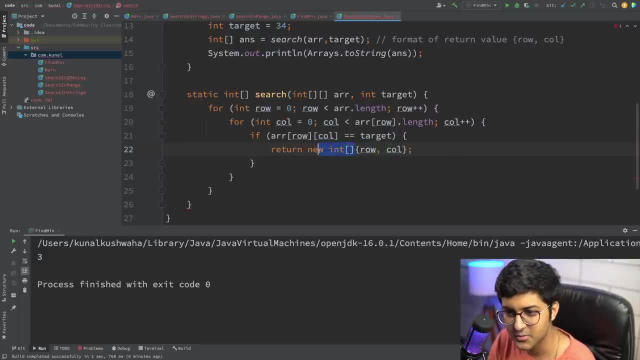 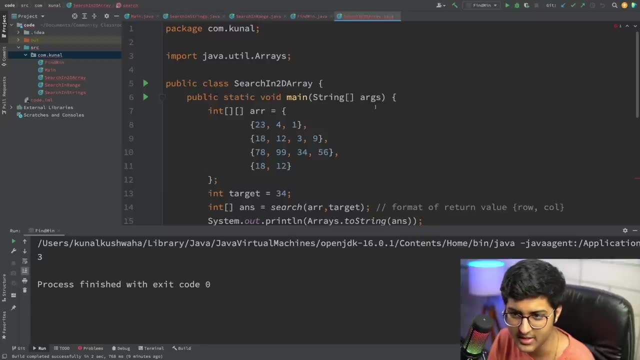 row and column. so notice something you might be like: hey, kunal, why are you not writing this? why do you have to create a new object? because the array is not initialized over here. now you might be asking: hey, why did you not add like new int, like this, like this over here? well, you can. 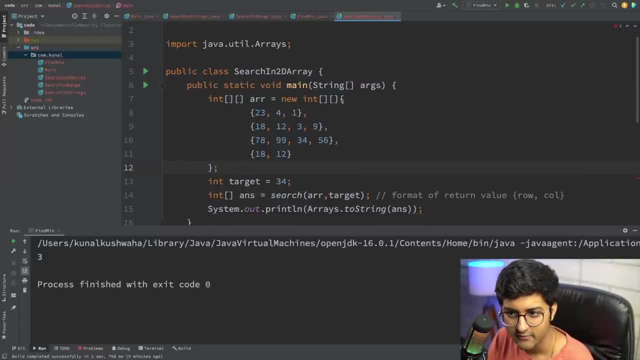 but it's like not mandatory over here. okay, when you know that it is of type array, when you're actually like assigning it like this, in that case it automatically knows that. okay, you are creating a new array and you're, you know, like uh, and you declare it like this, and when you initialize it, 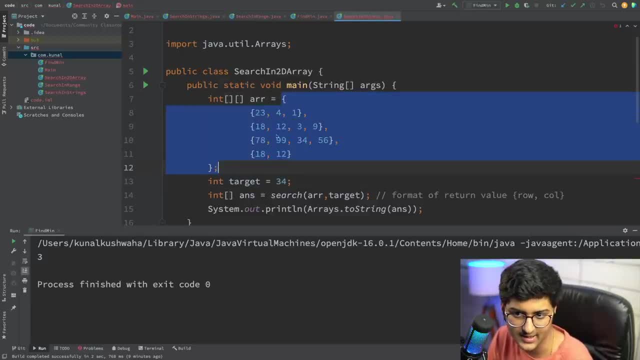 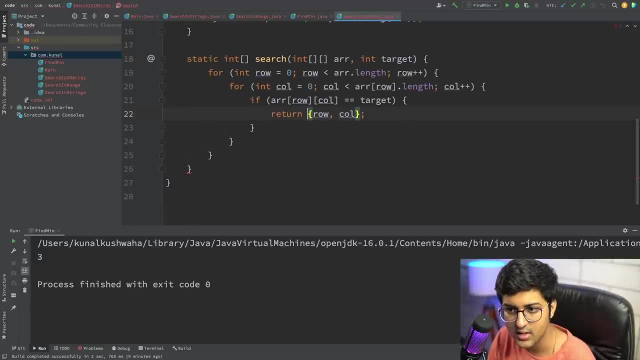 like this: uh, it already. it already knows that you're initializing an array to a like, uh, you know of a of an array type, but here it does not know that if you just do something like this, you say, okay, you're initializing this array, but where is it declared? is it declared anywhere? no, so in 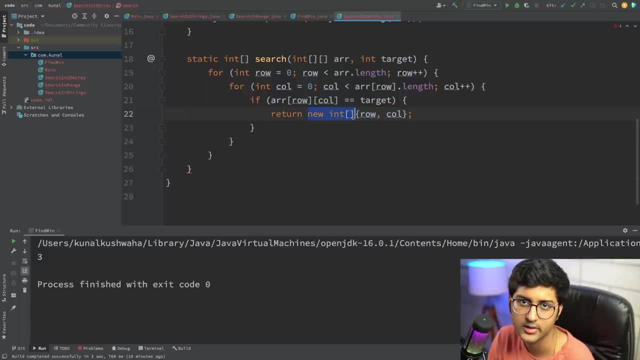 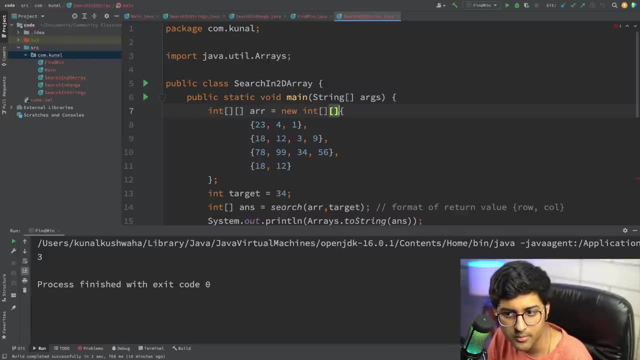 order to create an object. you can just create an object like the using a new keyword. how that makes sense. that. why are we, why is it okay to you know you not not put this line over here? and why why do we have to put over here? because over here we do not. 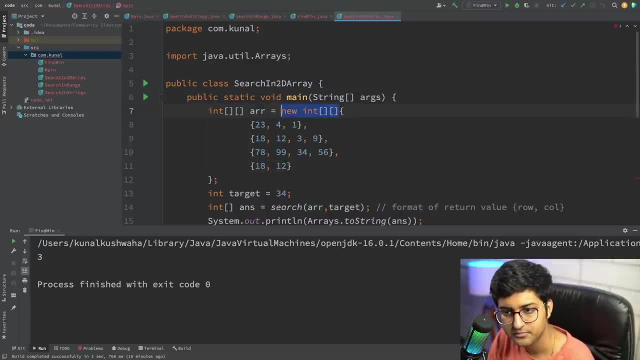 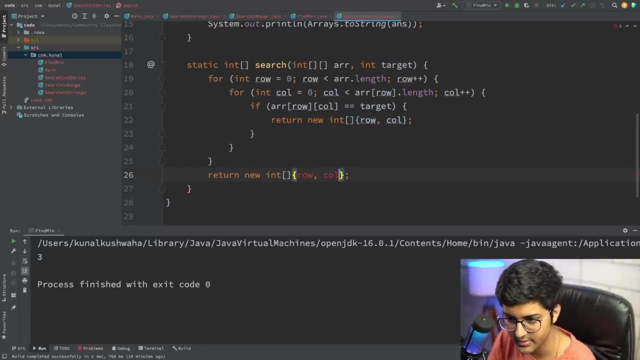 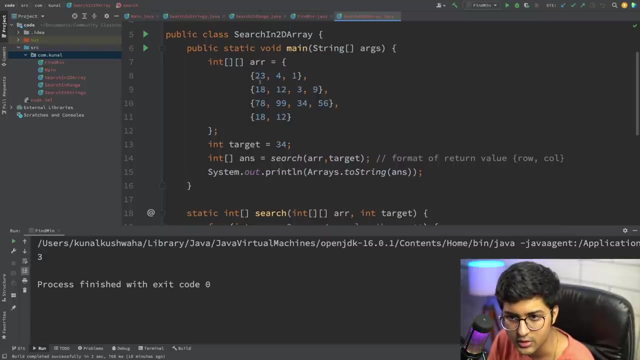 have this thing. okay, cool. so this you can put or ignore, totally up to you. otherwise, if it is not able to find it, i'm just going to return: minus one comma, minus one, that's it. so let's say you want to search for 34, so 0, 1, 0, 1, 2. so 2 is the row and 0: 1. 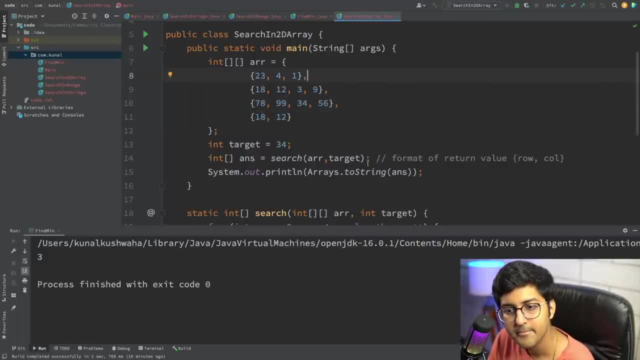 2. 2 comma 2 is the answer. 2 comma 2 is the answer. 2 comma 2. let's say, i try to search for 56, so 2 comma 3 will be the answer. second row means the row of index number two, zero one, two and column of index number three, one. 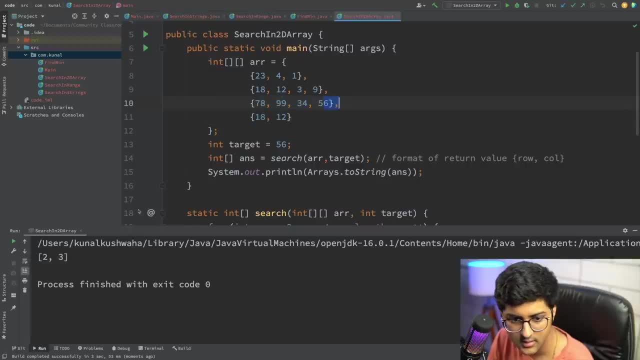 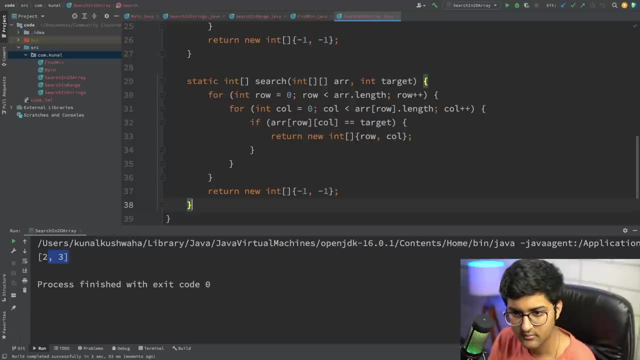 one zero, zero one, two, three, two comma three. okay, similarly you can find maximum in 2d array. you can say maximum item in 2d array. that will be returned as an integer. so i can just say: int max is equal to array of 0 comma 0, let's say the initial one. or you can do something like this: 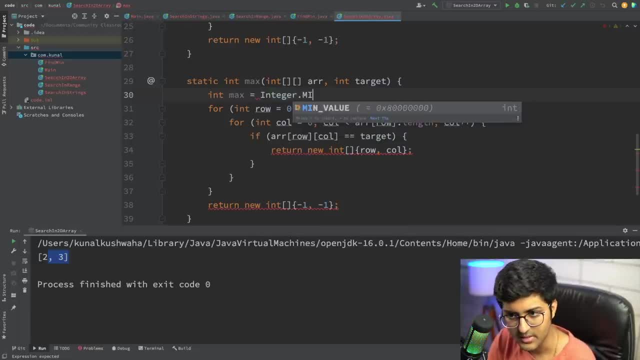 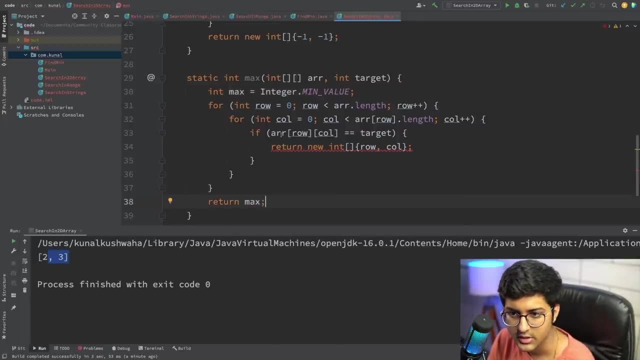 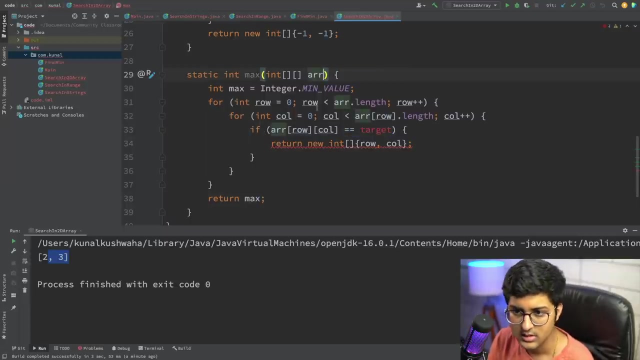 you can say: integer dot min value initially. then you can just say: return the maximum value. so here you can say: if this is actually, i don't need target over here now, so i can say: if the element is actually greater than the maximum value, then the maximum value is equal to this. 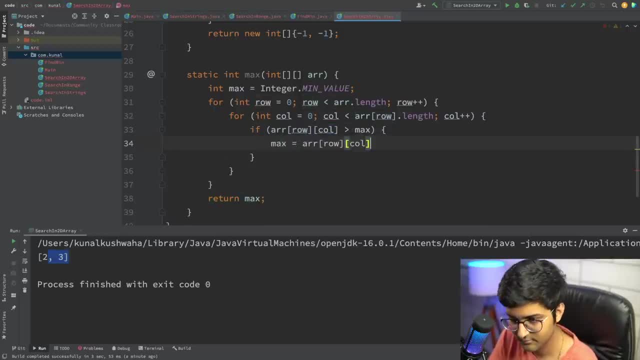 in the end just return the maximum value. you can also convert it into an enhanced for loop. we know every single array is going to be an integer array itself and in that integer array, every single array, it's going to have a particular element. i can refactor this. 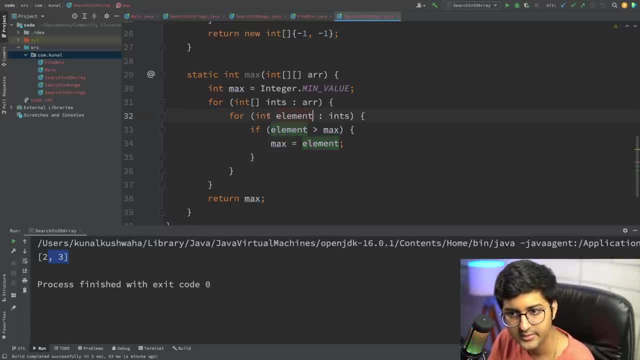 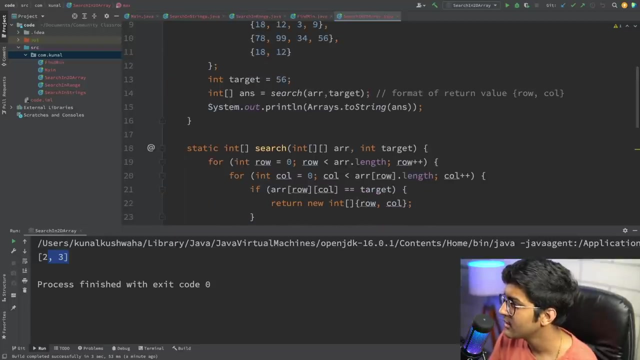 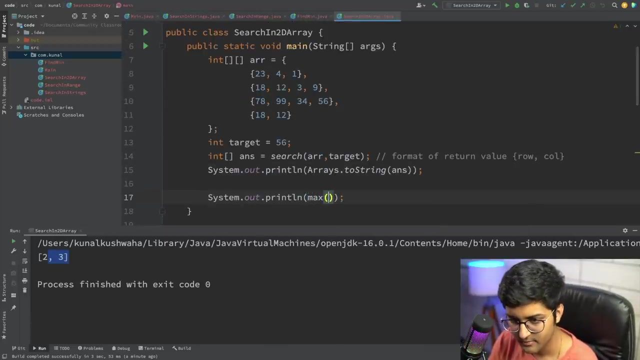 we can say element. okay, so very simple stuff and i think that is pretty much about it. cool, so you are also finding the maximum in an array, in a 2d array. but try to run this print maximum in the 2d array. so my, my array will go over here. it should print 99. 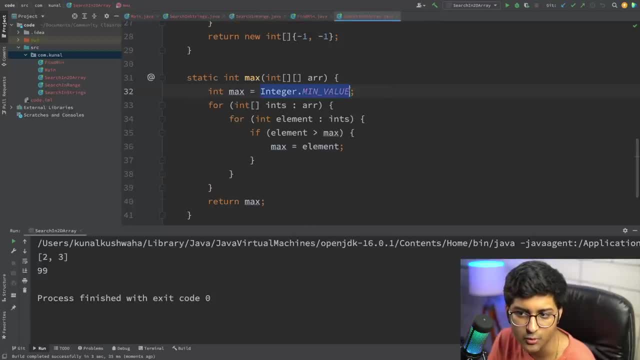 99. don't worry about this thing. what is integer dot? min value? Anil, it's just a minimum value that the integer can hold, which is equal to this, so that is why i am taking this: any item that is going to be greater than the max. 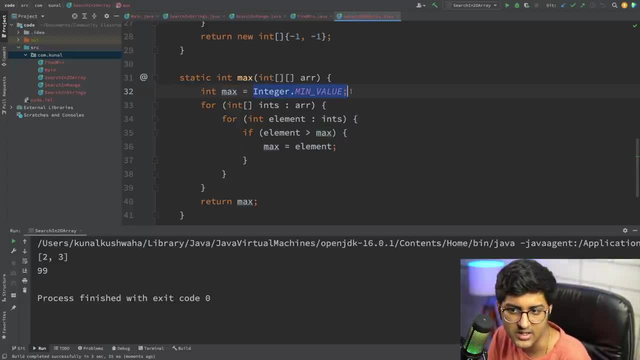 minimum that our maximum value that we currently have. that is going to be greater than we currently have. why i'm initially, you know, might some, might some people might take, like you know, infinity minus infinity or whatever. i'm taking the uh minimum value. so it's going to be like hey, um. 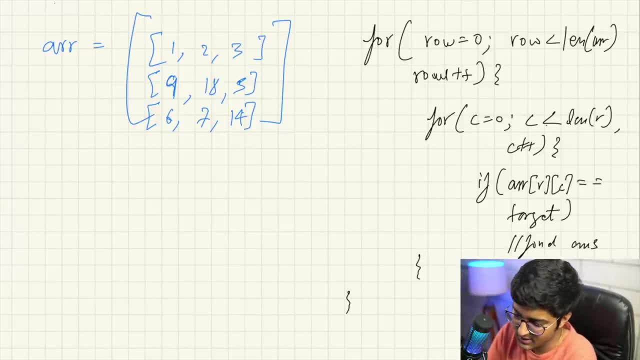 same thing, like we did over here. so for initially, the minimum value will be something like this: so it's going to have the minimum value as something you can also print- what is the minimum value? so i try to print it. so integer is a class and it contains a minimum value. 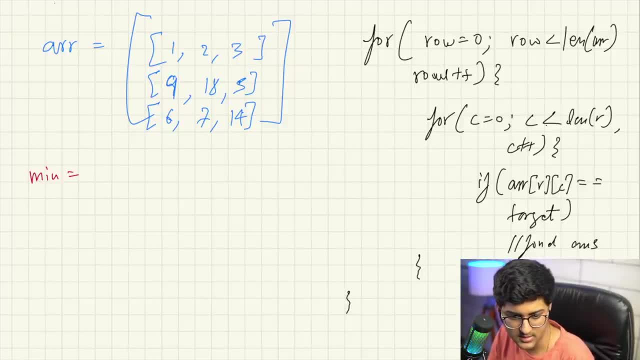 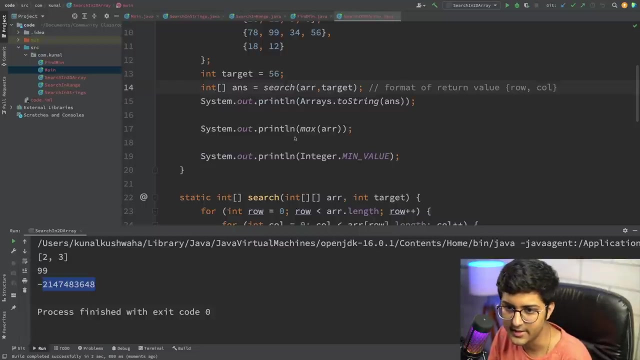 which is equal to minus this thing two, one, four, seven, eight, so on and so forth. so minimum value, let's say my answer initially- is equal to: oh, i see, you were not able to see it because i was on my ipad. this is what i did, i just said print. integer minimum value value. so minimum value that an integer can hold in java is this. and if you want to learn more about, how do we find this, kunal, how do you, how does this java know that this is the, you know, minimum value? this is known as ranges of integers and all the data types. so range of integer, float, double all. 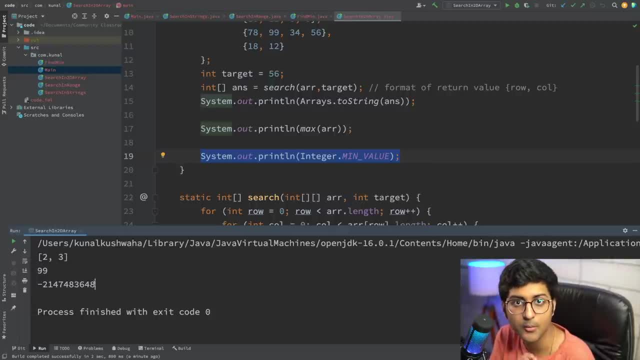 these things we will be covering in detail when we will be learning about binary numbers, range of byte, you know so bits and everything converting from one number system to another. we will go this through this in detail. how this is coming, we will learn in detail. we will actually. 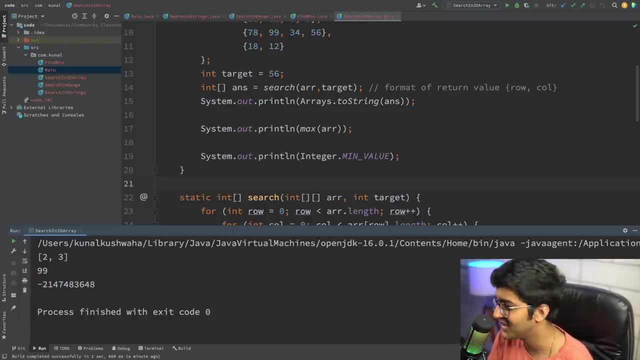 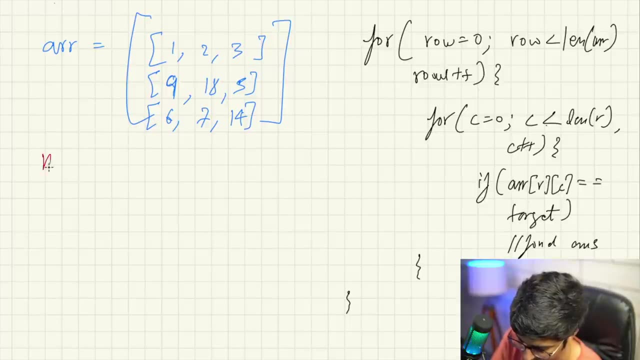 derive it. we will actually learn the formula for this. so make sure you like share and subscribe. okay, so here, basically, the idea is that my answer, my answer, like the, my max value, initially it's equal to minus two, one, four, seven, four, eight, three, six, four, eight. then it's going to check. 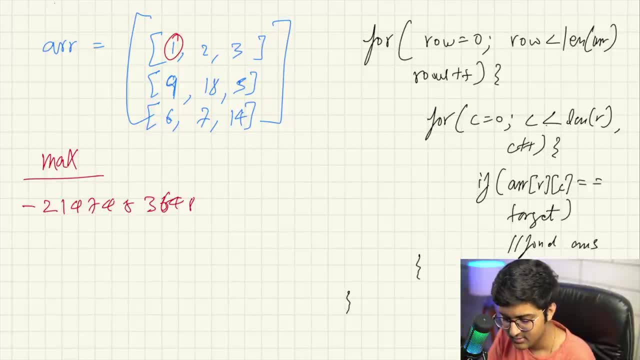 okay for this thing, is this greater than this? it's going to be like, yeah, duh, obviously it is, because this is a minimum minimum value. so now, our maximum value so far is one, and it's going to check for two. is two is greater than one? yes, it is. it's three greater than one? yes, it is. so, is three greater than two? yes, it is is nine. 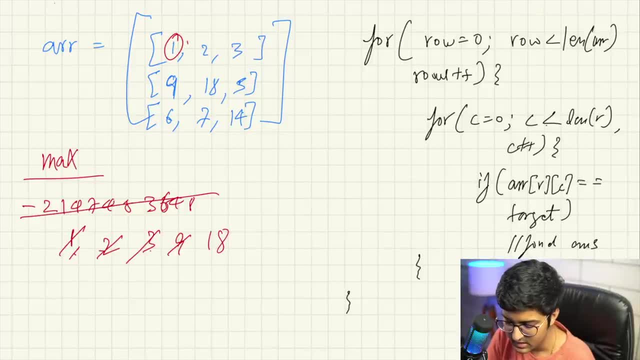 greater than the three? yes, it is. is 18 greater than nine? yes, it is. it's five greater than eighteen? no, it's not. a six greater than 18? no, it's not. is seven greater than 18? no, it's not. it's 14 greater than 18? no, it's not. answer: is 18, okay. so even though in the previous examples we have 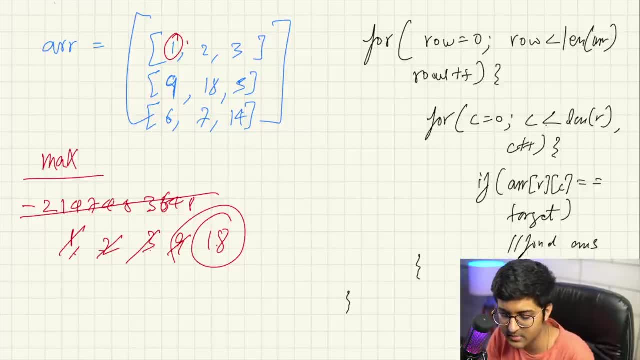 done something like: hey, let's assume the first element is the maximum one. you can also use this approach. you can take if you're finding the maximum element, you can take integer dot min value if it has the first answer and if you're taking the minimum value, you can. 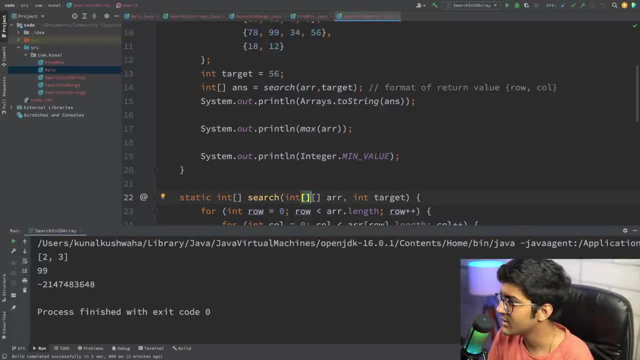 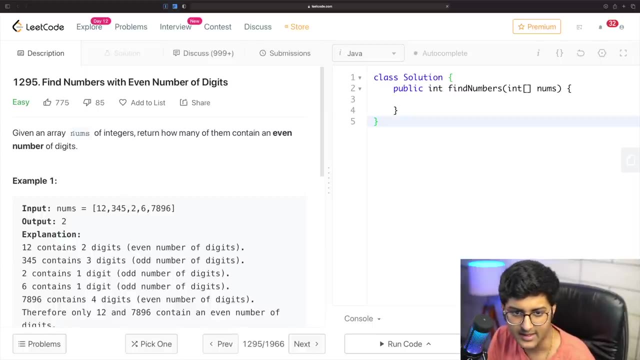 take integer dot max value. okay, so that was about finding uh, minimum and maximum values. okay, so let's do this question. so basically, in this question you are given an, a, an array of numbers of like integers and you have to return how many of the of those numbers contain even number of. 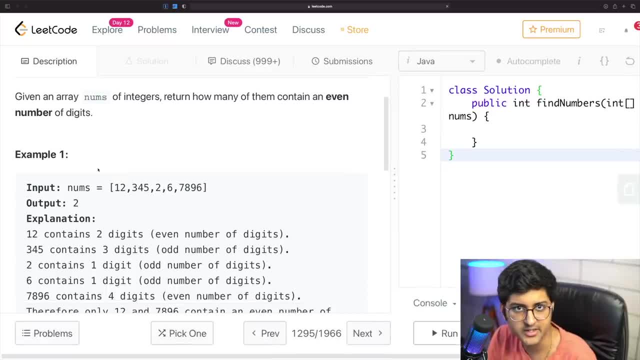 digits. so here example 12. 12 contains how many digits? two digits, one and two. so two is even number, so this is one number that contains even number of digits. 345 contains three digits, so three is odd number, so that's why we won't take it. two contains only one digit. six contains only. 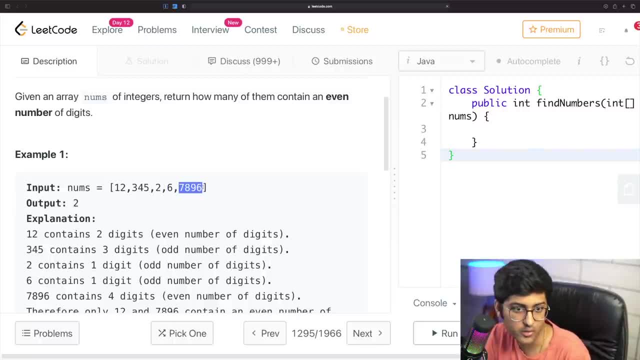 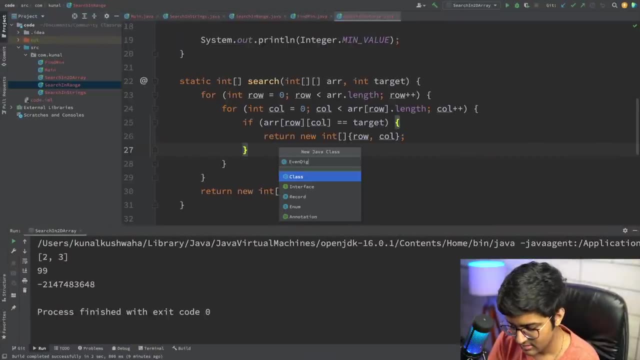 one digit. seven, eight nine six contain four digits. four is an even number, so only 12 and seven eight nine six contain even number of digits. how are we going to solve this? let's look into it. so basically we can do something like even digits question- public static. void me just copy this thing over. 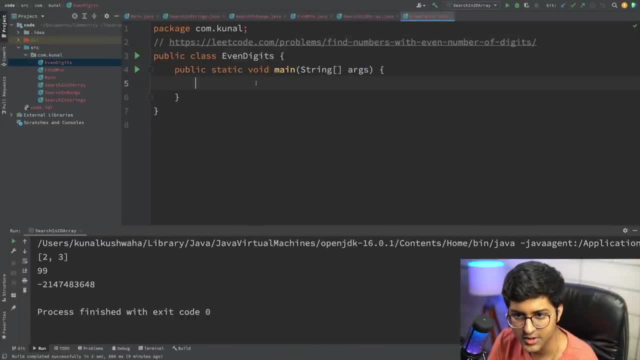 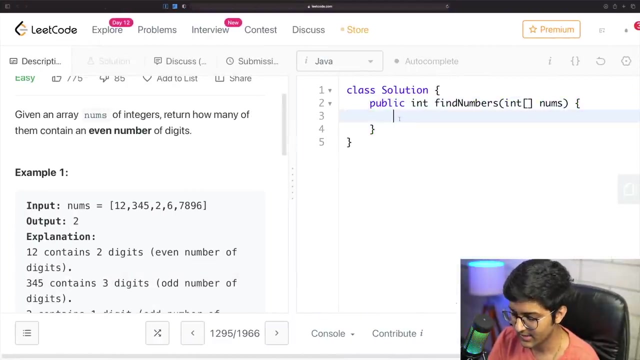 here. so this is the question. so maybe i can make something like um answer. so this is static or they have already. might be they might have already given something like this: i can directly code over here, no worries. but no worries, i can. i can code over here, no worries. so i can code over here, no worries. 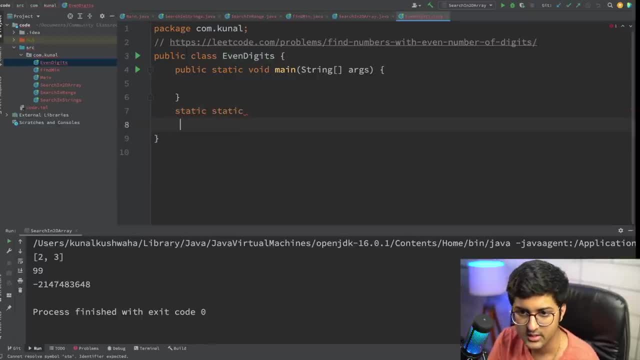 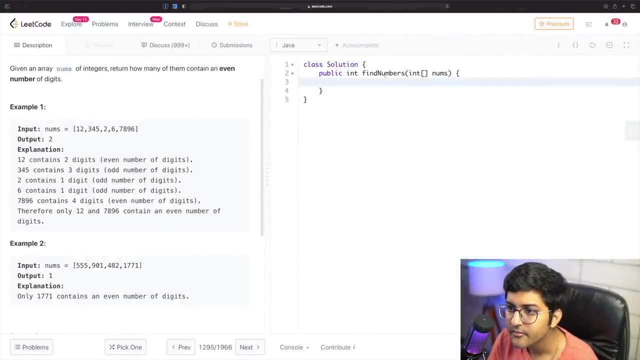 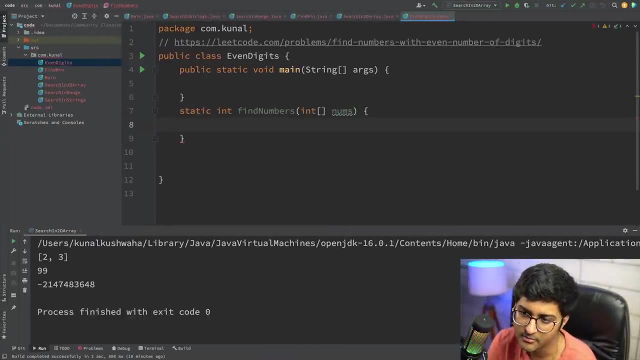 and create my own static- oops, public start static. and it's saying: return an integer, find numbers in num. so i'm just going to copy this, okay, and here i'm just going to say that. let's say i'm just going to iterate over the array, so i'm just going to say int, answer or count. 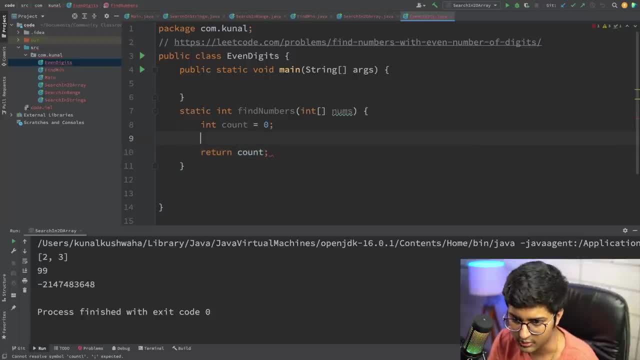 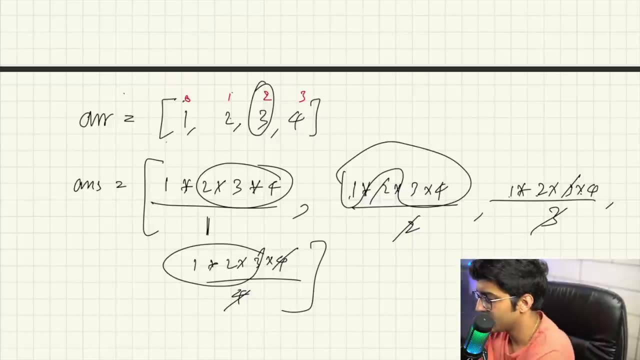 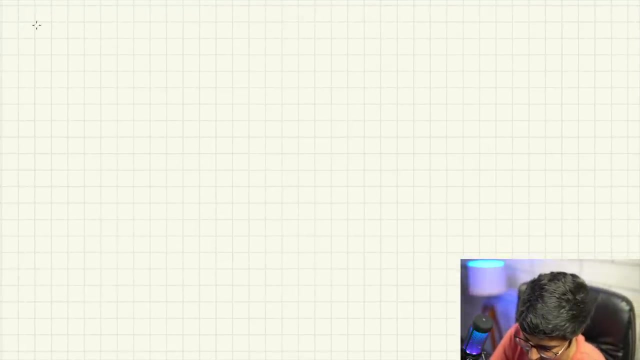 initially is 0 and then in the end i'm just going to return the count. basically, let me not write this code and first show you how this thing is working and what they're asking. so we already know we need to find the even number of digits. so question is: even number of digits? 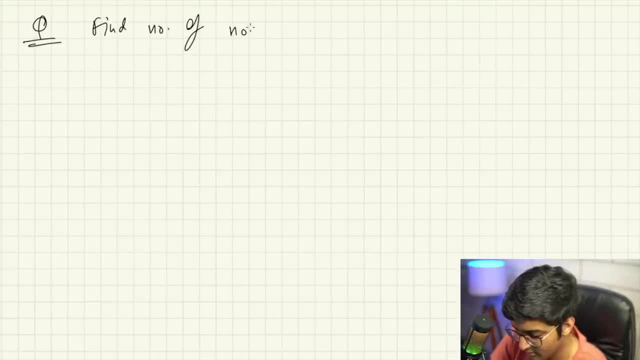 find number of numbers that have even number of digits. okay, for example, if we take array, nums is equal to 18, 124, 917, 36, 1764, 98 and 1.. over there, we know that this is an even number of digits. this is even number of. 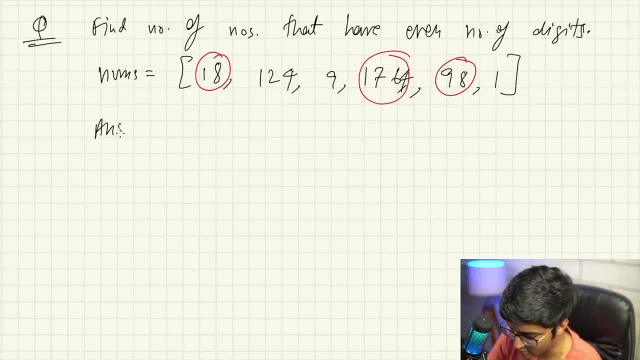 digits. this is even number of digits. so answer is going to be equal to three. three numbers are there that contain even number of digits? so let's say i just iterate over every number and i check: hey, does this number contain even number of digits? if it does, i increase the answer by one. 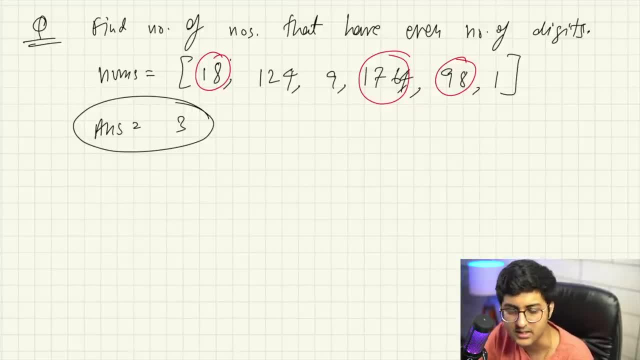 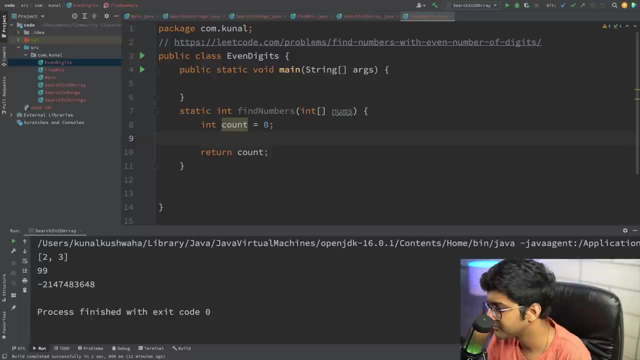 does this number contain even number of digits? if it does, i increase the answer by one. so let's do that thing. how we are checking if it contains even number of digits or not, that i will show you in a bit. so let's say for every number in the numbers, if i can say contains, or i can say even. 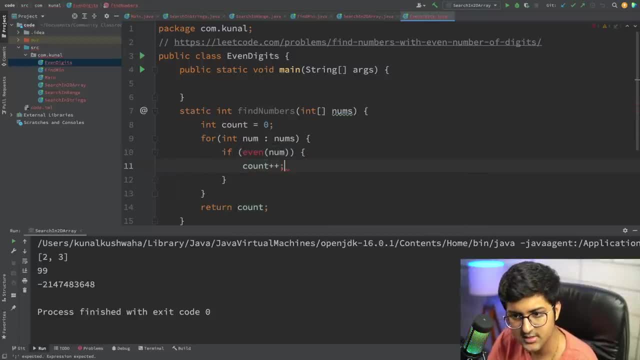 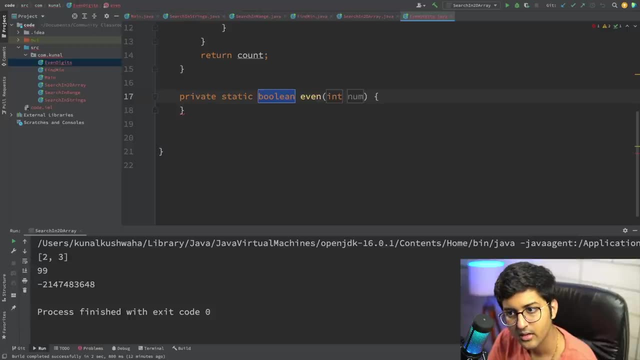 number, then i can just say count plus plus. now i just need to create this function. this function basically tells me whether this contains an even number of digits or not. function to check whether a number contains even digits or not. how can we check that? let's let's see how. 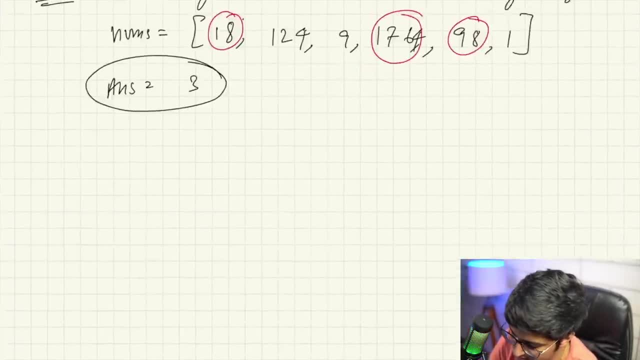 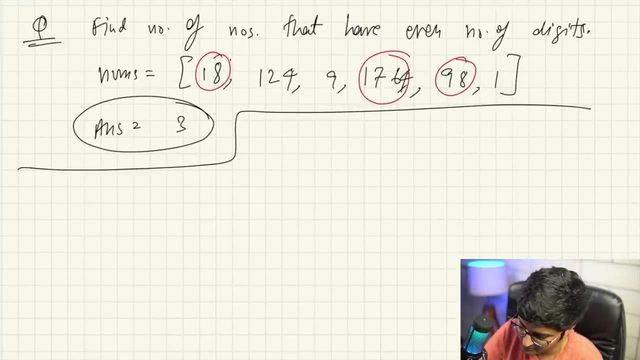 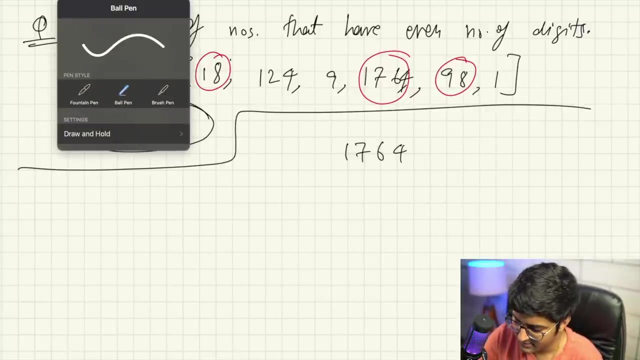 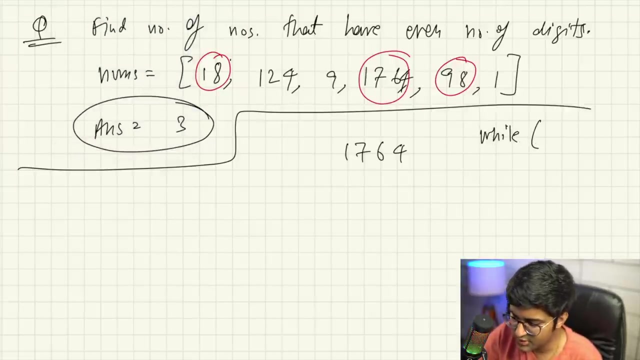 how can we check that? so how can we check whether a number contains even number of digits or not? so let's take any number: 1764, 1764. i know that i can just basically do something like this, that, uh, you know, while this number i just need in order to check if this contains even number of digits or not. i'm telling you how we can check that count the number of digits or not. that is what we are doing now. yeah, i can check my number, then i can check. so let's check this now also, let's now check this. so let's check my number, then i can check this number. so what's we know is that this is an even number numbers. 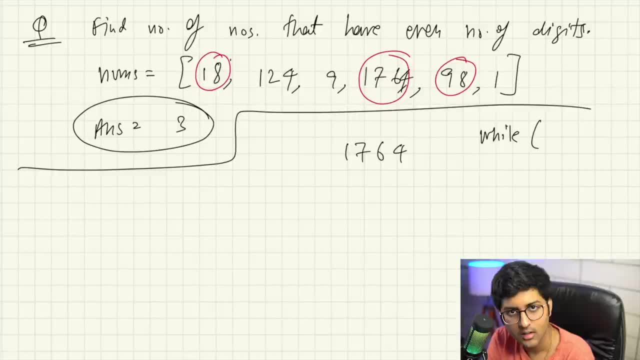 i mean number. can you count even numbers in this fpn? okay, so that's it, this number as one will start to function. digits: okay, count the number of digits. so first step can be: count the number of digits. second can be: convert this into a string and take the length of it. 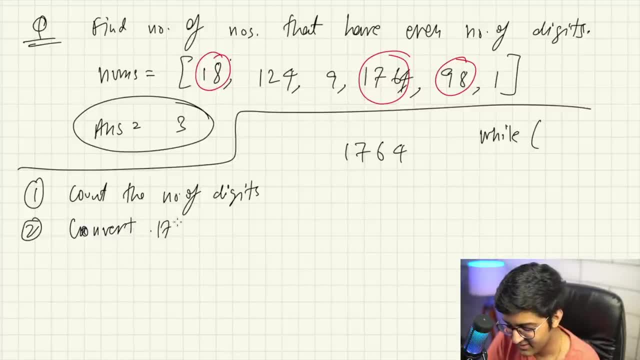 shortcut: convert one seven six four to a string. so you can do something like one seven six four. take the length. that is very simple stuff. you can convert it into string easily. you can just do one seven six four. so six four plus and plus a empty string. it will convert it into a string. okay, that is something you can do. 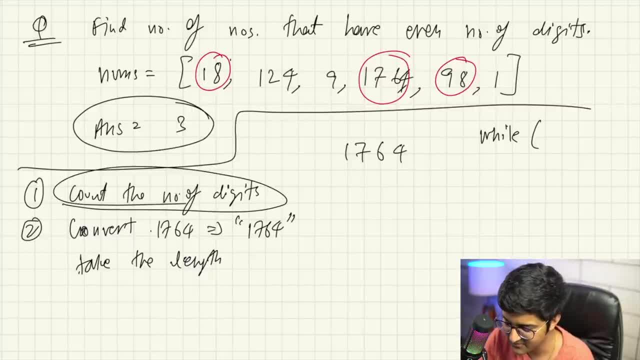 this is very basic stuff. you can do it yourself. I will teach you how to do this thing. so count the number of digits. we can literally count it. so while my number is greater than zero, I can say: count plus plus, and number is equal to number divided by 10. that is it. so it's. 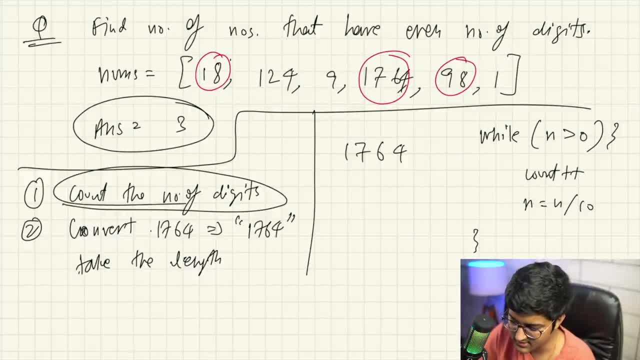 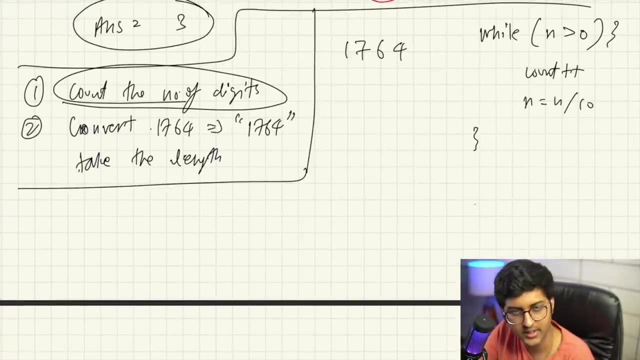 going to do something like this. is one, seven, six, four greater than zero? yes, so count is equal to. let me just write it down so that you can see it. it's once it's going to start from here. it's one, seven, six, four greater than zero, yes, so. 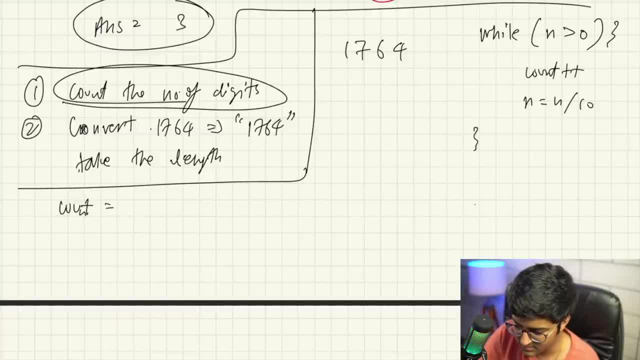 count value is equal to count plus plus. initially it was zero. then it will be one and is going to be n divided by 10. so this will be equal to one, seven, six. it's greater than zero. yes, it is. this will be plus 1 to 2. 1. 76 will be again divided. 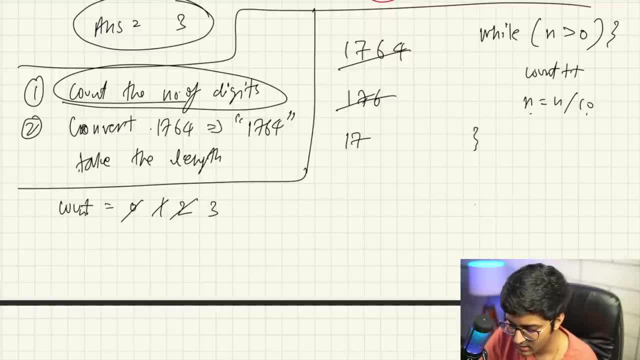 by 10 to 17. is 17 greater than 0? yes, it is. count will be 3. 70 will be divided by 10 to 1. is 1 greater than 0? yes, it is. count will be 4. this will you again be. 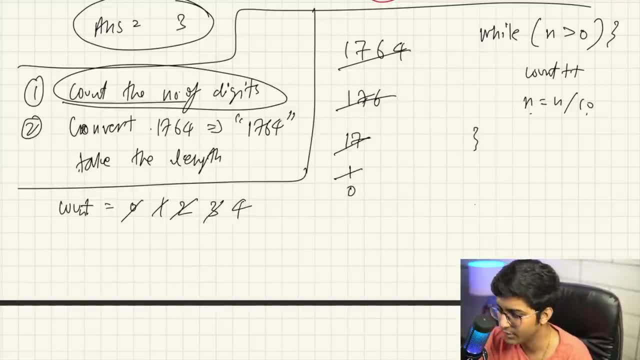 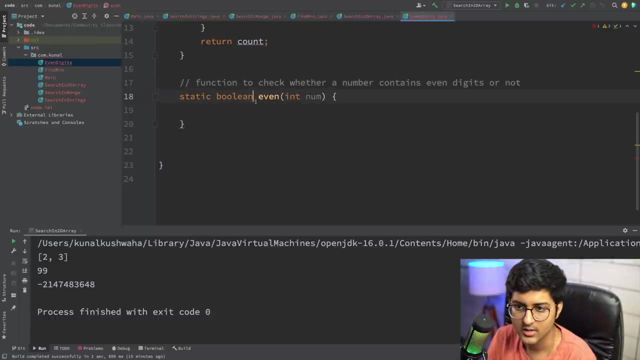 divided by 10, equal to 0 is greater. is 0 greater than 0? no, it's not. answer is 4, hence here. this is how you can count the number of digits. okay, let's try to code this thing so I can say if I want to check the number of digits, so I can say static. 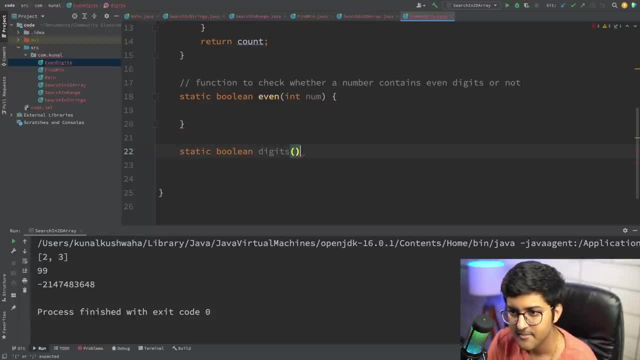 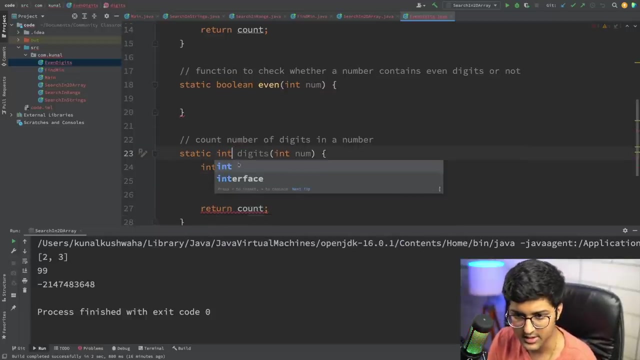 boolean digits in a number count, number of digits in our number. so I'm just going to say: in count is equal to 0. in the end I'm just going to say return count. and here I'm just going to italics. is this going to be integer? and then I'm just going to say: 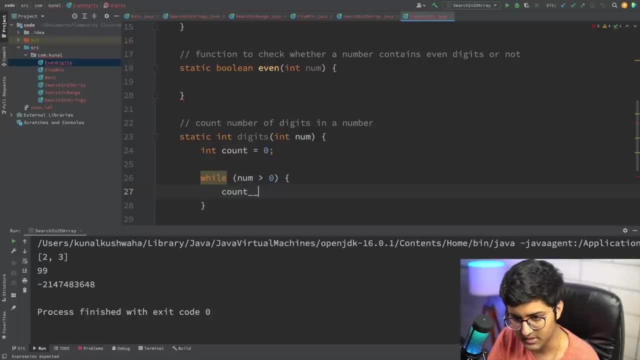 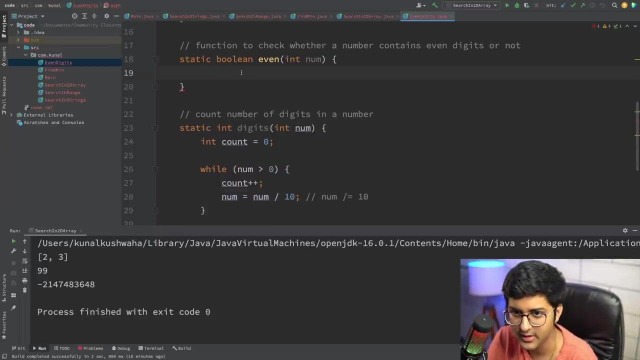 while my number is greater than zero. count plus. plus number is equal to number divided by 10. or you can write something like num divided equal to 10. okay, let's try to run this. and here, how do we know it is even or not? I'm just 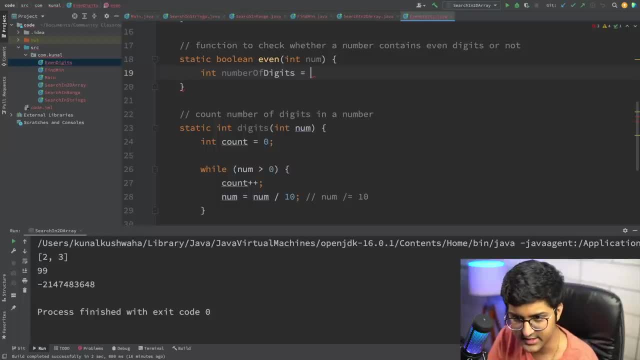 going to say int number of digits is equal to. I can just call the digits say in past number over here i can say: if number of digits modulo 2 is great, is equal to, equal to 0, then i mean that it is even so. if the number of digits is an even number, how do we check if a number of 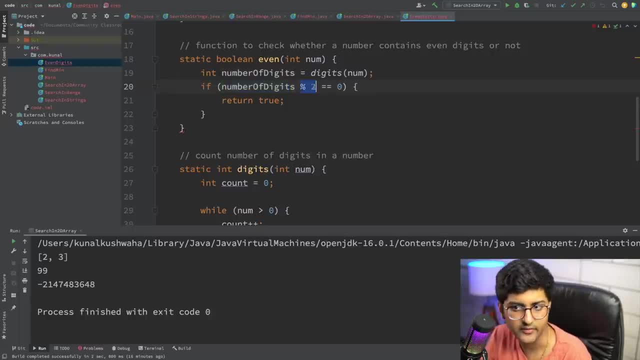 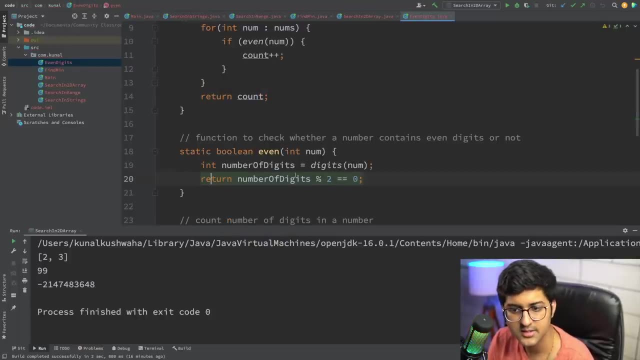 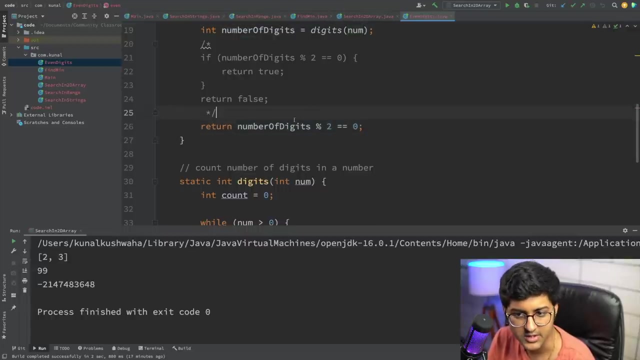 if, if the number is an even number, if the remainder with 2 gives 0, then it's an even number, otherwise return: false. i can also shortcut this. this is a shortcut. okay, this shortcut also we have discussed previously when we're doing functions and stuff. so this statement return basically means: 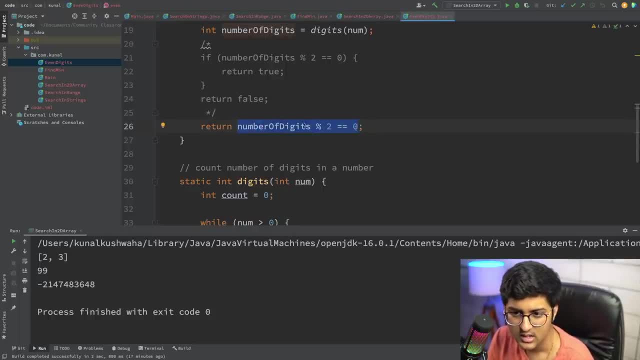 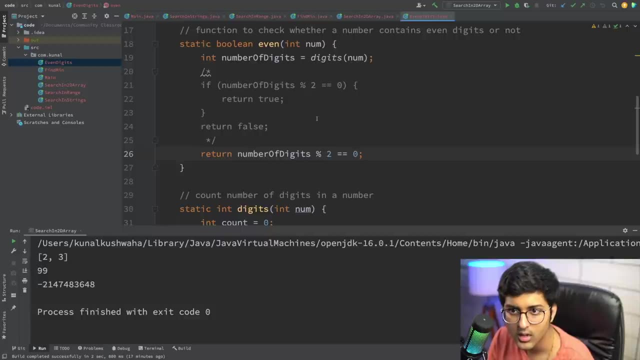 if this statement is true, return true. otherwise return false. whenever you return a boolean statement, it returns true or false. if not return true, then return false. if number of digits modulo 2, the remainder of 2, gives 0, it will return. true means it will be even. that is it. 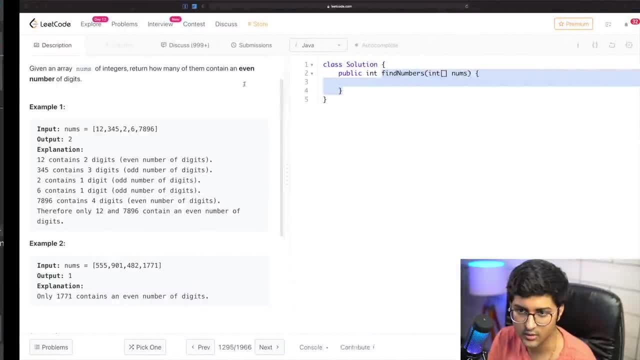 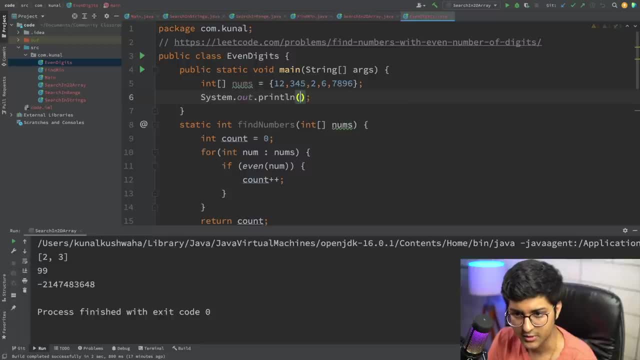 in nums is equal to. let's say we copy this, then i'm just going to print my answer: find numbers: nums run. it should give me 2 because there are only two numbers that contain even number of digits: 12 and 7, 9, 7, 8, 9, 7. 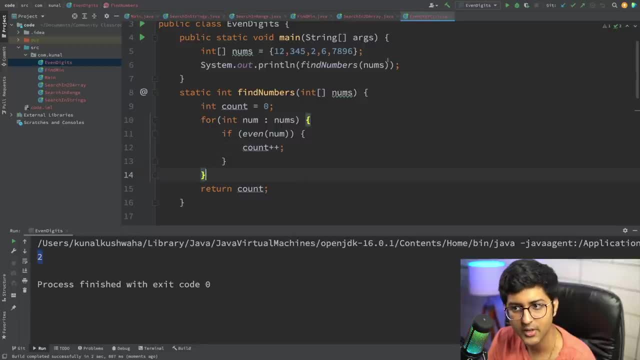 so if i'm going to print my answer- find numbers, nums run, it should give me 2, that's correct. okay, if you want to run the digits example so you can say: find the number of digits in any number. so let's say this should give me how many digits. 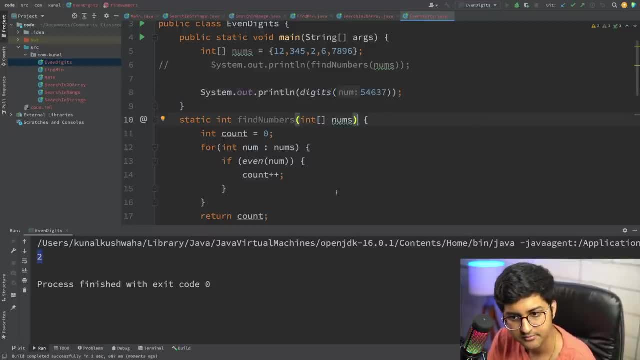 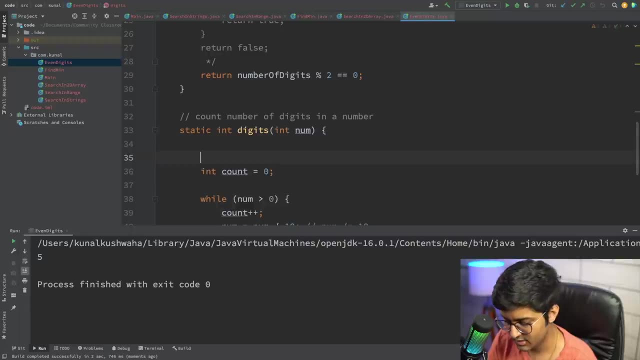 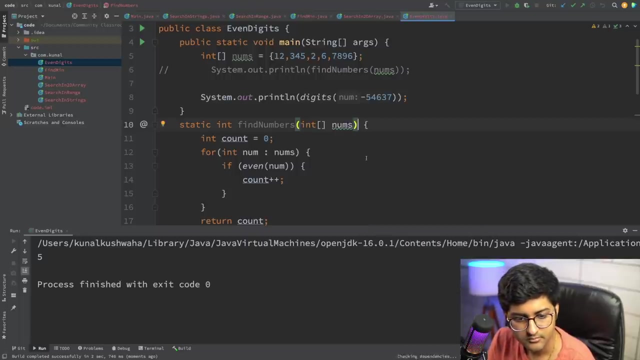 one, two, three, four, five, five digits, okay, and you can just add a case over here that, uh, initially you can say something like: um, you know, let's say i'm going to write a case over here that, uh, initially. you can say something like, um, let's check for, uh, negative numbers as well. 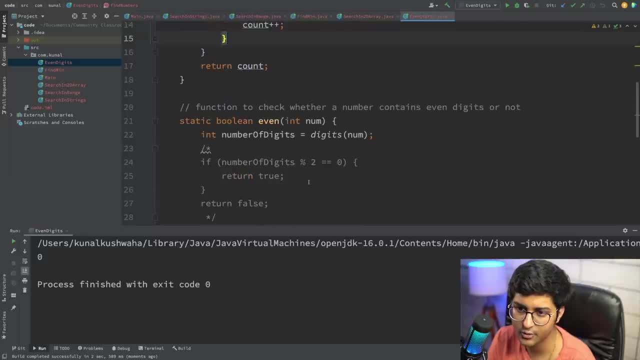 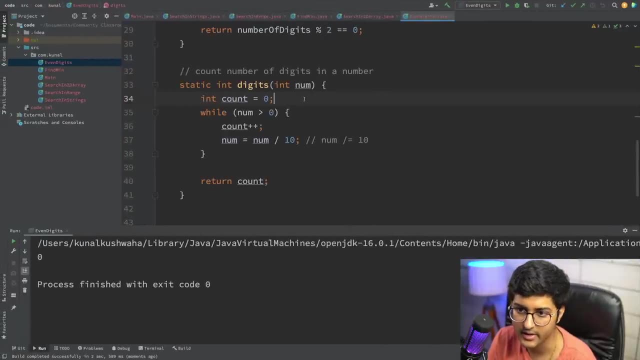 yeah, for negative numbers we would have to convert it. so basically we can say: isn't, isn't the answer they're taking, they might be taking negative numbers. so here we can just say for negative numbers that, um, i can say: if number is negative, make it positive. 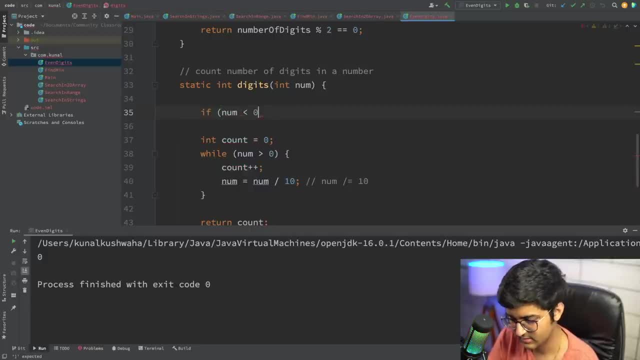 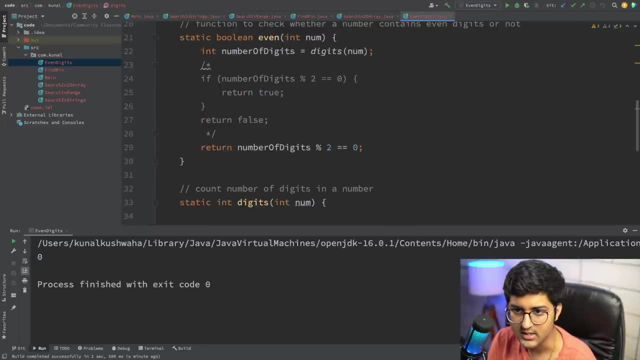 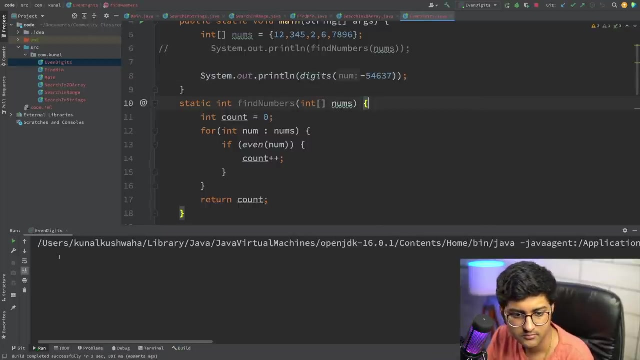 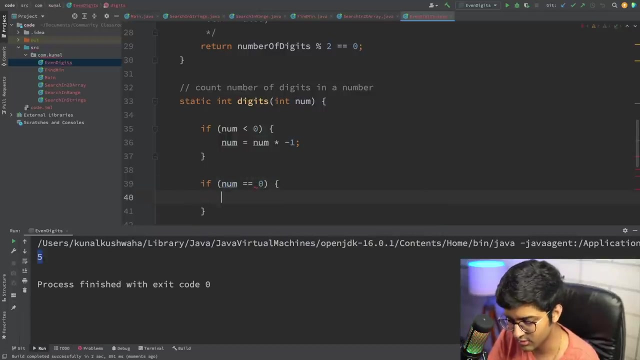 number is less than zero, i can say number is equal to number into minus one. okay, in this case, now for negative number, it will give me five, also five. and also one more case i want to add over here is is if the number itself is equal to equal to zero, return one, because otherwise it will never increment this for zero. it also. 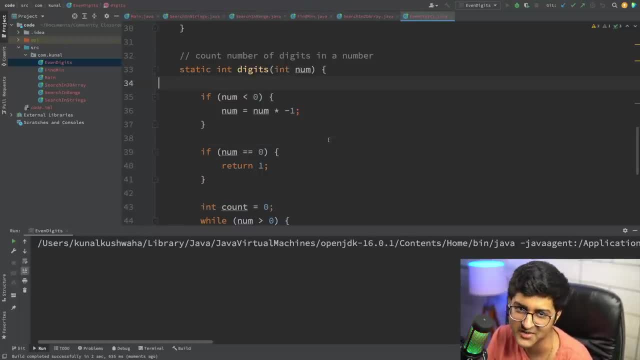 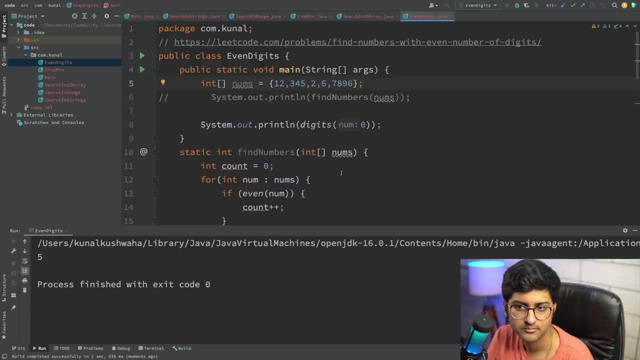 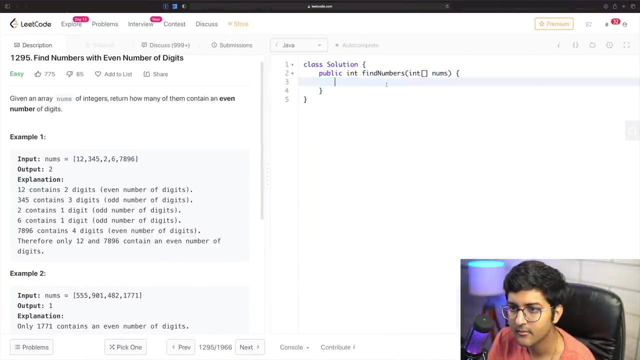 also it will give zero contains zero digits. but that's not true. zero contains one digit. so if i just add zero over here now, it will give me answer as one. okay, let's try to submit this code copy and paste- good old copy paste. and then i can just say something like: 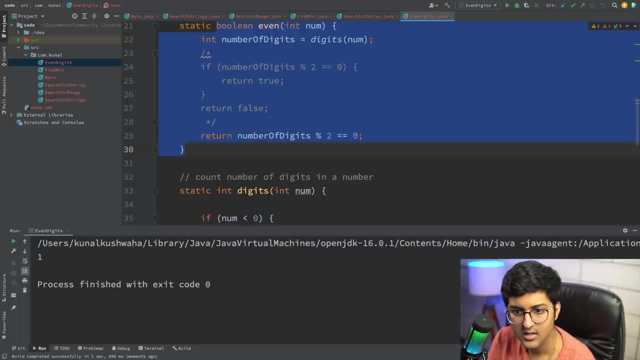 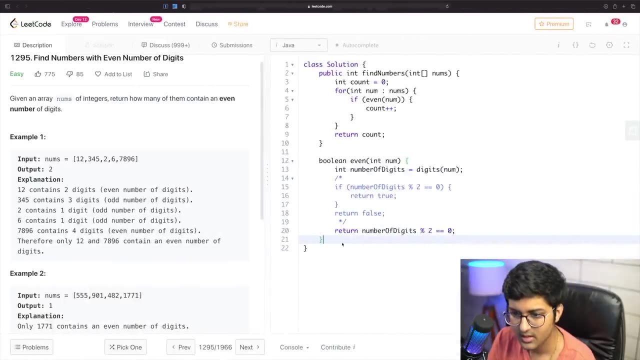 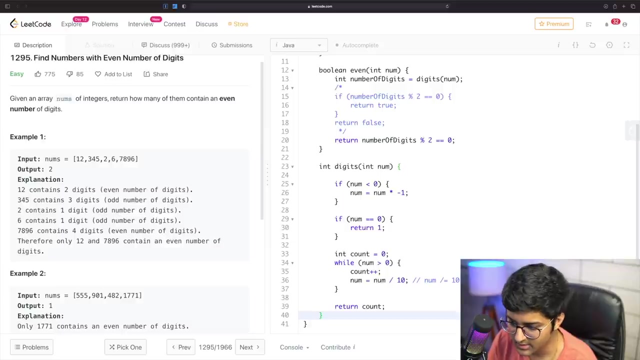 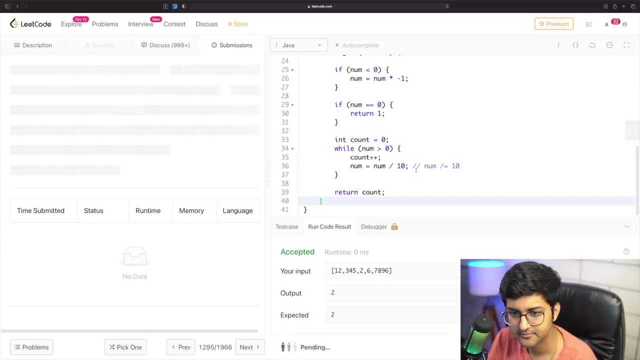 um, boolean, and then i can say something like this thing: why we are not adding static in lead code? uh, we will cover in object-oriented programming, and that looks good. let's try to run our code giving the correct answer. let's try to submit it. yay, okay, it's accepted. we can try to obtain the answer here. 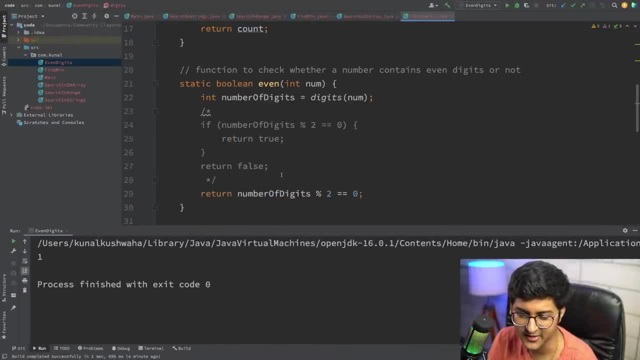 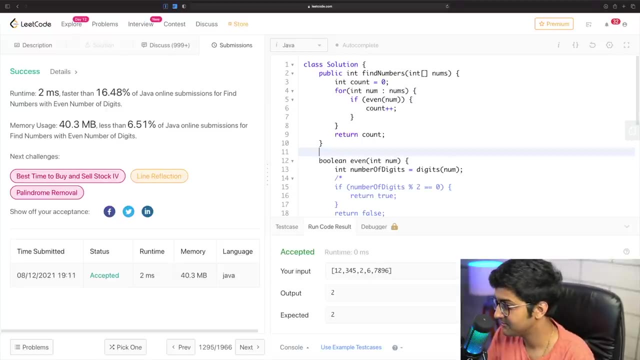 we can try to obtain the answer here. so it should work well, absolutely it should work well. let me show you how we can optimize this a little bit. let me show you a nice little trick. okay, so how can we optimize this? let me first show you how, and then we can. uh, you know then, 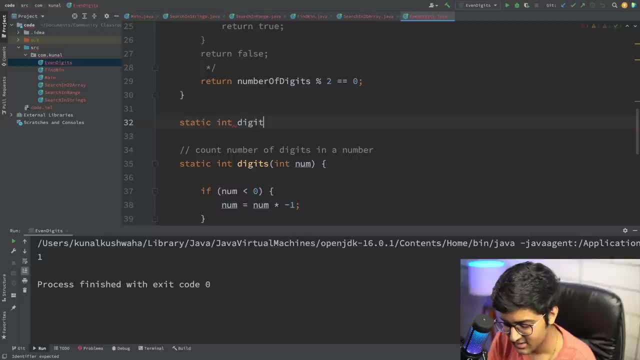 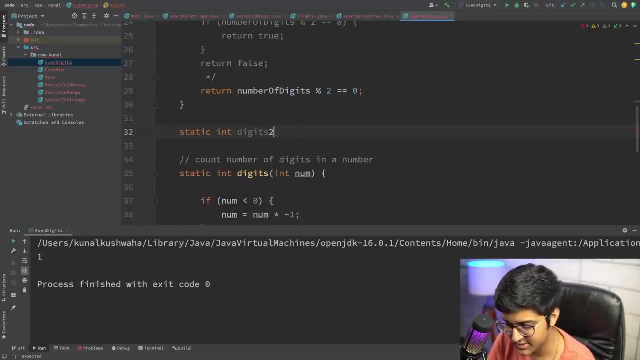 we'll cover how it actually works. so basically, in order to find the number of digits- right now i'm like iterating over the entire digit and stuff, so i can say int digits to. second way to find number of digits. so here i can see um doi, both indicate the same value- in order to find the number of. 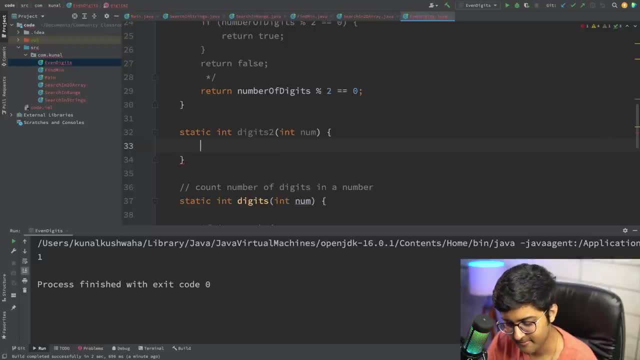 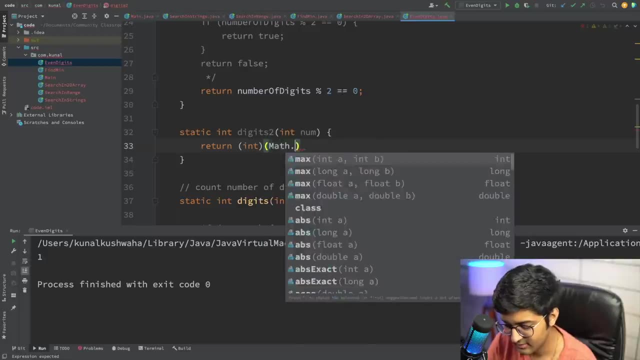 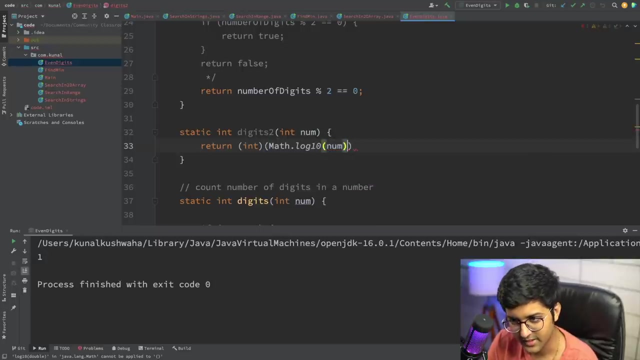 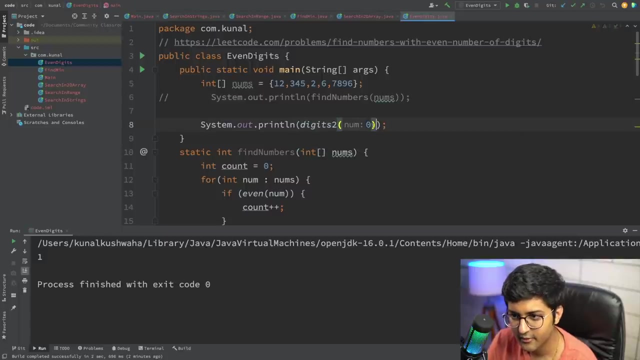 digits. so the last step is to just first of all find the number of digits. it's basically the second. I can say return integer value of the log, math dot log of my number divided by- I think it's log 10- only, that's fine- plus 1. let's try to print digits 2 for. 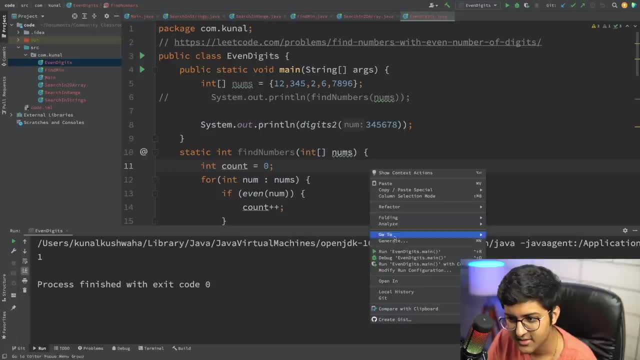 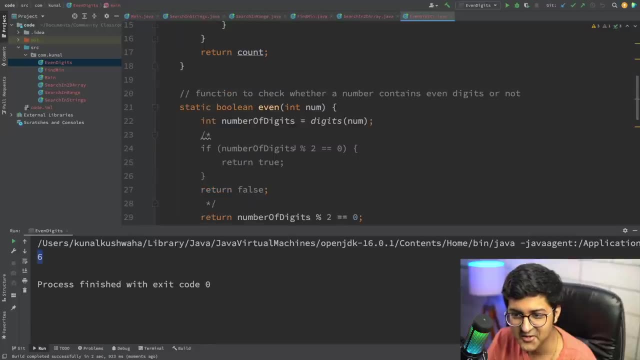 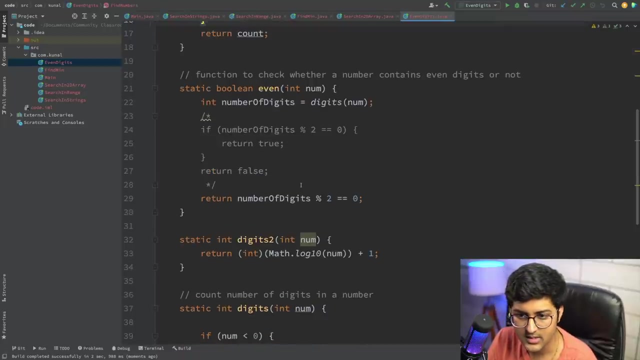 something like this: it should give me 6. how it's working, I'll tell you later on 6. this is a shortcut to find the number of digits: integer value of log 10 of that number plus 1. okay, and for negative numbers I can add the similar check I. 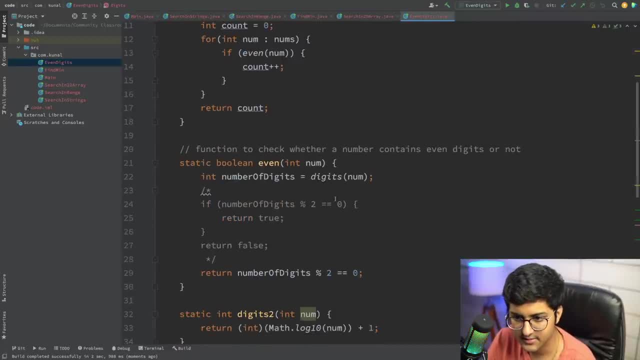 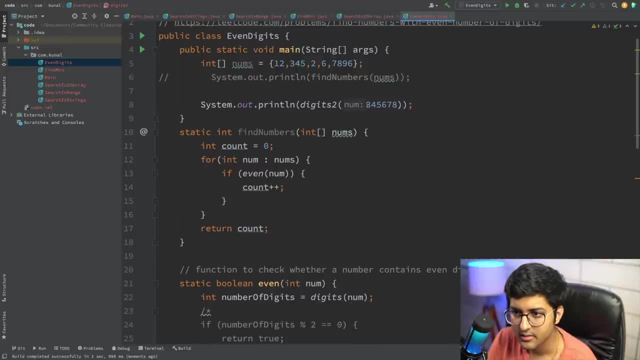 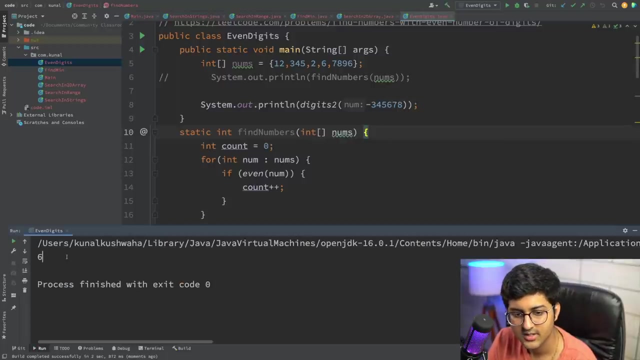 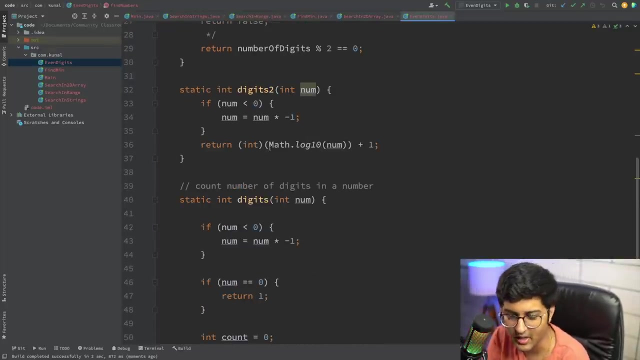 can say something like this: all right, and then I can just say: negative of this number. it should give me six digits. six digits. how is this thing working internally? so, basically, this is something we cover in number systems. okay, this is a formula, but I will cover it in number systems. okay, how this thing is working, I will cover it in number. 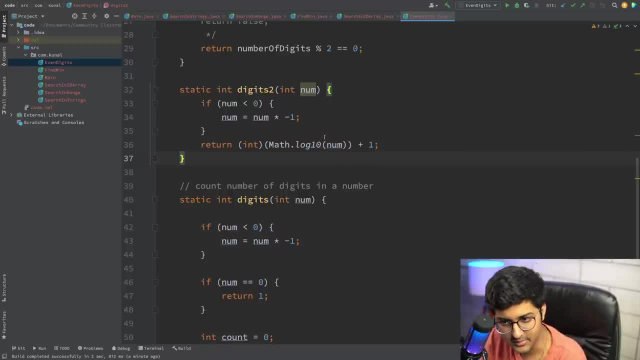 systems. this is a shortcut. so basically, if you want to get the number of digits in any number, let's say you want to get the number of digits in the binary representation of this number. if, for example, if this number was converted to zeros and ones, how many number of digits would it have? then you can just take the. 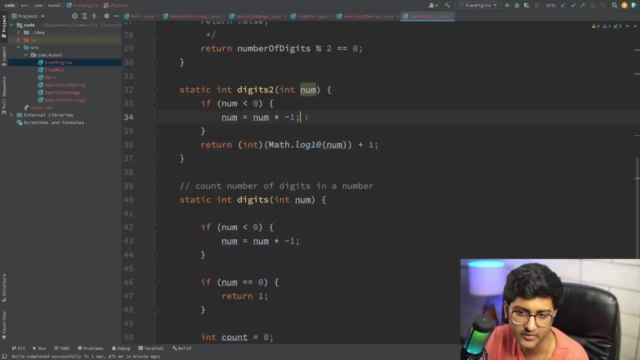 log 2 of this log base 2. okay, if you want to get the number of digits in the octal representation base 8, so this don't worry. I am not going to cover this right now because we have a separate module on this number system. we will. 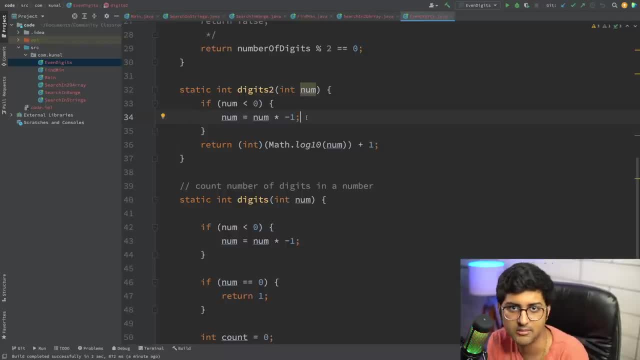 cover it in very, very detail. what is base? what is number system, how to convert one number system to another number system. you know how to read binary numbers and how to get this particular formula. everything we will cover in detail. so if I just replace this, this should work as well. so for number systems, I will cover it in very, very detail. so if I just replace this, this should work as well. 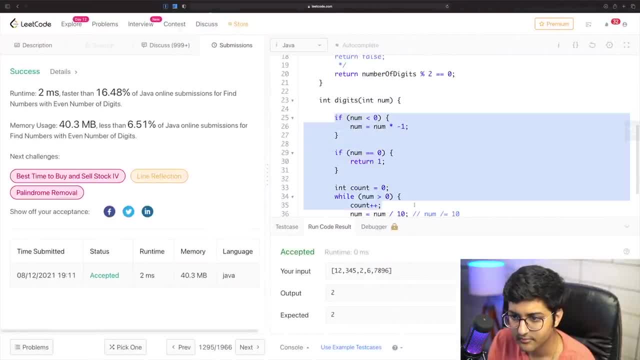 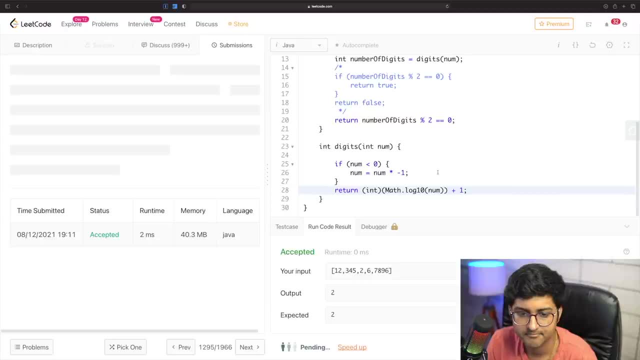 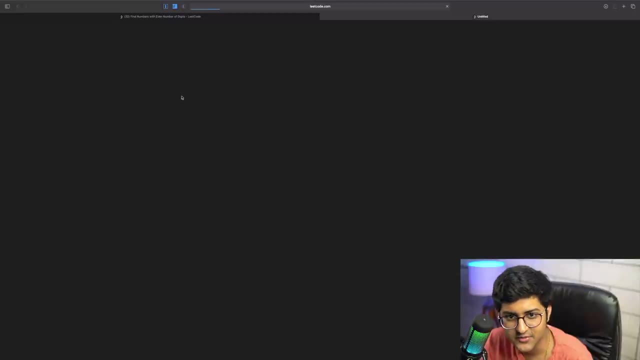 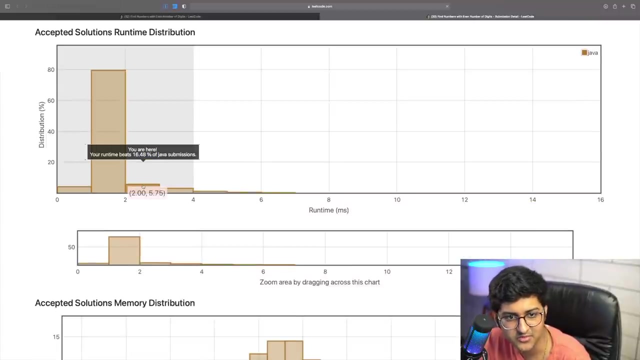 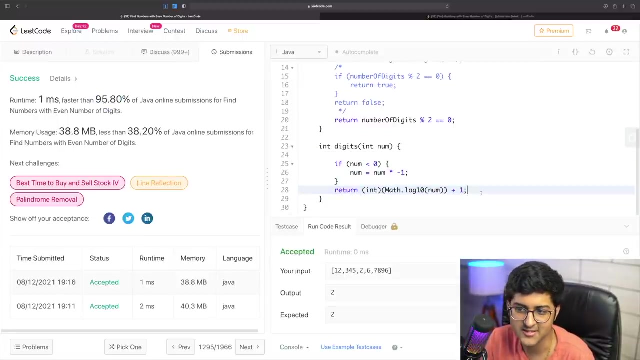 if I just replace this, this should work as well. well, submit faster than 95% of Java submissions, and this one was faster than you can see, faster than 16%. this was the first one. this is faster than 95% of Java submissions. this program only change I made was this: this is why time. 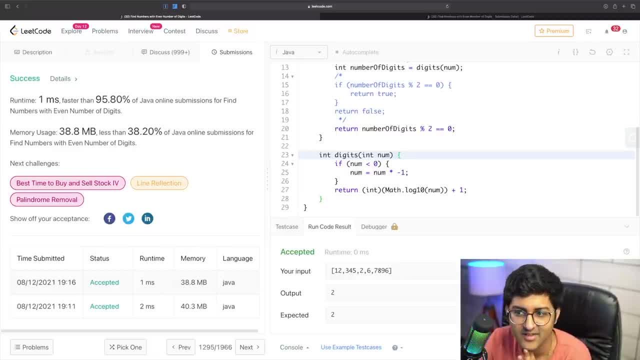 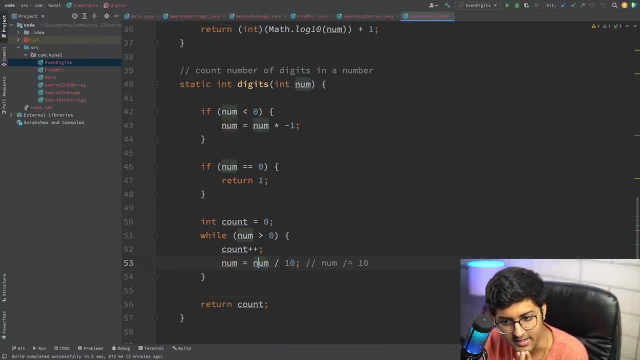 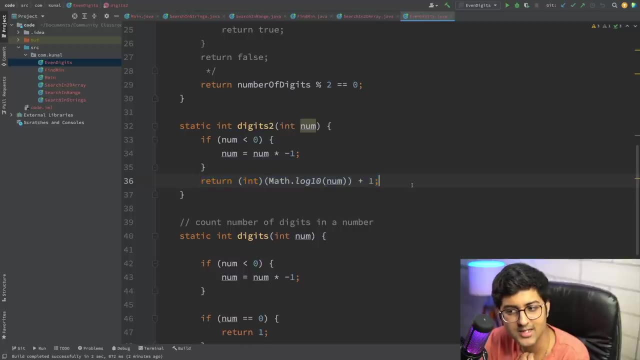 complexity analysis is very, very important here. it was running the while loop, running the while loop for every number, you know, and taking division and everything, but this was able to do it in just one single step: no while loop or anything. one single step, very optimized. I can optimize this step as well using 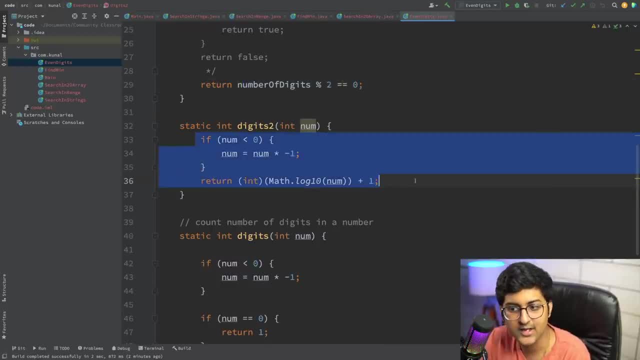 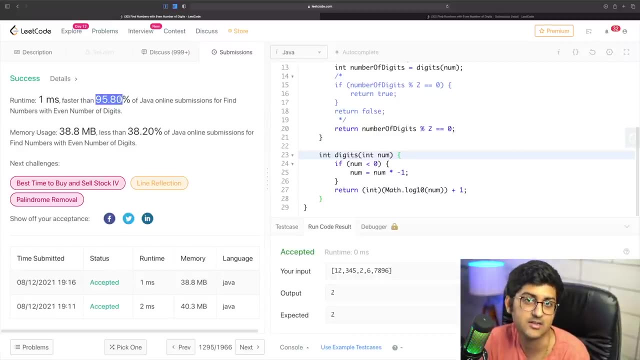 a and operator, but not right now how this thing optimized. why is this so fast? literally so fast. this is 16% faster. new submission is 95% faster. all of these tips and tricks we will learn as we progress over, you know, with more detailed questions and more detailed topics, and for this particular section, this: 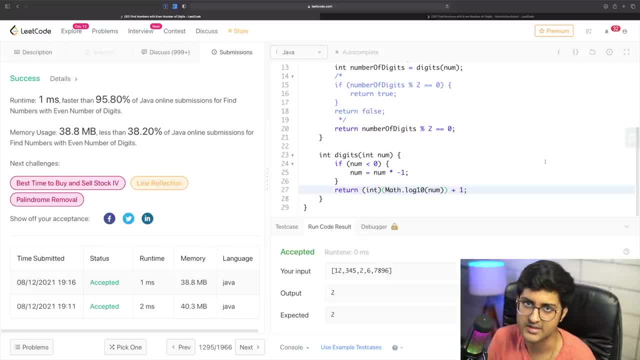 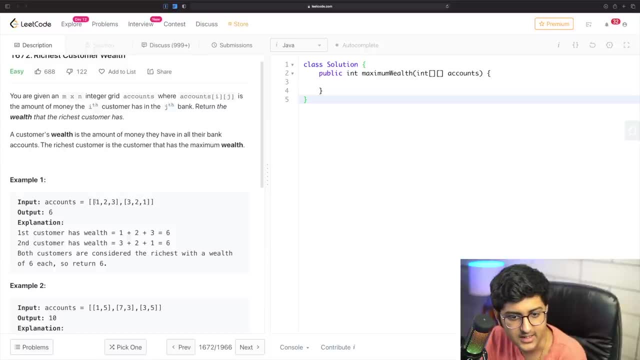 particular thing. I will cover it in detail. when we learn about number systems, let's look into the next question. so now this is the next question. it's very easy question. so basically it says that this is like the 2d array is given and each particular array is like the account number. so basically, a person has 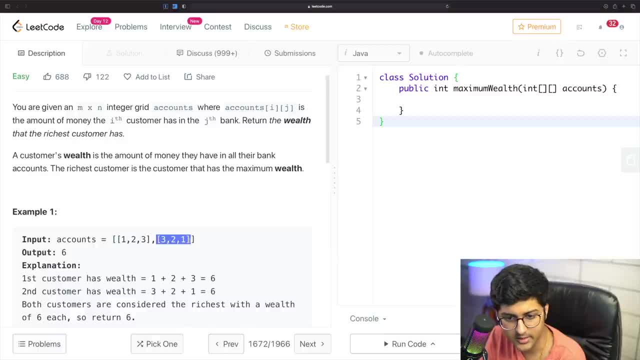 this is person number one. this is person number two. person number one has three bank accounts. person two has also three bank accounts and the person number in the first bank account of the first person there is the wealth of one. the second bank account of the first person wealth is two. third account number of. 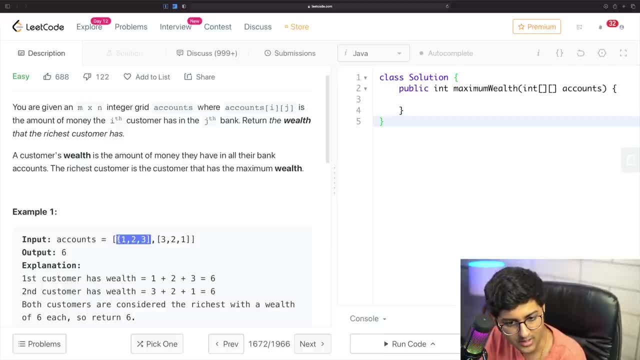 the same person wealth is three. so the total wealth of person number one is one plus two plus three, which is H, 6. ok, total wealth of the second person is three plus two plus one. he has a bank account in three banks, so again six for the second one. this is: 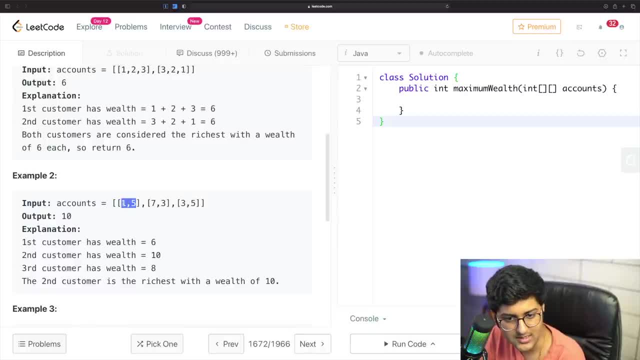 person number one. they have two bank accounts, total isuck. for the second person, total welfare is 10. for the third person, total wealth is it to tell us the richest person is second person? now i answer this, finished. this video is here and see you in the next conference. that's why answer is: the potential is 7. if you hit neutral or authorization is the same. Points are 3, middle of year 3,. The second person is 8. total wealth is 1. Another person from the bank all the same, or A With modelacji, also needs the same amount of money and 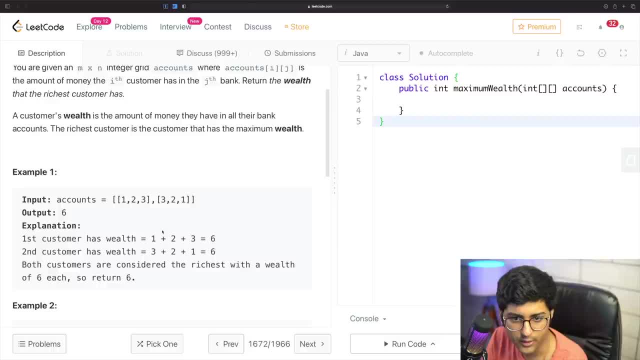 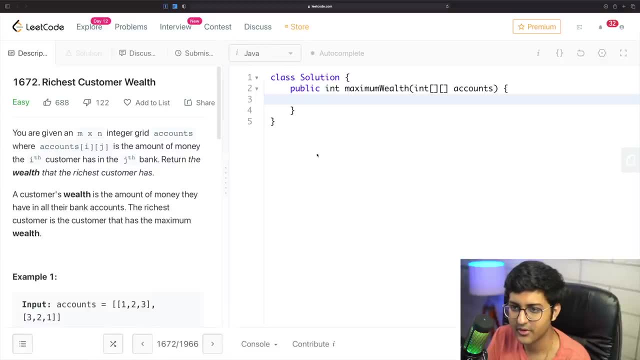 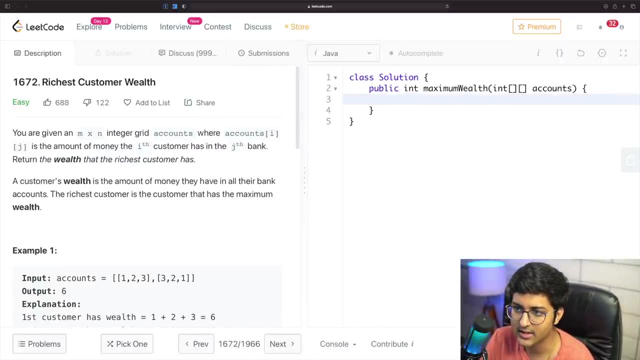 wealth of the second person, which is 10. that is what we want to do. it is just a simple question of iteration, nothing new over here. okay, so if you try to directly code it on intelligent idea- sorry, not intelligent idea- directly on lead code, but since you all want the solution, so I can directly code on like intelligent as 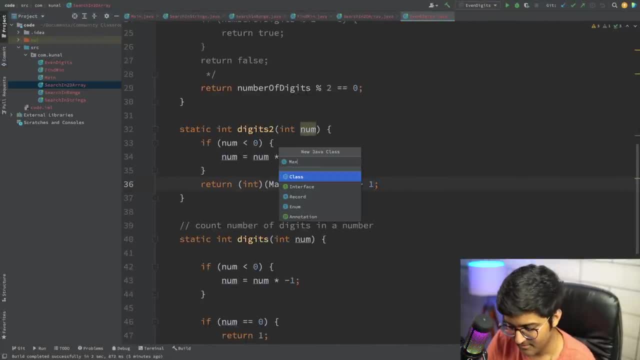 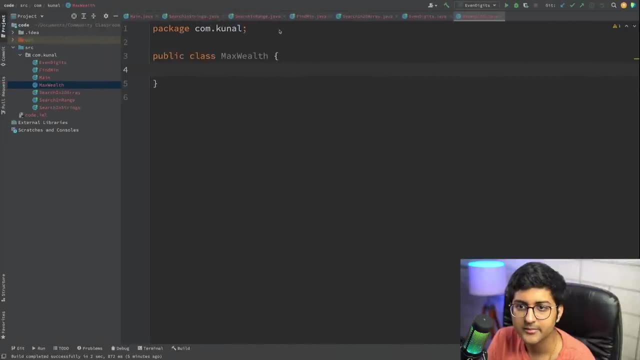 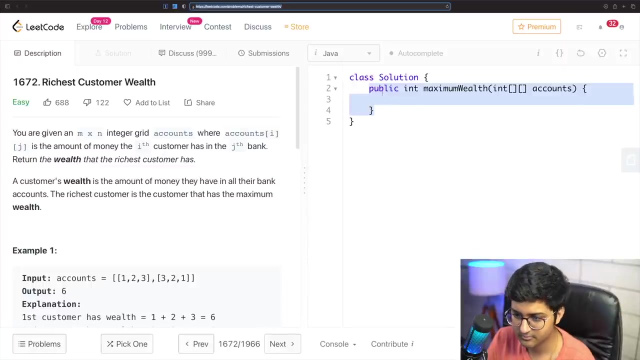 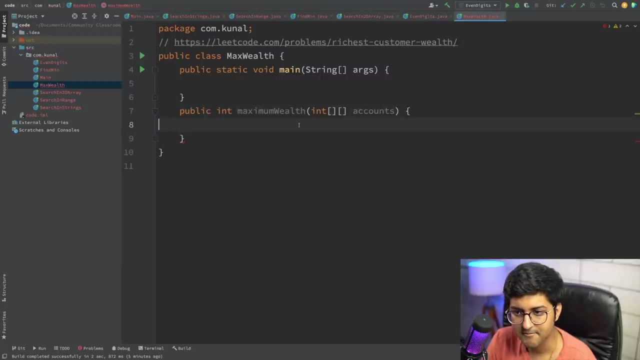 well, max wealth. try not to practice on like intelligent, like this, because auto completion is not a very good habit. so try to directly code on lead code, because that will help you in the interviews. okay, so here I will just say: for every bank account, for every person, for every. 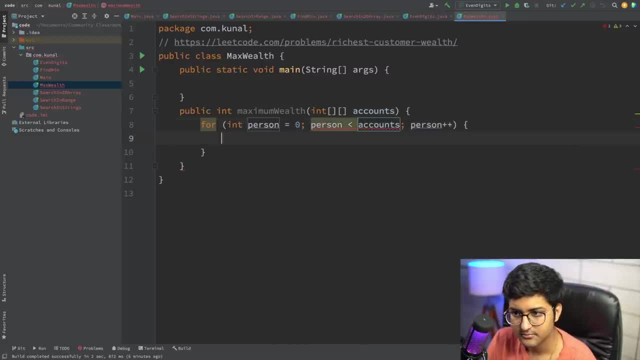 person in accounts, dot length. okay, then I can say: for every bank account, for every account which is going to be trading over the same thing, persons- sorry, accounts of that person, dot length. similarly, here, person is equal to row, account is equal to column. I don't think I have to explain this, we have done it. 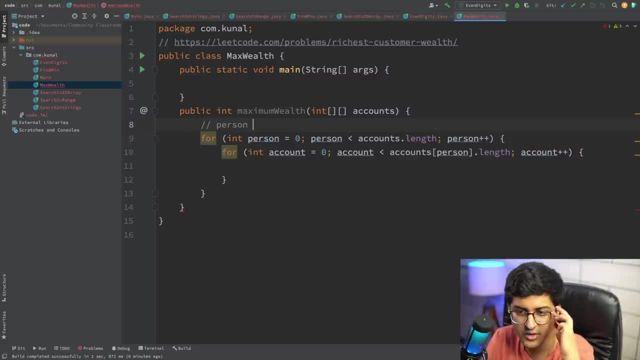 like many, many times. we also revised this in this section. we also revised it in the arrays section and account is equal to column. so before saying hey, Kunal, you did not explain this in detail. iteration of 2d arrays: we have covered multiple times. please check this video, previous section only how to search in a 2d array. 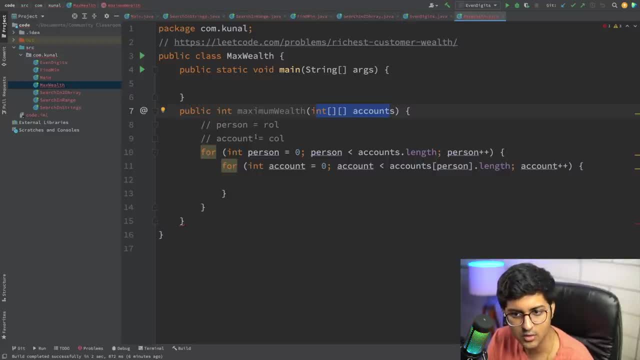 check out this section- this is the same thing, row is person, column is account- and also check out the array section. arrays video that we did link is in the description. so this is iterating over every column and I'm just to take a sum of every column. so whenever we start a new column, when you start a new column, 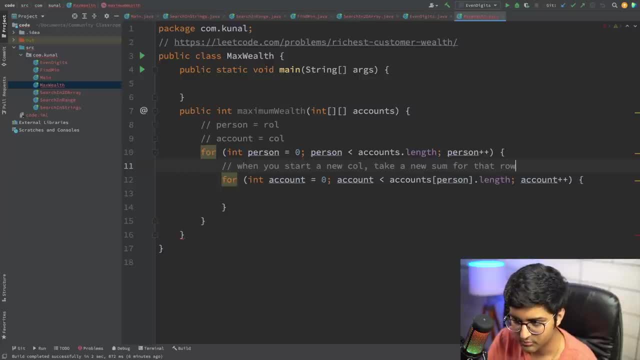 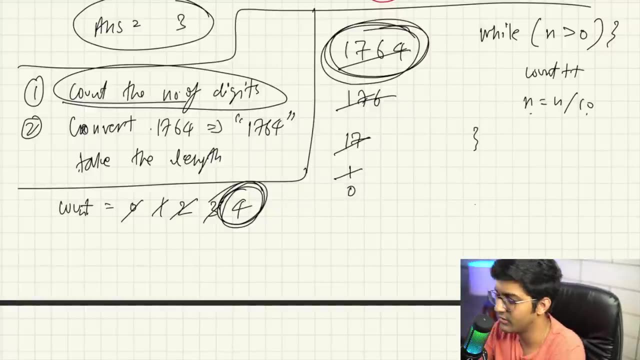 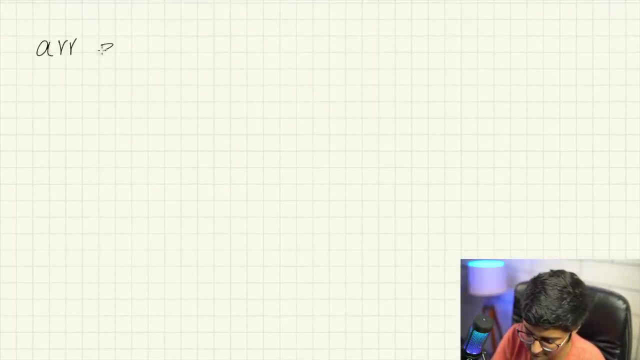 take a new sum for that row. okay, so this row contains this particular. basically, let me just only write this down over here. okay, let me show you what we are doing over here. i think it's very simple, should not be elaborating this much, but never mind. 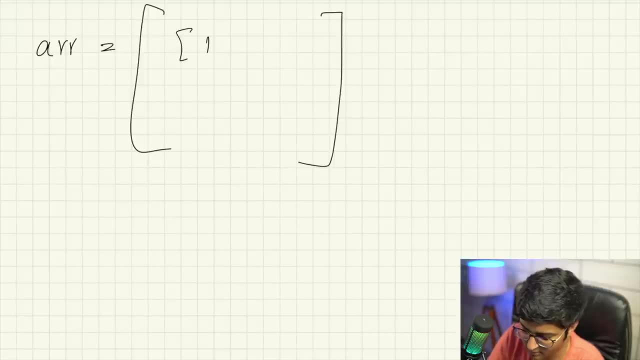 person one has wealth of one, two and three. person two has wealth of nine, one and six. person three has wealth of three, three and seven. this is person number one has three bank accounts. person number two has three bank account. person number three has three bank accounts. this is for every row. 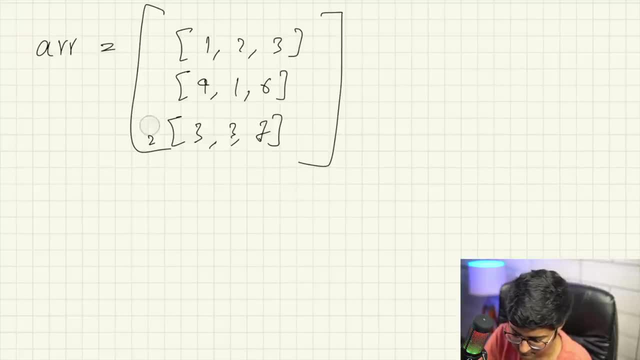 zero one two. let me just write it in a different color. index of every row. example. i'm going to write this as this is: one row: zero one two. index of every column: zero one two. these are the columns, these are the rows, so the outside loop is going to run for every row. 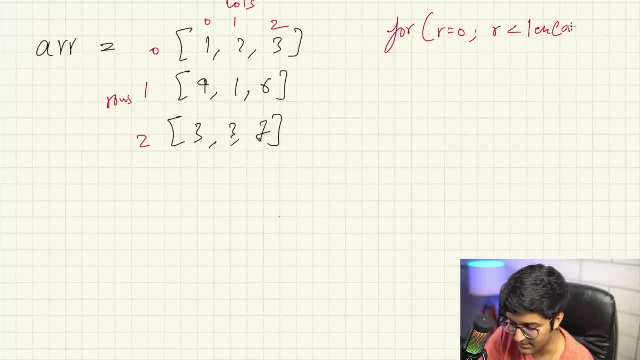 so when i'm saying for row is equal to zero, row is less than the length of my array and row plus plus. and then i'm saying for column is equal to 0, column is less than the length of that row and column plus plus. so here it's actually going through every row. the outside loop is going. 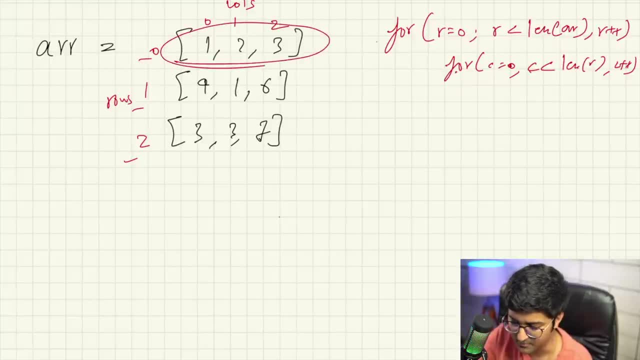 inside loop is going through every column of that row. this is going through every column of the each row. okay, that is what it's doing. so when rho is equal to 0, this thing is going to iterate over this. when rho is equal to 1, this thing is going to iterate over this thing. 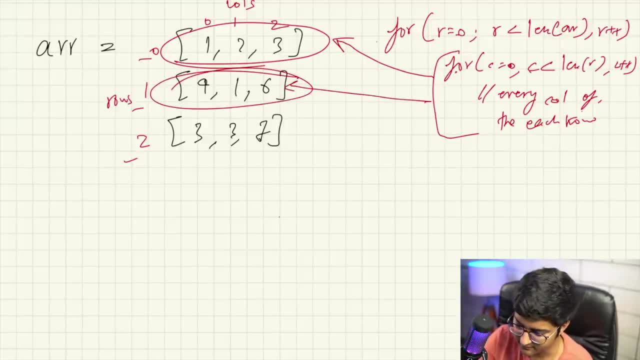 okay, very simple stuff. so when rho is equal to 0, it will iterate over this thing. here i'm just going to say something like that: row sum- sum of this entire row is equal to what initially zero. and here in this for loop, i'm just going to say: row sum plus equal to every single element one. 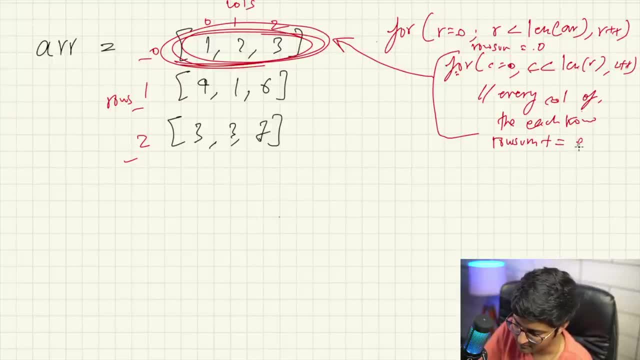 plus two plus three, okay. so in this case, we are going to iterate over this thing. or i can say: what is the element? very simple element is nothing but arr plus equal to- sorry, not array of row, comma, column, okay. and when you come out of this for loop, when you come out of this for loop, 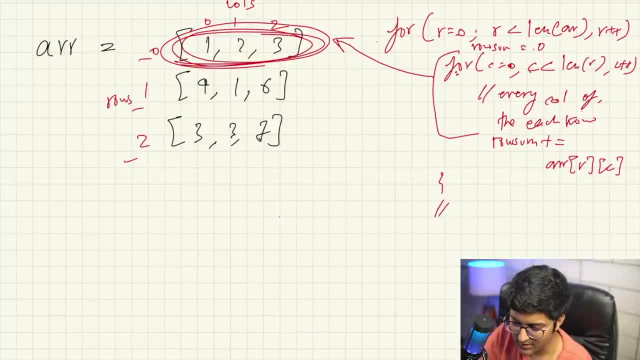 one row will be finished. okay, one row will be finished. you will have the sum of that row. so now it's going to check with the main answer: okay, if this row sum is actually greater than the maximum value so far, then the maximum value is going to be equal to row sum. that's it. that's our question. iterate over every row. take the sum of. 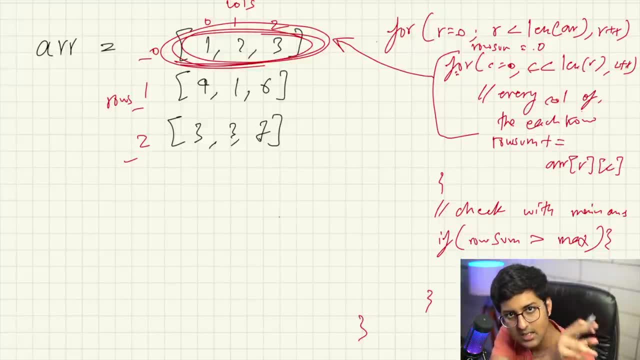 every row. okay, take the sum of every row means every column in that row and then check when. when you are done with every line, when you're done with every line like this, check it with the main answer first. it's going to say: okay, row sum is going to be equal to what one plus two plus three. so it's: 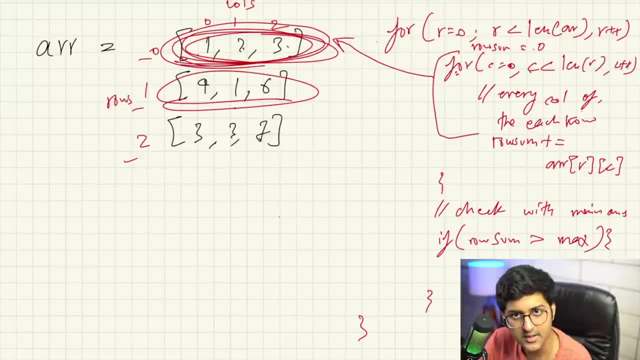 going to say okay. answer like: currently for this row, the column is three. is this greater than the maximum sum? it's going to be like: let's say maximum sum initially is equal to zero. it's going to be like: or: index dot negative value like the index dot minimum value. it's going to be like: 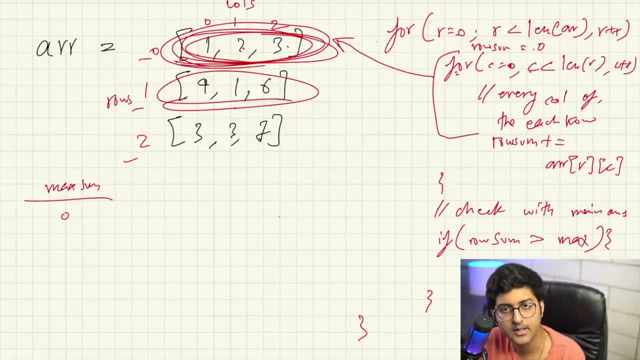 hey, is uh, one, two and three greater than the maximum value so far? it's going to be like, yes, it is so sorry. is six greater than the maximum value? so far? it's gonna be like, yes, it is okay, the answer is six. then it's going to initialize: row sum is equal to zero again, so row sum initially was six. 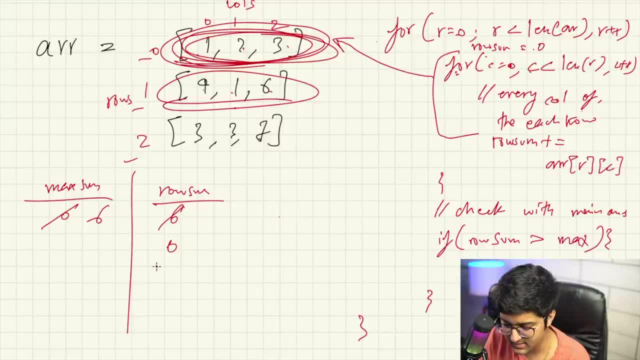 then it will be zero again. then it will taking the nine plus one plus six, sixteen. then it's going to come out of this for loop again. then it's going to check like: once it's done with this line, once it's done with this line, it will come out of the for loop. then it will check: is sixteen greater than? 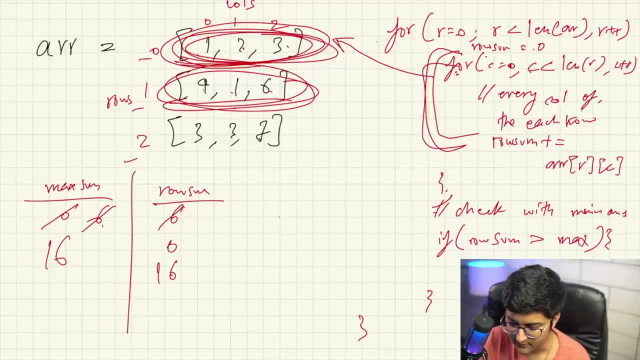 six- yes, it is maximum sum so far- is equal to sixteen, then for next it will be like thirteen. it will be zero again, then it will check, start from again. so basically it will be zero again and start from three plus three plus seven. thirteen is thirteen greater than sixteen when it come out. 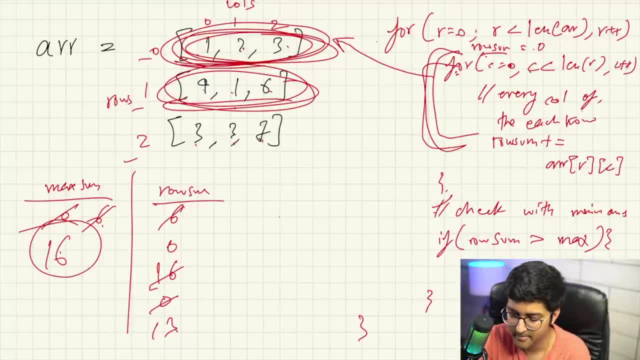 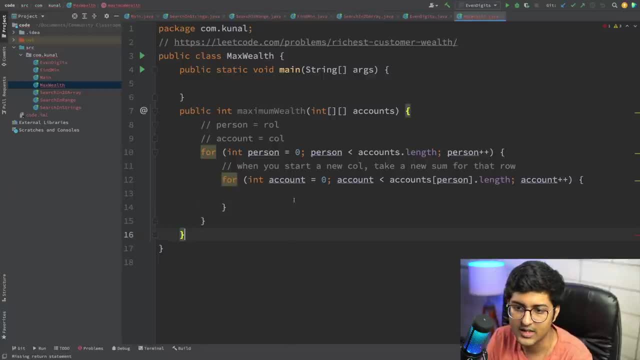 comes out of this for loop, it's gonna be like: no, it's not, the answer is sixteen. okay, very simple stuff. so let's try this thing. so basically i'm going to say int sum here is equal to zero. i can say sum plus equal to accounts of that person's account. 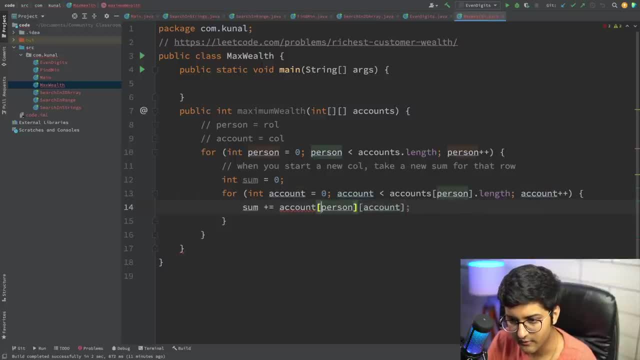 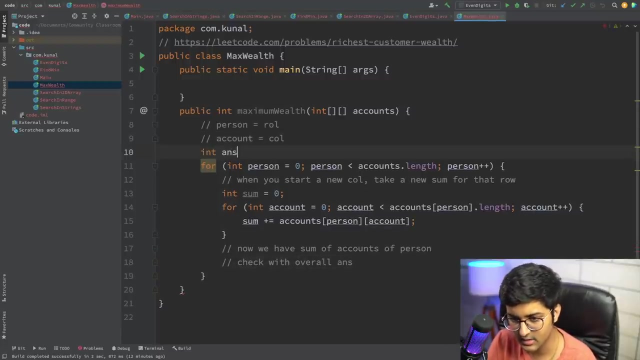 number accounts of this thing when i come out of this loop, when you come. so here now we have sum of accounts of person. okay, check with overall answer. so overall answer i can take initially i can say in answer is equal to integer dot min value. so here i can say for the overall 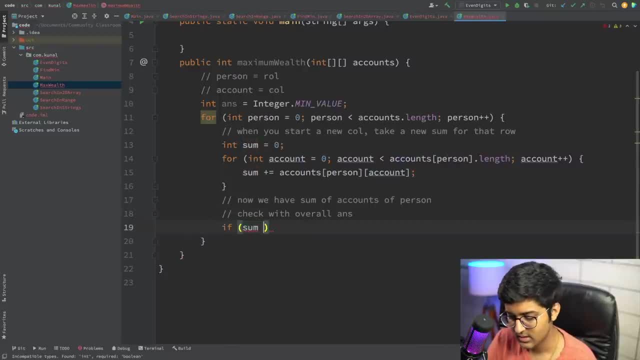 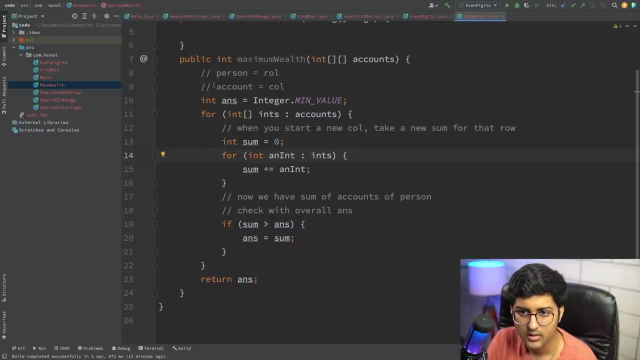 answer. if the sum is greater than the answer, sum is equal to. so the answer is equal to sum in the end. just return my answer. i can also enhance this. since i'm not really using the index, i can enhance it. okay, you can copy this and let's see if it runs or not. 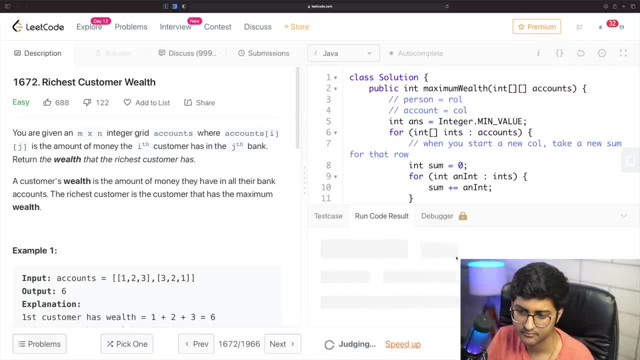 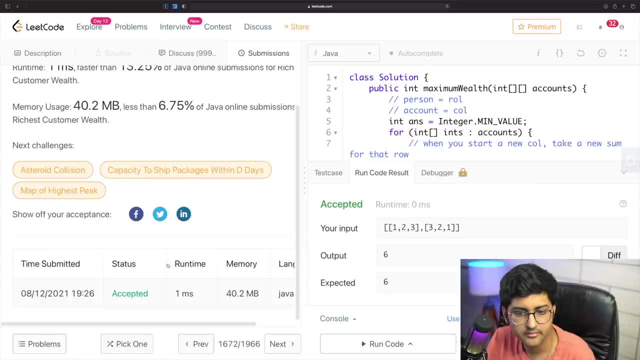 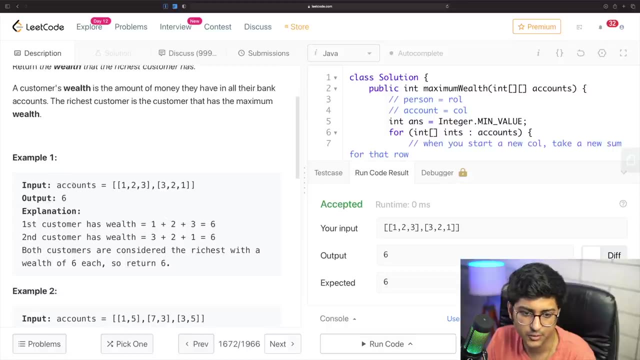 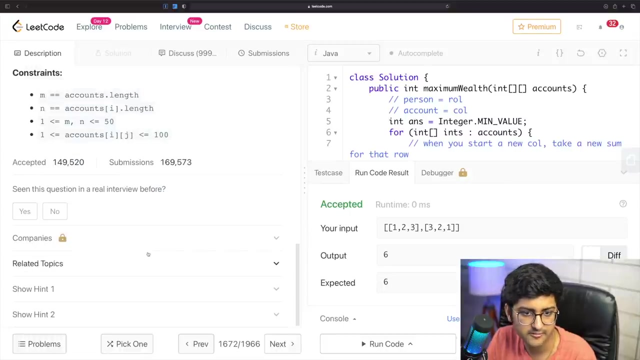 run. the code seems to be working, let's submit it. accept it. cool, that's basically about it. so you try to take the sum of every single one and then you, you, yeah, that's it. okay, let's look into the next question. all right, these were like some. 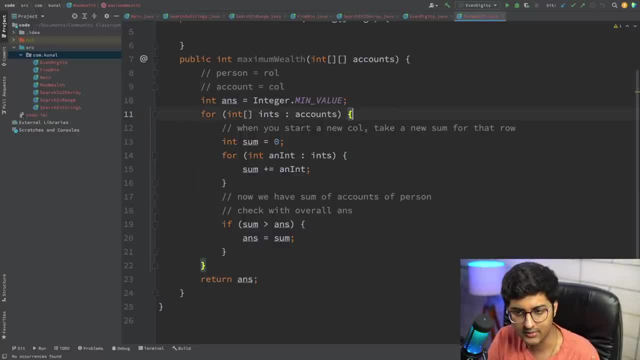 very basic questions. but, uh, i assure you, as the level of complexity grows of the algorithms- which you will definitely see in the next video itself, when we will be doing another searching algorithm known as binary search- so when we do binary search you will learn so many amazing algorithms and 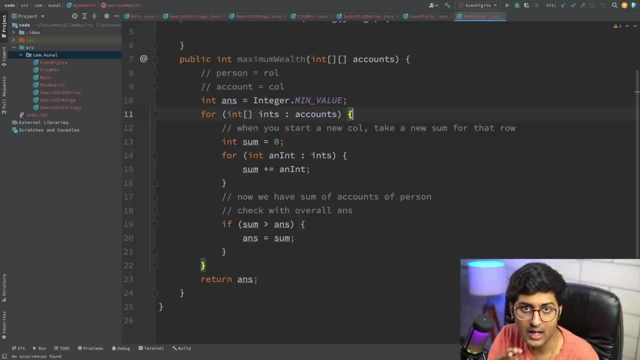 so many amazing things. we'll be doing some hard questions as well. it could hard and like google interview questions, for example, and that is pretty much about it, and uh, it's not like um, this is the topic that is over over here right now. no, these are like essentials, so we are going to be using linear search in many other complex 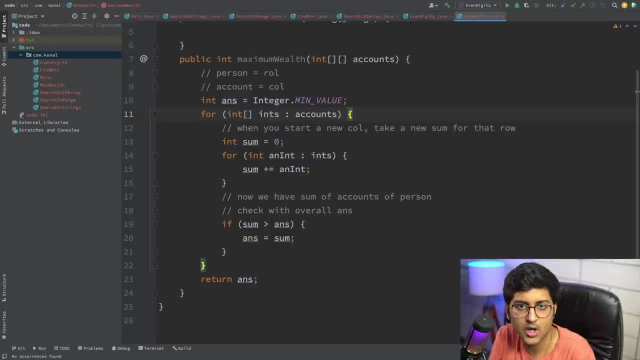 algorithms. so, for example, when we do recursion, so it's not like when the recursion topic is over, then recursion is over. no, it will be used at every single, like most of these concepts that will be working after that, so it's not like this topic is over yet. similarly, when we did drs before, 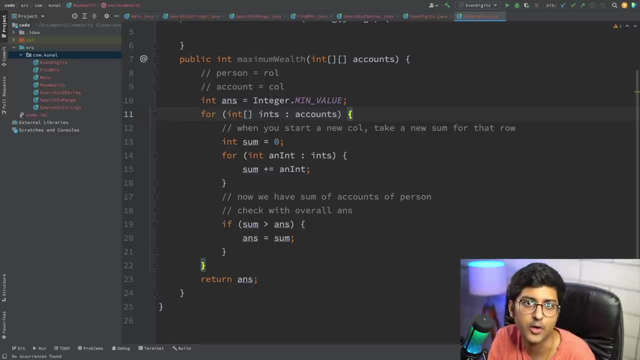 it's not like the topic of arrays is over. arrays will keep going on when we do heaps and stuff over there also, we'll be using arrays when we do some complex algorithms, when we're doing some like sliding window, two pointer stuff, when we're using hash maps and, like you know, heaps and stuff over.